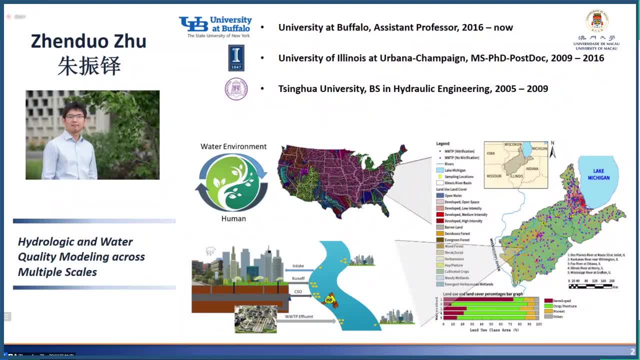 From 2009 Since 2016.. I'm assistant professor at university, at the buffalo, the state University of New York, So my research focus on hydrologic and water quality modeling, especially across multiple skills. So, as you can see here in our group, 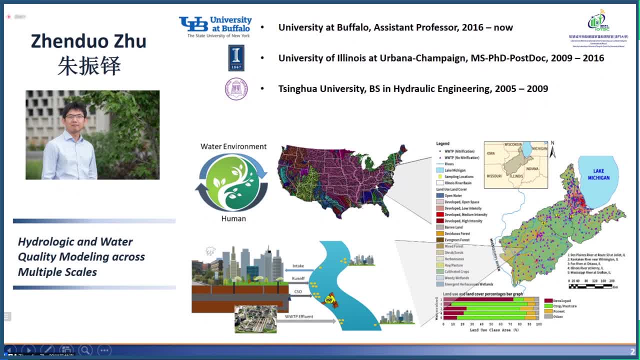 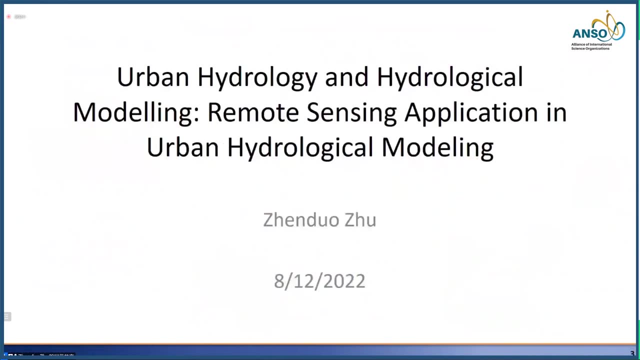 we work on, like you know, as large as a nation scale to a large watershed scale and also zoom into urban river or urban system scale. Okay, so this is my research background And this for the summer school. I want to share with you something. 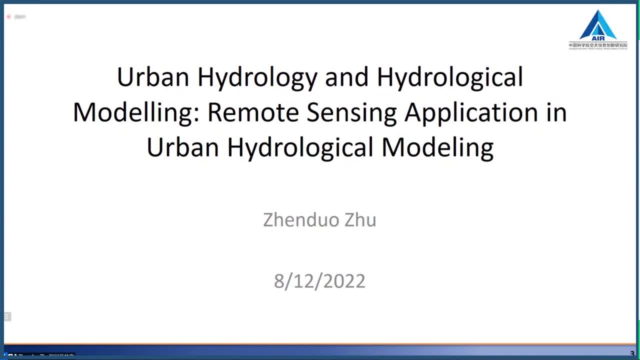 about urban hydrology and hydrologic modeling. So it is my understanding that for this summer school I want to provide basic content, So this is not like cutting edge research. I do want to share a little bit of cutting edge research during the presentation, but most of the time this is quite basic. So if 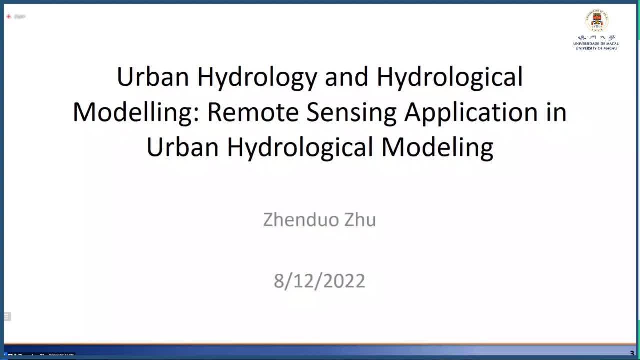 you have already taken classes in remote sensing or hydrology modeling. I apologize, you know you may not learn too much more from here, But hopefully some of the stories I want to share with you, hopefully they are- they are useful. Okay, So the 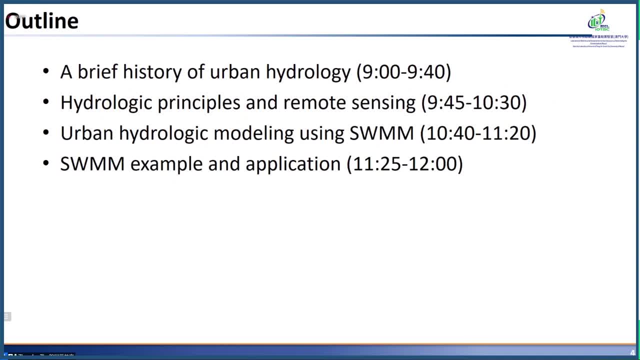 outline of today's class. I basically divided into four chapters or four parts. In the first part I want to introduce a brief history of urban hydrology. In part two, or chapter two, I want to talk about hydrologic principles and how remote sensing can help to understand. 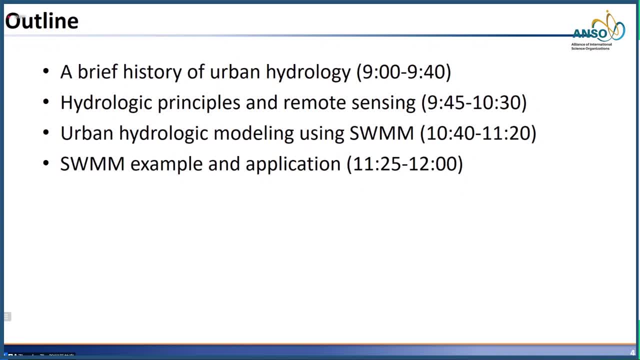 hydrology. Then in part three I will talk about urban hydrologic modeling using SWIM, And in part four we will see some SWIM example and application. Okay, as you can see, here between two parts there will be short breaks and a little long break, So just 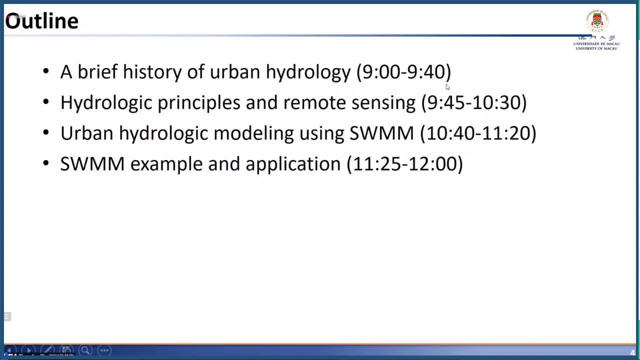 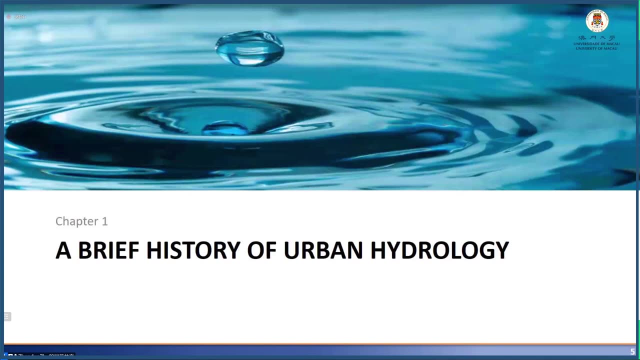 hopefully, if I can finish earlier than the schedule, maybe we will have more break or maybe I can have time for some questions. So yeah, just hope I will not be late. Okay, Let's get started with chapter one. Okay, a brief history of urban. 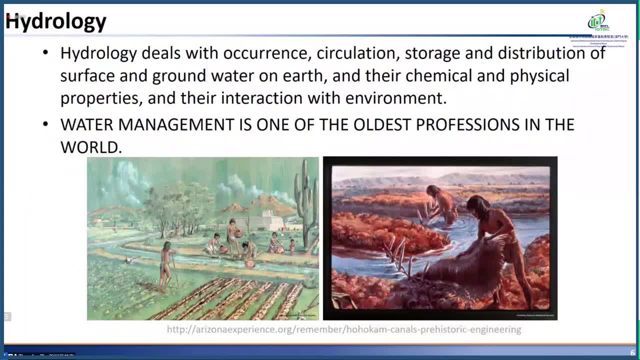 hydrology. So before urban hydrology, I think first, obviously, we should talk about hydrology, right? Hydrology- this word comes from ancient Greek, Hydro- means water, Largy means the study of, So basically, hydrology means the study of water. And, as you, 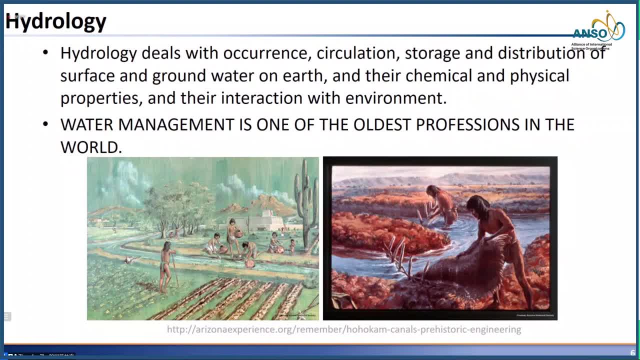 can imagine. like urban hydrology means the study of urban water, So hydrology deals with occurrence, circulation, storage and distribution of surface and groundwater on Earth and their chemical and physical properties and their interaction with the environment. Okay, So water management is really one of the 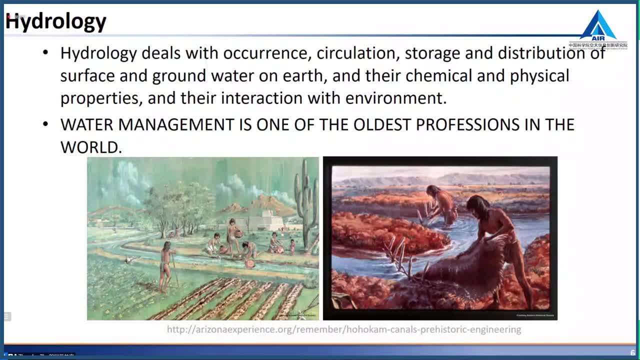 oldest professions in the world, if not the oldest, for sure one of the oldest professions, Because humans need water right. So water and food are essential to human beings. And in order to grow food or obtain food from animals, we also 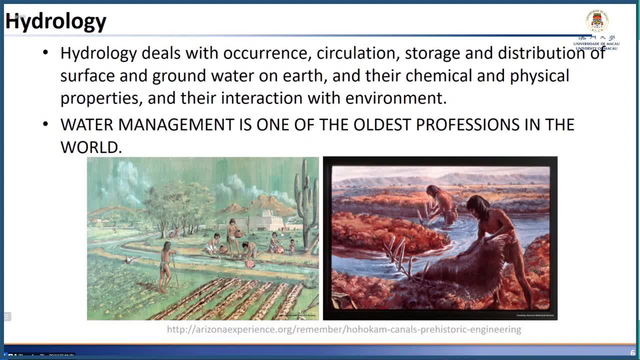 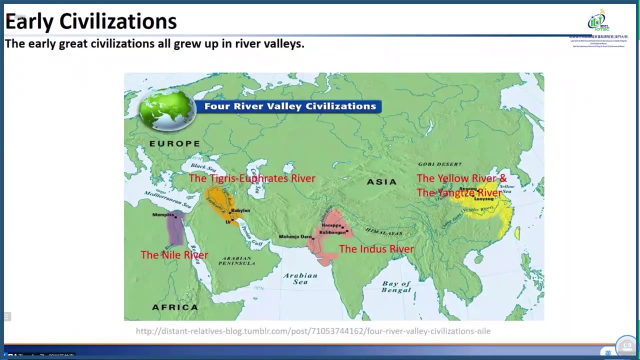 need water, right. So it makes totally sense that from the very beginning that people try to settle down close to rivers where you can get water supplies. So here are some examples If you look at the earliest civilizations. okay, so all of these early Greek civilizations grew up in river. 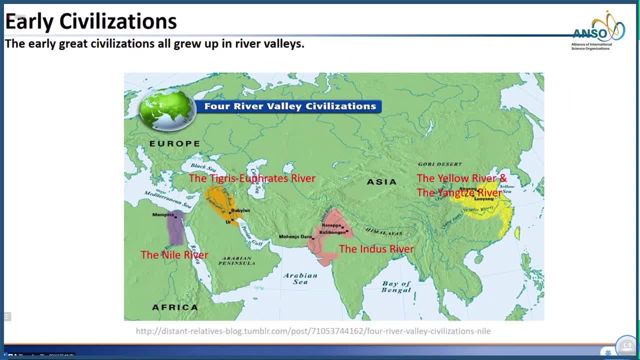 valleys. Okay, so those are the Yellow River, the Yangtze River civilization, the Indus River civilization, Tigris, Euphrates River and the Nile River civilizations. So I'd like to go through one by one, to introduce what humans were doing back then. 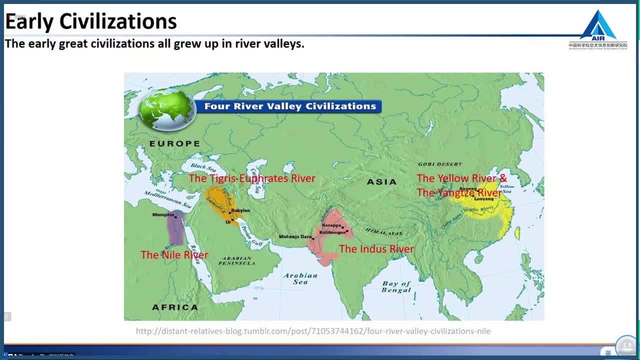 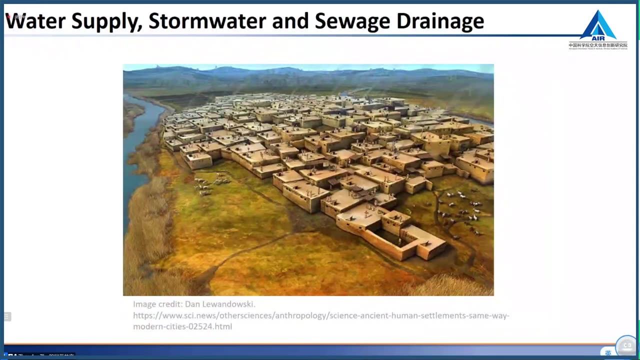 regarding urban hydrology: Okay, I'm not sure we can call it urban or not, But some of the concepts are pretty similar to what we call it like modern urban hydrology. Okay, So water supply, stormwater and sewage drainage- they are basically the. 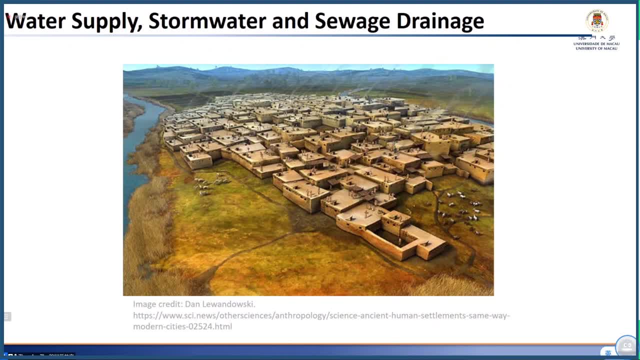 most important problems, especially water management problems, for human settlement Right. So, as you can imagine that when humans started to settle and live together, okay, So one of the most important thing to consider is where to get water and then where to dispose wastewater and where to 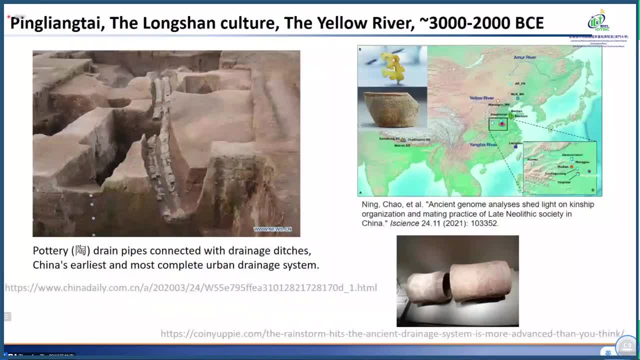 dispose sewage Right. So this is actually excavated very recently. If I remember correctly, this is early 2020.. So just before the pandemic, okay, in Henan province in China called Pingliangtai, which belongs to 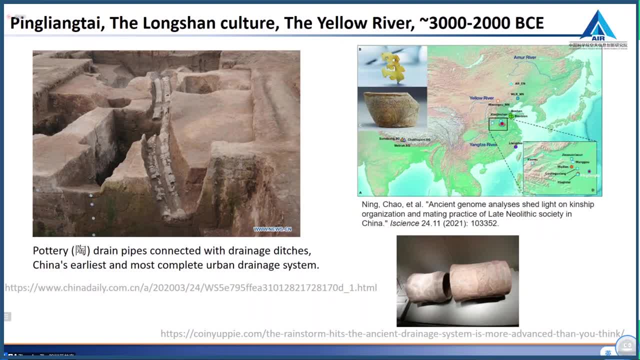 the Longshan culture. This is located in the lower Yellow River about 3000 to 2000 BCE, which is more than 4000 or 5000 years ago. So here from the excavations people find out that back then. 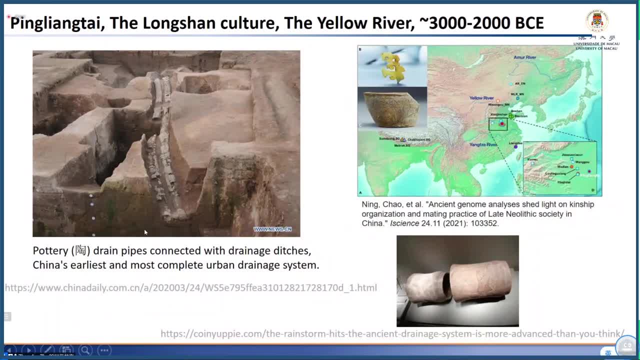 right. humans already started to use drainpipes, which are connected with drainage ditches, And the pipe is made of a pottery Tao, So this is believed to be China's earliest and most complete urban drainage system, and also one of the earliest. 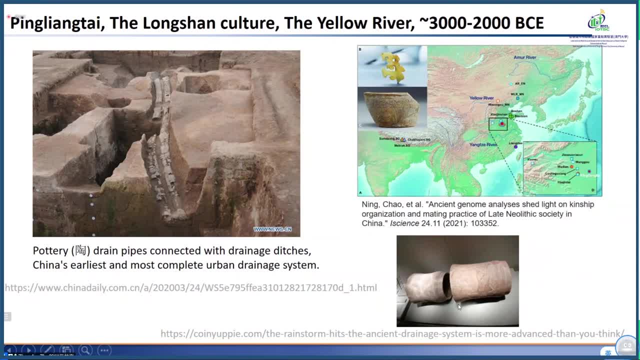 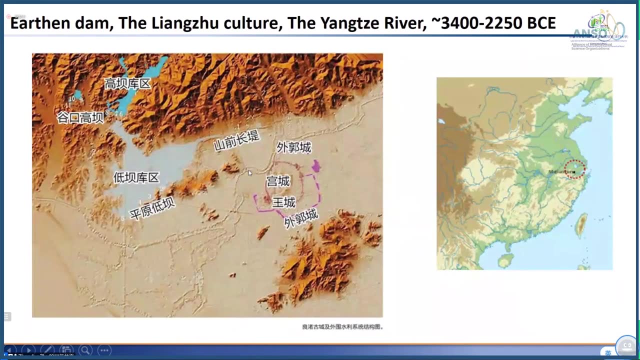 in the world. So here is covered complete pottery drainpipe But, as you can see, is mostly broken right now. So the other example of how humans use water, especially for settlement, is the Liangzhu culture which is located in the lower Yangtze River. 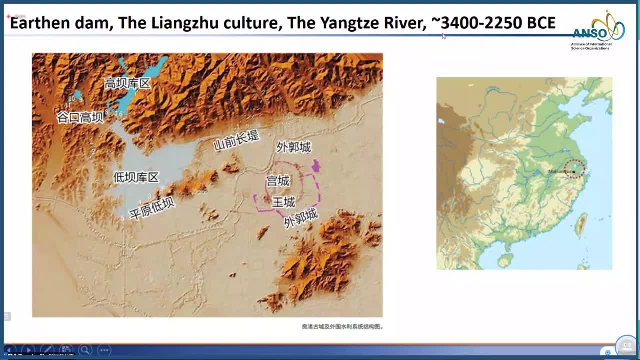 there in the lower Yangtze River, also about 3,000 to 2,000 BCE, the same, similar as the Longshan culture. So here in Liangzhu culture people have discovered there is a city. So of course not comparable in terms of you know. 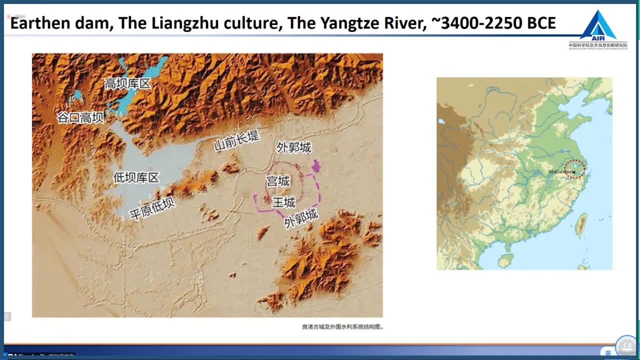 scale and size, population to like our cities now, but back then is pretty impressive, right, And more impressively, people started to build dams to first protect from flooding and also to get water supply into this city. okay, So just you know, think about that 4,000. 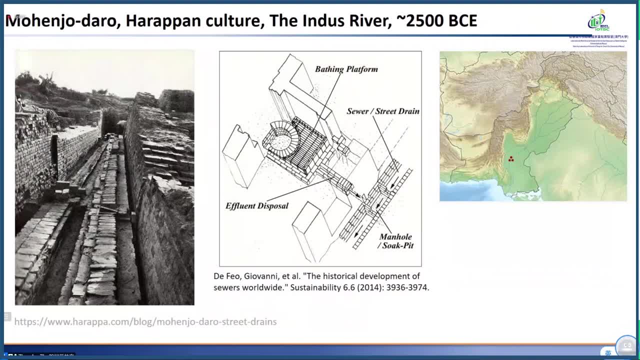 or 5,000 years ago. okay, So here is another example in the Indus River: civilization, Harapeng culture. So this is a city called Mohenjo-daro- I hope I pronounce it close, okay, So here, similarly, people have found that you know. 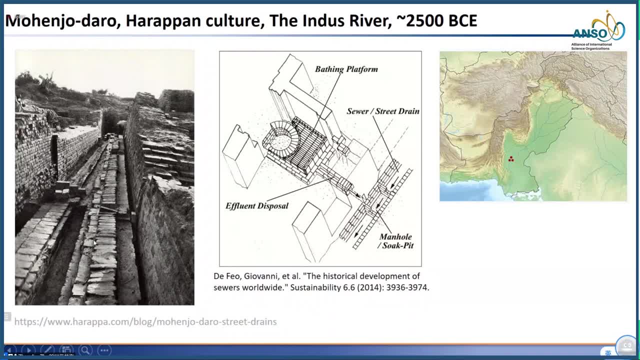 even at more than 4,000 years ago. so human started to know, like, how to drain, how to get water, how to get water, how to get water. So people started to know how to drain storm water, as well as waste water, from their settlement into rivers. 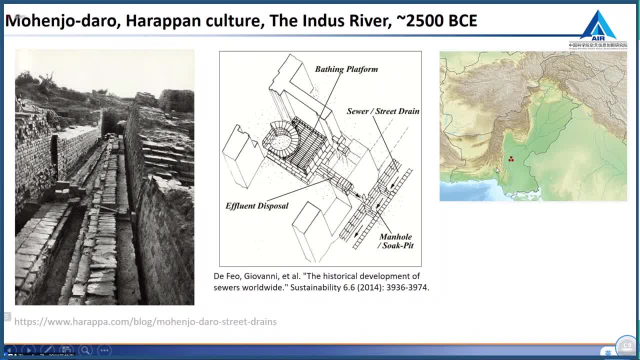 Okay, so in this case it would be the Indus River And also as you can see here. so back then people already started to have a bathing room and also knows how to drain the water from the bathing platform, So people started to know how to drain the water. 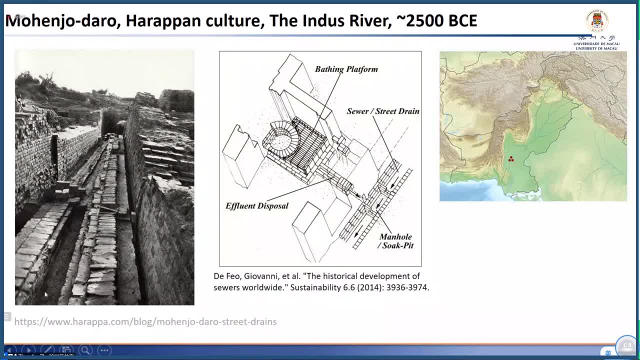 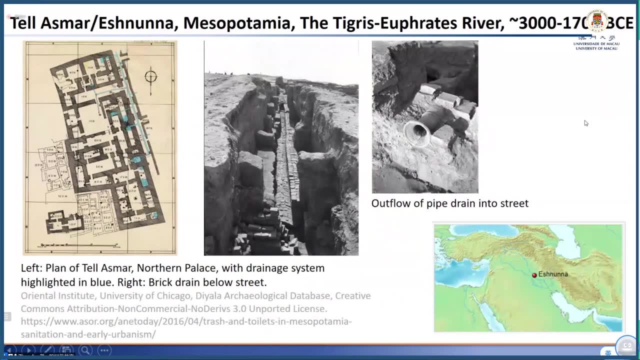 from the bathing platform into a surface channel right And then finally goes to the river nearby. okay, So here again we are looking at about 3,000 to 2,000 BCE located in the Tigris-Euphrates River. 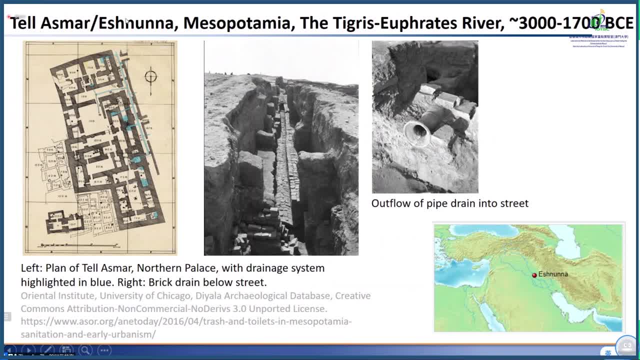 So what a city called Keoathmer, or also called as Ashu Ashunana- again, sorry if I pronounce it wrong. okay, So this belongs to the Mesopotamian culture And here, as you can see, in this northern palace, 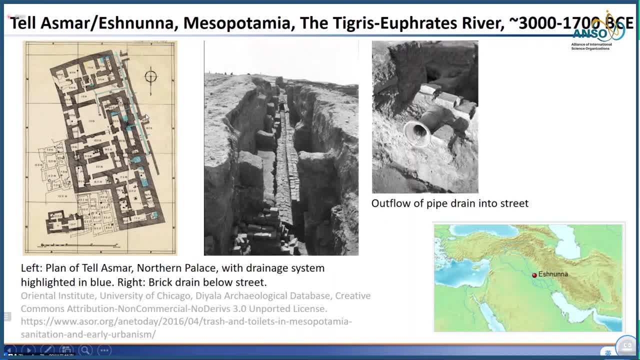 there has been drainage system, highlighted in blue in this figure. okay, This is how it looks like now. So, as you can see, there is drainage channel that is lower than the street, which is covered by bricks, And also people found the waterfall pipe. 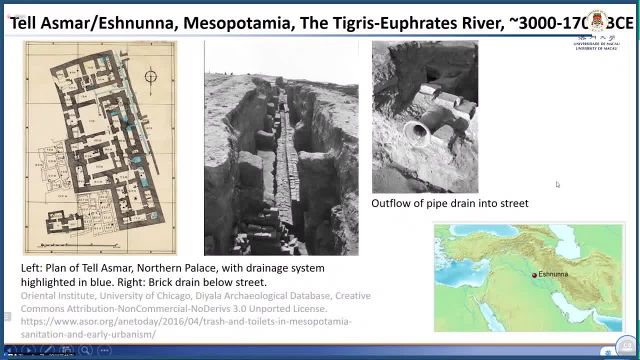 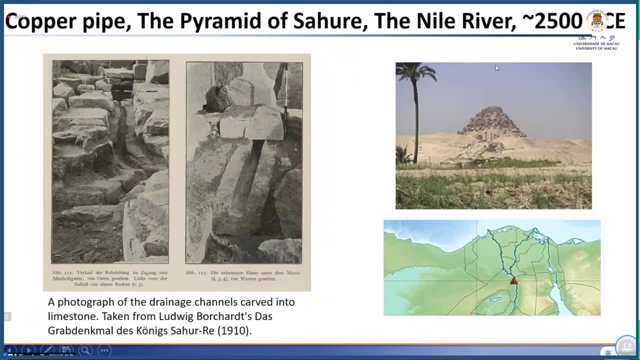 which drained into the street. So if we look at the last one, the Neo-River civilization here in the pyramid of Sahur, again back to more than 4,000 years ago, so people started to use copper pipe instead of pottery or clay. 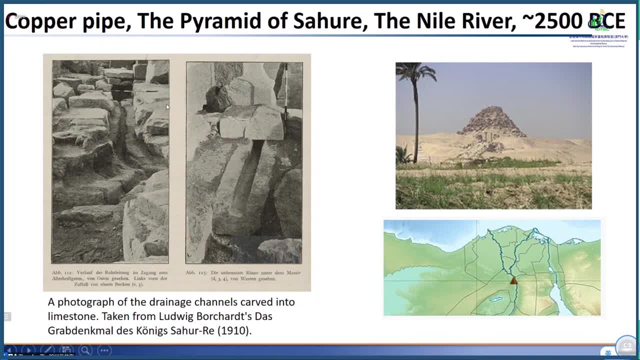 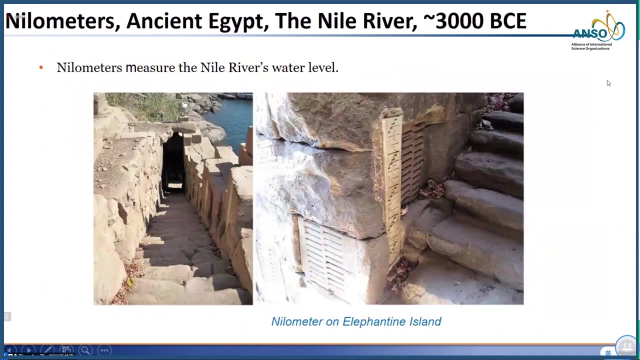 So obviously this is a more advanced material And back then they cannot use it to sew out the whole drainage system, but only a couple of hundred meters. However, I think it's already very impressive. So also I want to point out this is not urban drainage. 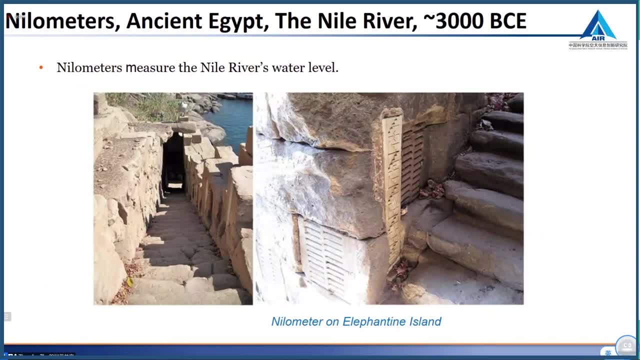 or water supply, but a very impressive invention which is called nanometers. Right, Right, Right. This is in ancient Egypt, at the Neo-River. More than 5,000 years ago, people started to measure the water level of the Neo-River. 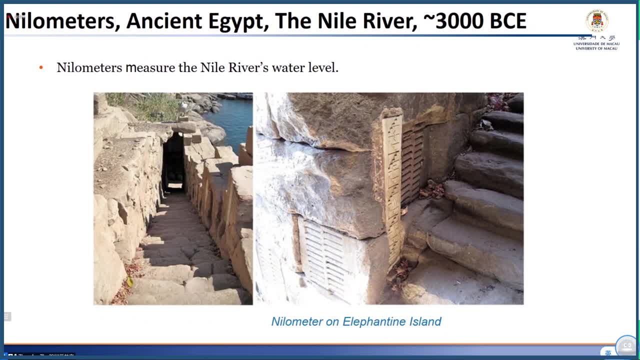 Because the agriculture in ancient Egypt heavily depends on the flooding of Neo-River, which delivers nutrients to the soil, to the land. So if you know the water level, you can actually predict, you know, the agricultural production for the coming season. 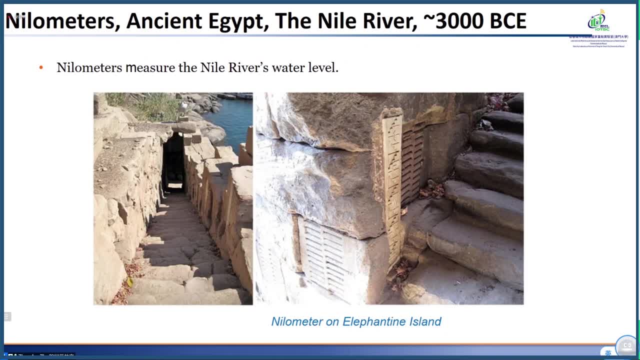 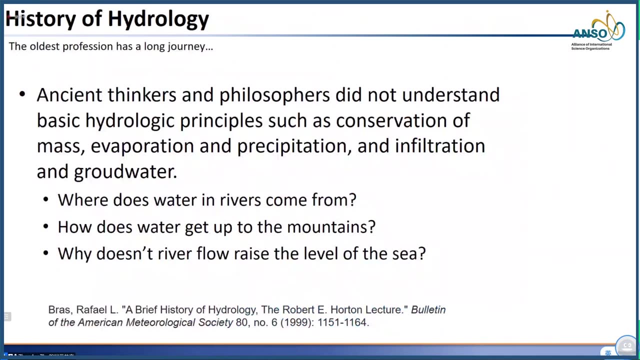 So just think unbelievable that how, like 5,000 years ago, you know, people started to collect those knowledge. OK. So, given what we have said about the impressive projects or you know, drainage systems or materials, OK. however, in terms of hydrology, 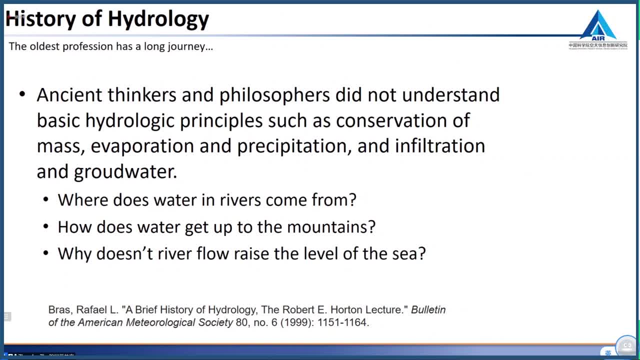 from a scientific perspective, this oldest profession actually took a long journey to reach our modern understanding about hydrology. OK, So I would just ask you to imagine if there is is a time machine that you can actually travel back to 4,000 or 5,000 years ago. right? 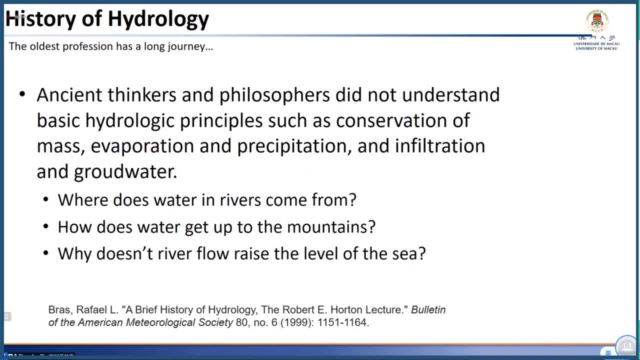 Even with the knowledge you have, OK, how are you going to convince human back then what hydrology should be right? So for example, like what hydrologic cycle should be? Where does water in rivers come from? How does water get up to the mountains? 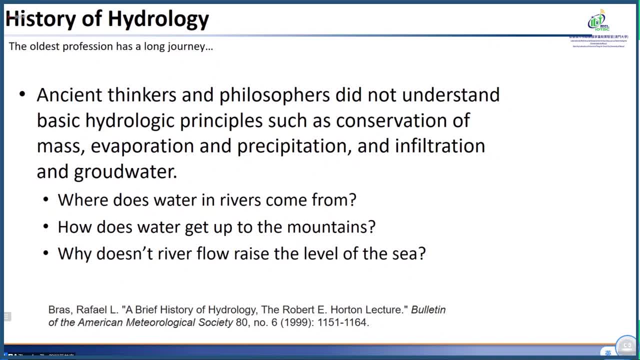 Why doesn't a river flow reach the level of the sea? So those may seem very simple questions for now, but back then, you know, those are very, very challenging. So the ancient philosophers actually did not quite understand the basic hydrologic principles. 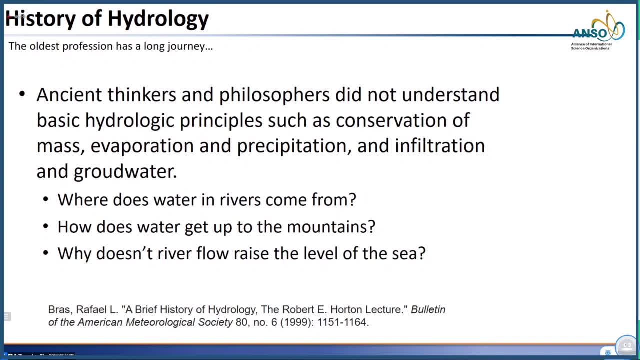 such as conservation of mass evaporation and precipitation, especially infiltration and groundwater. OK, Those are very, very challenging for ancient thinkers and philosophers. So if you go back to ancient Greece, if you can sit down with Aristotle and ask Aristotle those questions, 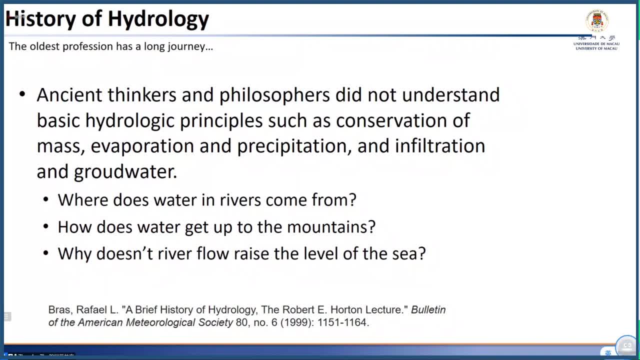 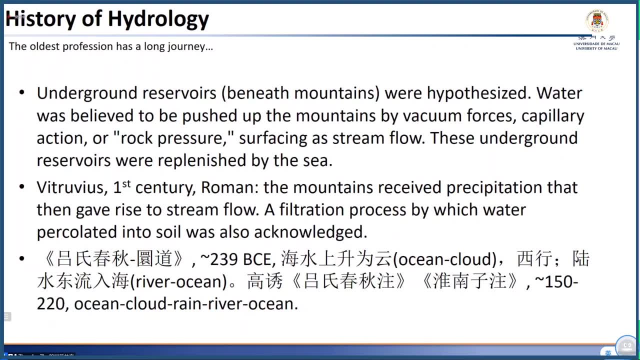 he probably wouldn't be able to give you an answer, or at least not the correct answer. So because of that, there are hypotheses. you know, people have human, people have proposed OK, So one very interesting hypothesis which actually was pretty widely accepted, at least in ancient Greece. 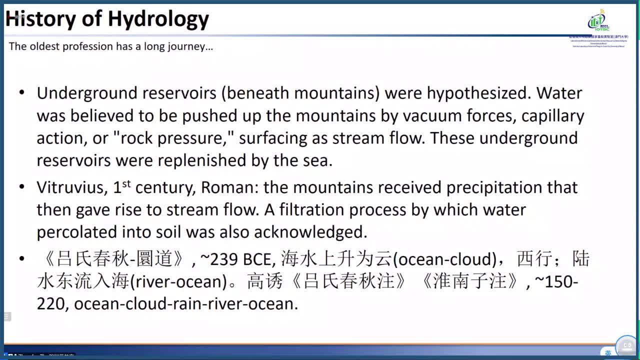 is the underground reservoir hypothesis? OK, So they believe that water is pushed up to the mountains? So they believe that water is pushed up to the mountains by some kind of source. OK, Some kind of force, maybe vacuum force or capillary action. 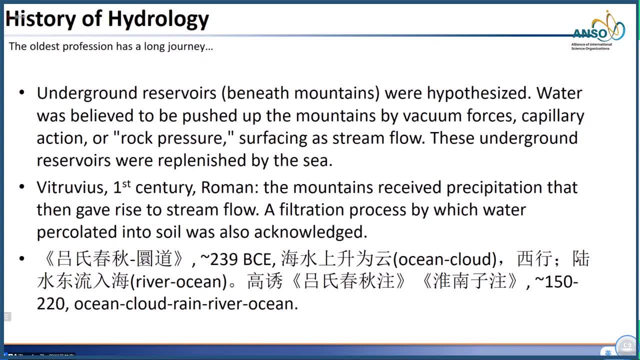 or rock pressure whatever, But those water are actually pushed up to the mountains from underground reservoirs, And these underground reservoirs were replenished by the ocean. OK, So I think it sounds very interesting for us now, But again, like these hypotheses was widely accepted, 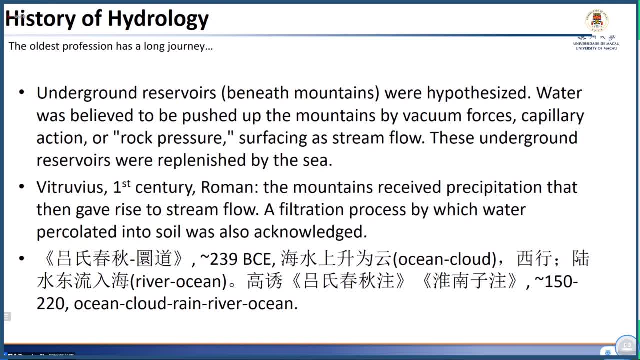 for a very, very long time. Then, in the first century, Vitruvius, a Roman. so he actually wrote down that the mountains received precipitation. So the mountains, there was a very large amount of precipitation that you know gave rise to stream flow. OK, 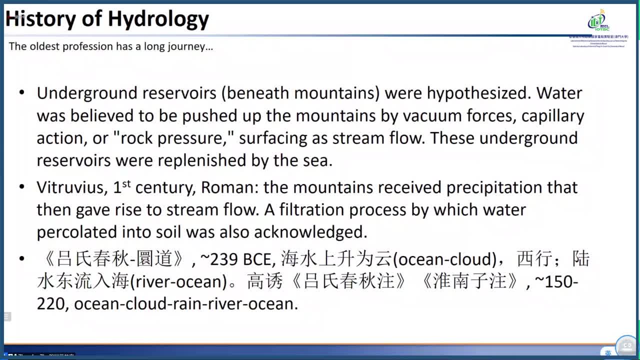 So this has been a big step forward, right? So at least he answered the question where does water come from in river, correctly, OK, So his answer is: the mountains receive precipitation and then the precipitation actually cause stream flow. OK, Also, at the same time he acknowledged: you know, 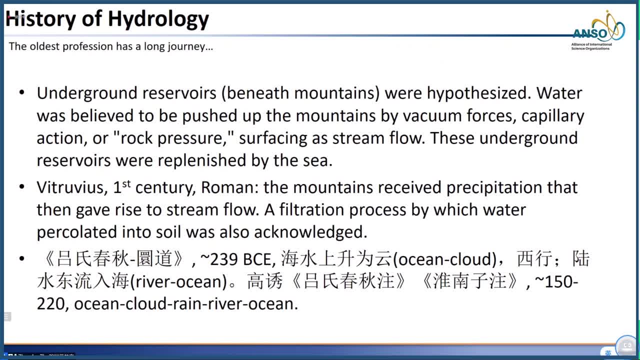 filtration process. So he noted that water can percolate into soil and he called it filtration. OK, So at about a similar time in China, basically circle. So that is about 239 BCE, So it was recorded, OK. 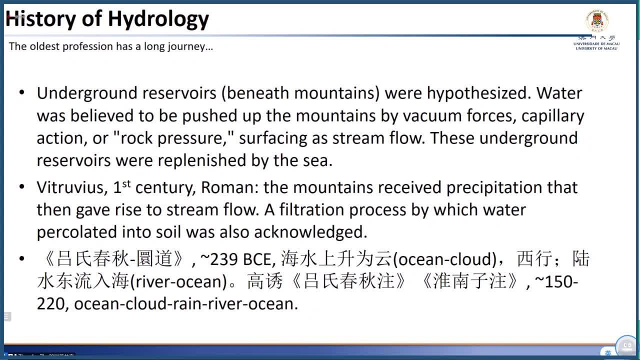 He recorded that, meaning that you know water in the ocean can become cloud right And then you know the cloud will move to the west. That is because if you know the geography of, you know China, so China, actually, you know the ocean. 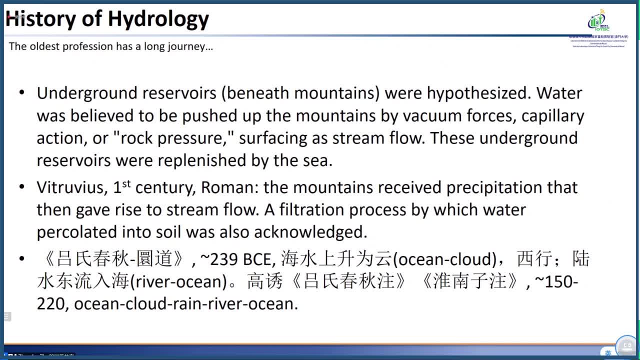 is located on the east side of China, right. So that's why he said the cloud will go. once formed on top of the ocean, it will go west, OK, And then the rivers will flow east into the ocean, OK. So later in about Han Dynasty. 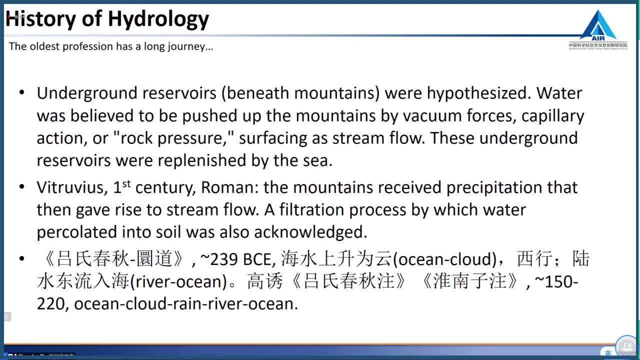 in, and which is about 150 to 250- BCE 220.. So he has explicitly noted a circle that goes from ocean to cloud, then to rainfall, then the rainfall goes to the river and then river goes back to the ocean. At the same time, he also 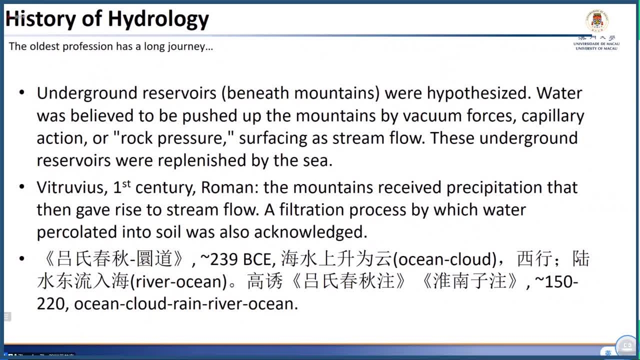 noted some circle about groundwater, But again the infiltration concept is not clear, at least not recorded explicitly or clearly back then. So basically now if we do a very quick summary, if you think about from 5000-4000 years ago, 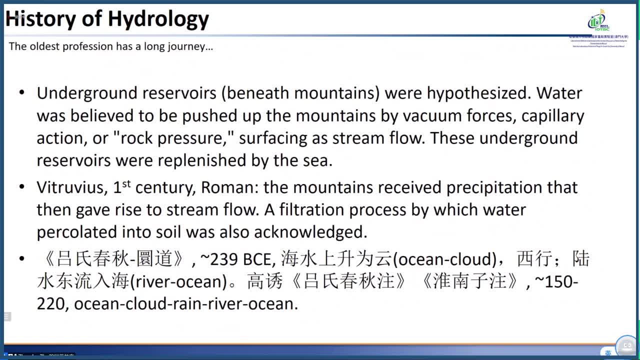 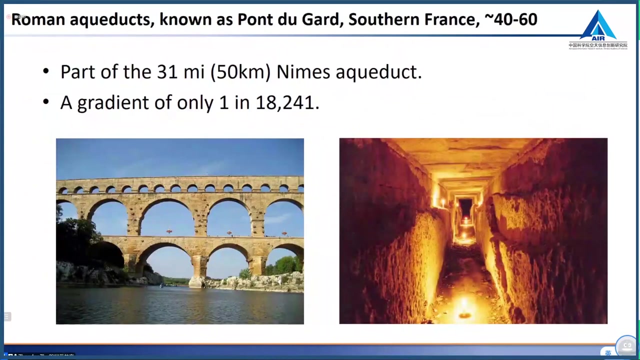 until about 2000 years ago. it took about two to 3000 years for humans To kind of get the hydrologic cycle correctly. Okay. so still it's not very complete, It's not quantitatively proved, But at least you know we get this most of the circle correctly Okay. 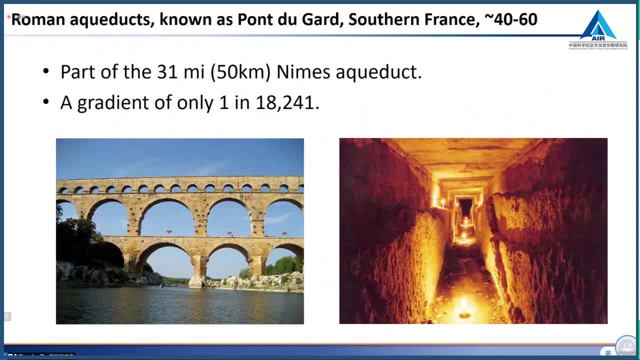 So, but at the same time, hydrologic engineering has been advanced a lot, right? I'm only showing you one example, which is the Roma aqueducts. So this is at in the first century. So here in the picture we are showing part of a 50 kilometer. 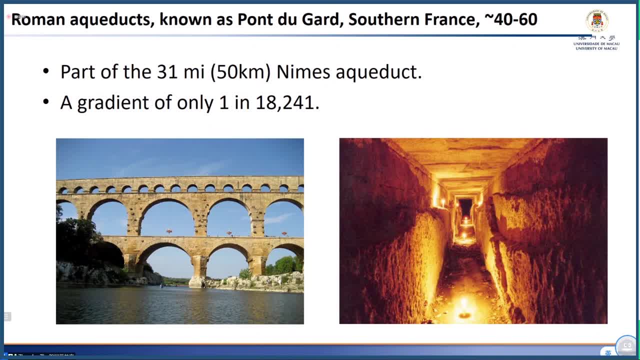 aqueduct. And what is more impressive is the gradient of this aqueduct is only one in more than 18,000.. So which means back then people must have mastered the technology of measuring elevation very well. So this is kind of a very brief. 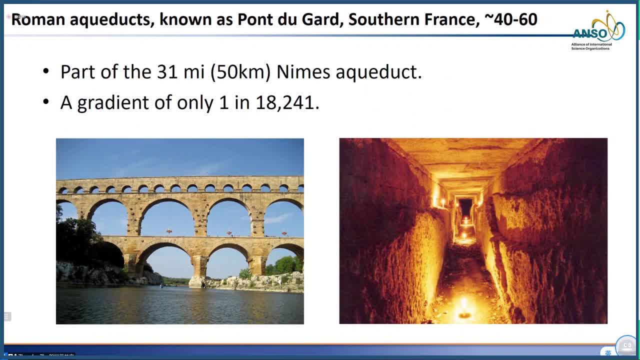 history from 3000 BCE until like the first century. Okay, Then, unfortunately, from first century until you know, 16th or 17th century is not much things like too exciting. Okay, Well, I shouldn't. I should take it back. So there are a lot of engineering. 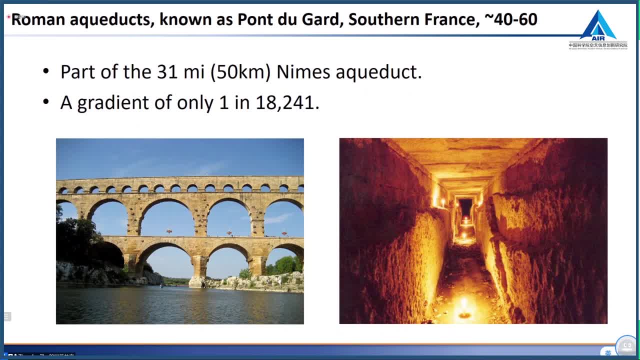 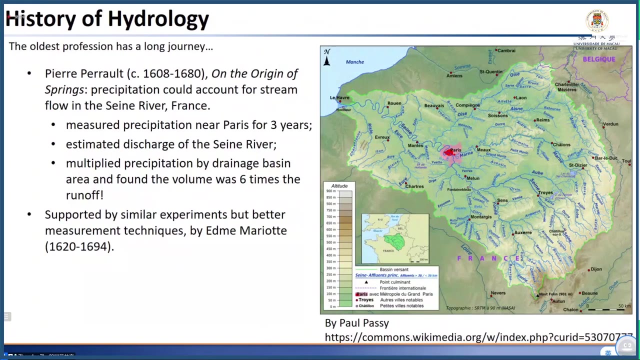 practices which are very, very impressive. For example, in China we have Du Jiang Yan Right, which still functions now, But in terms of hydrology, in a scientific perspective, it didn't go very far. So interestingly it. 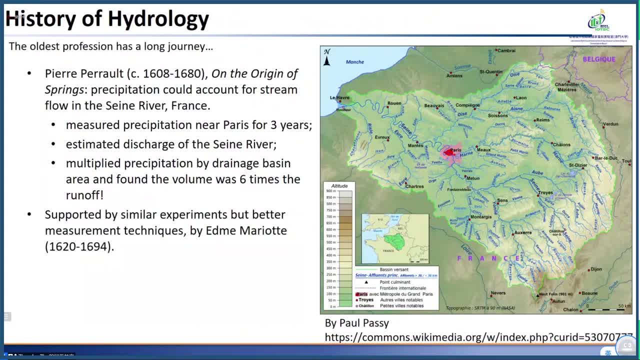 is until the 17th century, in 1600s, that people started to make measurement and try to prove the hypothesis which had been proposed a long time ago. Okay, So one of the first measurements was done by Pieri Perrot, So he documented his measurement in this book called On: 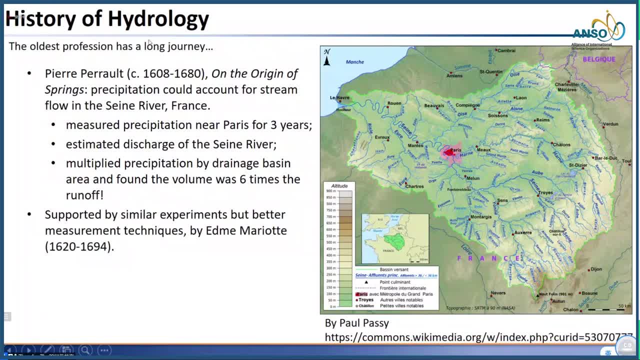 the Origin of Springs And he basically tried to prove that precipitation could account for streamflow in the Seine River in France. Okay, So what he did? he measured precipitation near Paris for about three years. He estimated discharge of the Seine River. 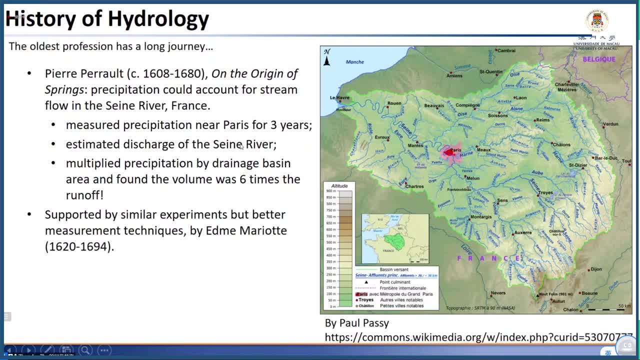 Oh, by the way, one I think important reason why, from the first century until 1600s, there were not too much advancement in terms of the Seine's. I think one important reason is because the measurement technique Okay, So you need a very good. 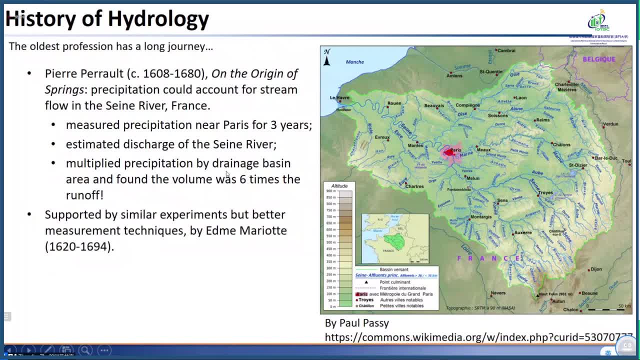 measurement technique in order to do this kind of study. Right, And that later I will talk about. you know the remote sensing technology, So obviously you know that wasn't there back then. Okay, so then, after measuring precipitation and measuring flow, discharge. so he 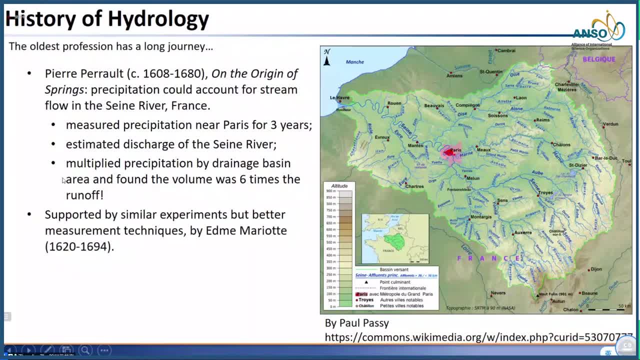 multiplied precipitation by the drainage basin area and found that the volume of the precipitation was actually six times the flow discharge. Okay, So, at least quantitatively, you know. this is the first proof that precipitation is large enough. right, the amount of precipitation or the volume of 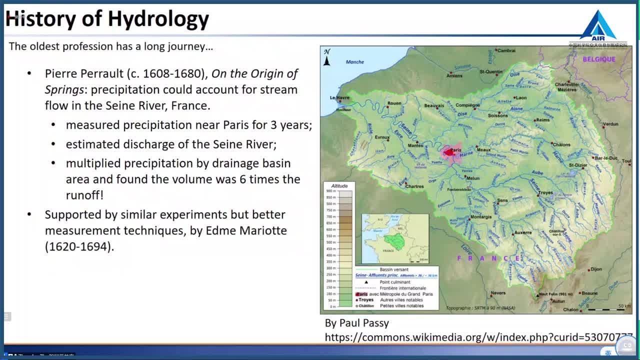 precipitation is large enough to account for streamflow. So later, this same conclusion was supported by similar experiments, but with better measurement techniques. For example, one of that is Mary Arch. So I'd like to point out that those are very, you know, pioneering scientific research. However, due to the 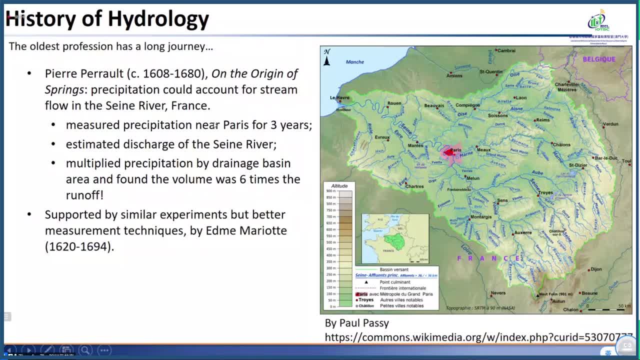 limitation of the measurement and also the limitation of a lot of other knowledge, right? so, as you can see here, this is not a very complete water balance analysis, So it is simply precipitation versus streamflow, right? So he did not discuss about infiltration or you know other. 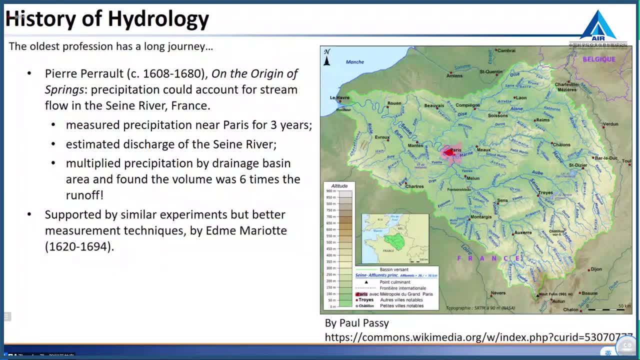 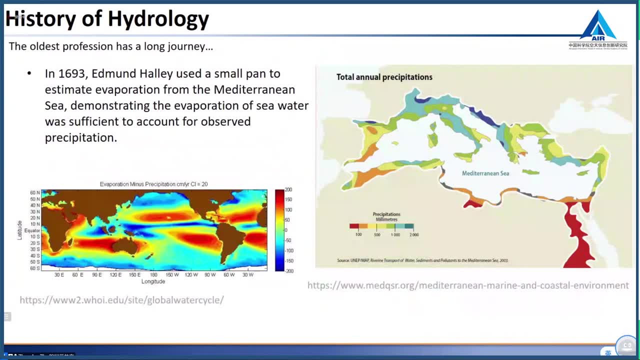 processes in the hydrologic cycle or in the water balance, in the whole entire water balance. So later, by the end of 1600s, Edmund Harley used a small pan to estimate evaporation from the Mediterranean Sea. Then, from his study, he 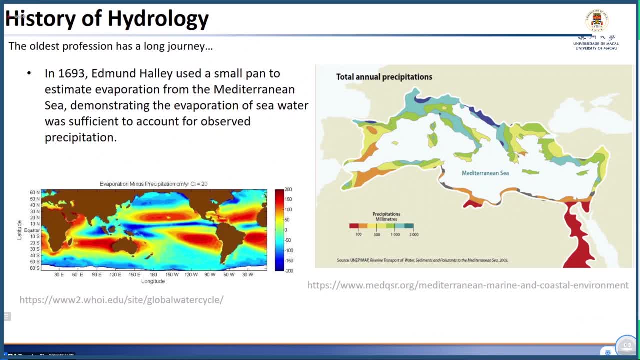 demonstrated that the evaporation of seawater, basically the Mediterranean Sea water, was sufficient to account for observed precipitation in the Mediterranean Sea basin. So, as you can see here, this is the map for the Mediterranean Sea. So Mediterranean Sea is almost a closed. 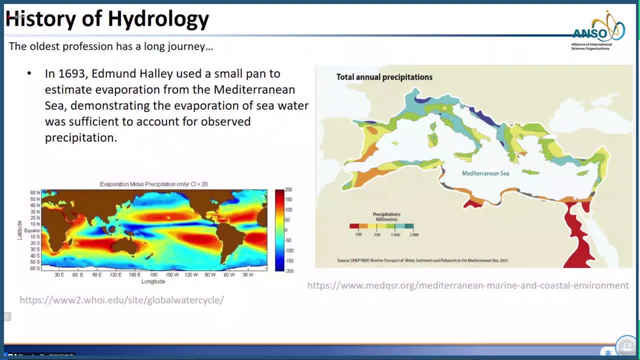 ocean or water body, right. So in his study again it's very pioneer and you know, I think it should get a lot of acknowledgement. But from a modern perspective now this is again. water balance isn't really accurate, right? Because as we know now, 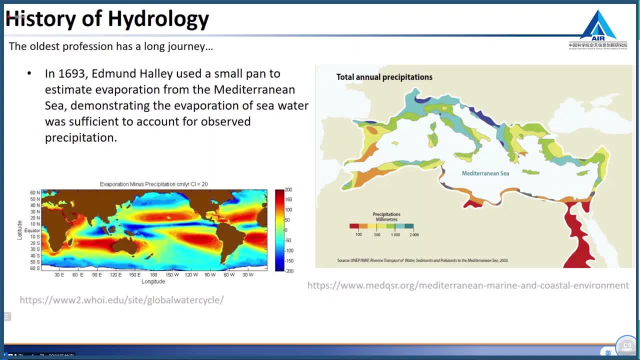 evaporation actually is a global scale process, right? So you cannot just look at one watershed or one basin, Even though Mediterranean Sea basin is quite big, but it is not accurate to only compare the evaporation of a Mediterranean Sea, Even though Mediterranean Sea basin is quite big, but it is not accurate to only compare the evaporation of Mediterranean Sea. 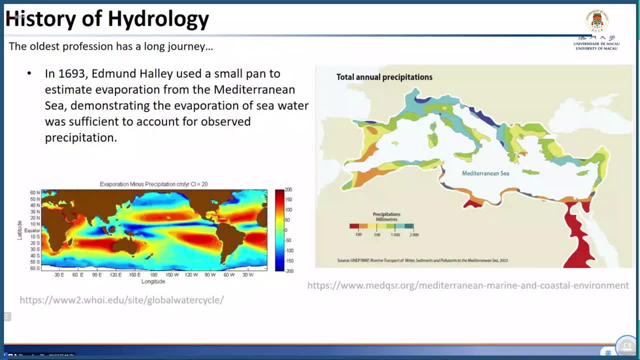 Mediterranean Sea versus the precipitation on the Mediterranean Sea Basin, right, So this is precipitation, and evaporation should be a global scale process. So, as you can see here, right, But of course back then you know there is just no way to do that. 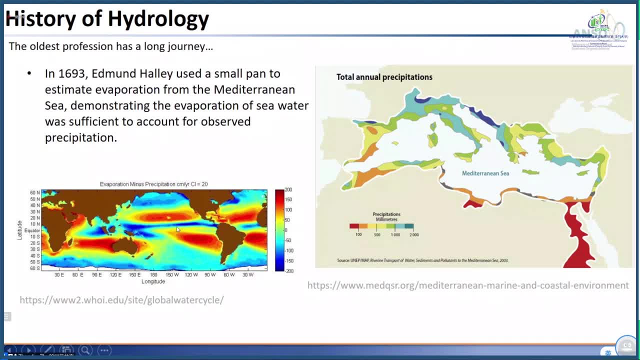 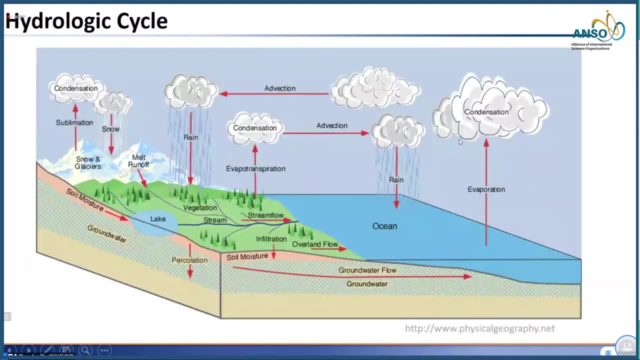 And nowadays we can do it largely thanks to remote sensing technology. So after thousands of years now we have a complete understanding of hydrologic cycle. So water in the ocean or lakes, basically surface water, can evaporate. then you know, by condensation it became the cloud. 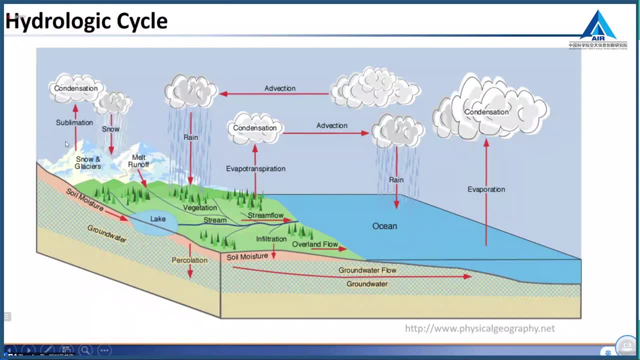 And by global circulation. this can bring precipitation on the land or snow, right It could be rainfall, either rainfall or snow, And then the precipitation generate runoff. runoff forms rivers and streams, then finally stream goes back Back to the ocean. 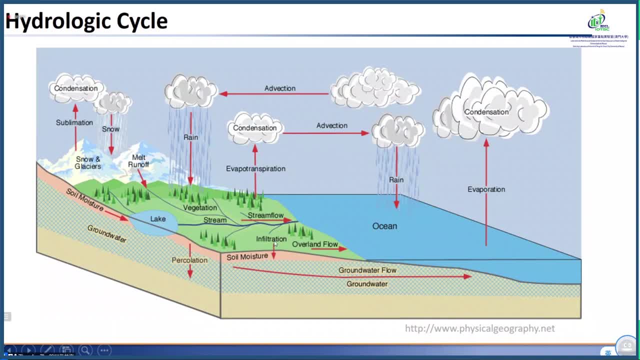 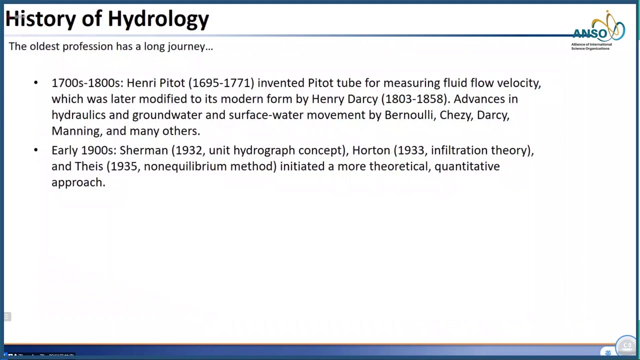 Also. at the same time, precipitation can infiltrate to the soil and became groundwater, And groundwater also from a global scale. it flows into the ocean right. So this is our current understanding of hydrologic cycle. So later, Sorry, Sorry. 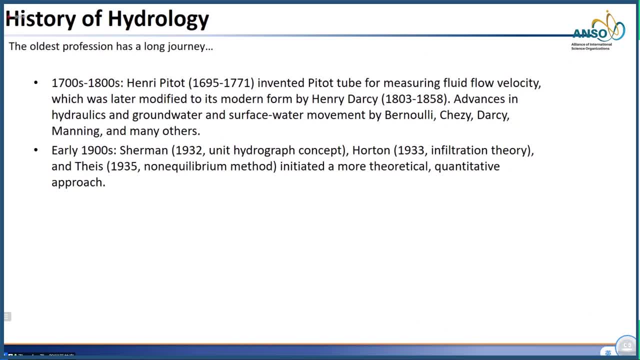 I'm sorry. So when we are talking about the 1700 and 1800. There are, you know, significant advancement. For example, Henry Pitot invented the Pitot tube for measuring fluid flow velocity, which is still widely used nowadays. 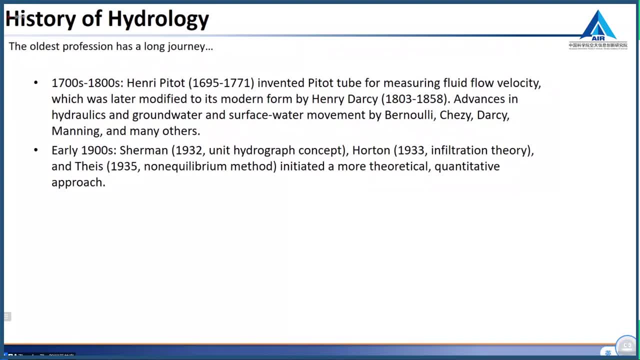 It was later modified to the modern form by Henry Ducey And there are also advances, Significantly significant advances, in hydraulics and groundwater. so both groundwater and surface water, by Bernoulli, Chezy, Darcy, Manning and many others. I believe if you have started hydrology, 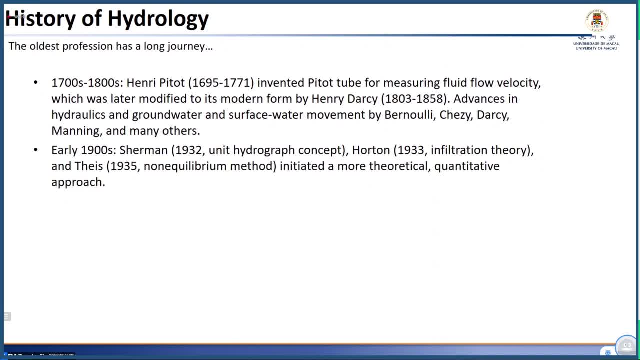 or hydraulics. those names are all very familiar. However, it is until the early 1900s when the modern hydrology started to evolve. These start with Sherman in 1932, who proposed the unit hydrograph theory or unit hydrograph concept. Then, at a similar time, Houghton. 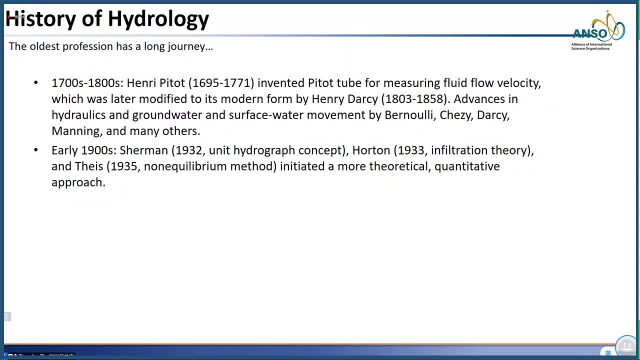 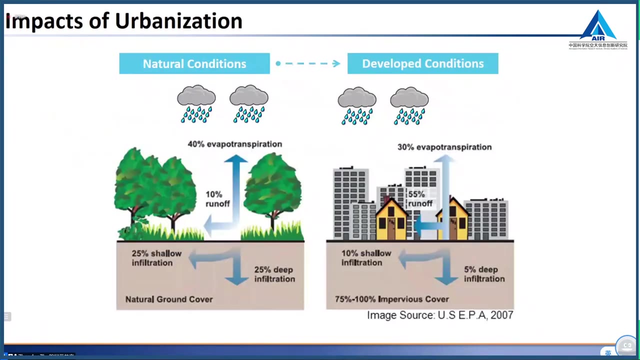 introduced an infiltration formula and Thiers, in 1935, introduced a non-extraordinary equilibrium method. Then all of this in the early 1900s initiated a more theoretical and quantitative approach to study hydrology. So through the same time, if you look at it globally, it's a global. 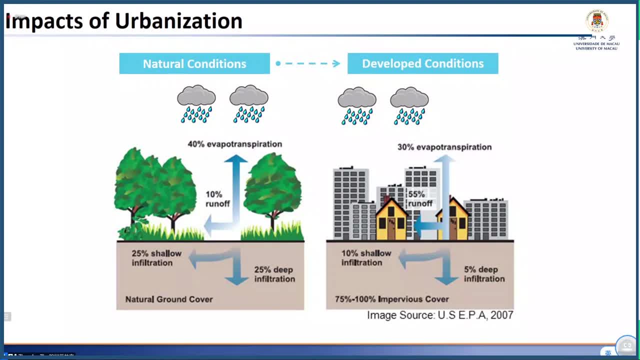 plan shipping and all thesehmassings And then. thank you, Io. if you are interested into learning more about Hydrographs, please share. this link will be on the top of the slide, But it's nice to see the affairs of order. 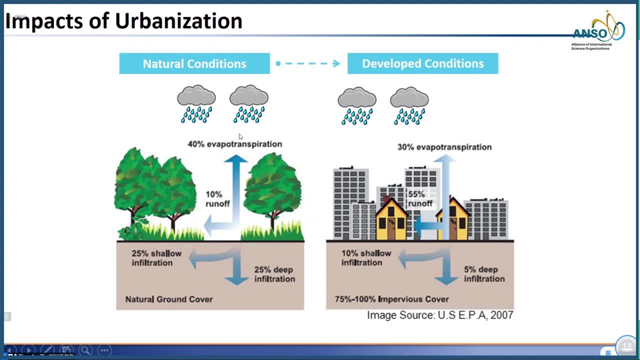 hahahahahah бел. 40% of the precipitation will evaporate or transfer it And 50% or half of the precipitation will infiltrate. Then there is only about 10% runoff generated, However, under the same rainfall amount. 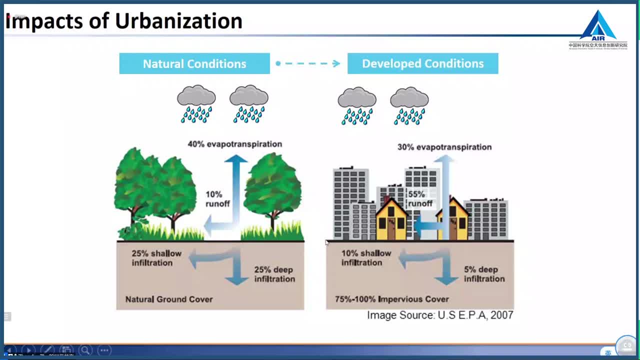 if you look at a developed condition, because of the land it becomes much more impervious in a developed condition than the natural condition, So there will be much less infiltration. So instead of 50% it's only 15% of infiltration. 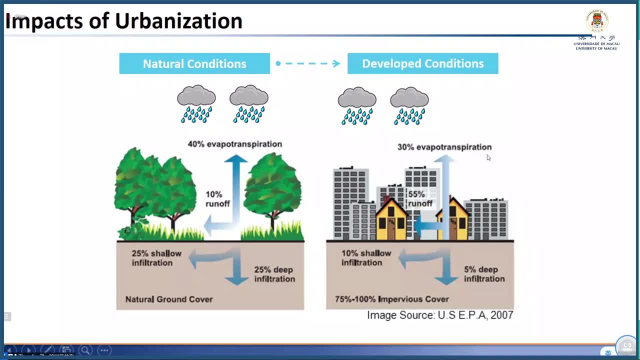 And also evaporation or transpiration becomes slightly less or 10% less, Then in the end there will be more runoff. So So 55% of the precipitation can become runoff, compared to only 10%. So that's a problem in the urban environment. 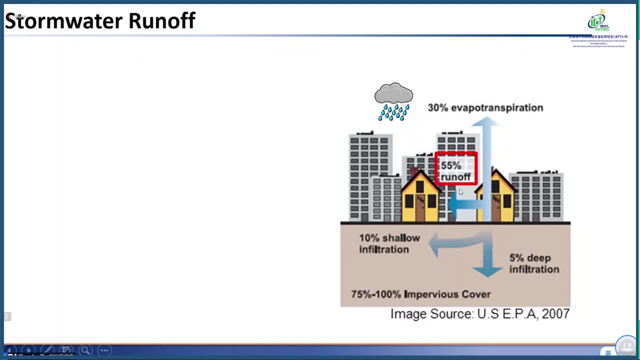 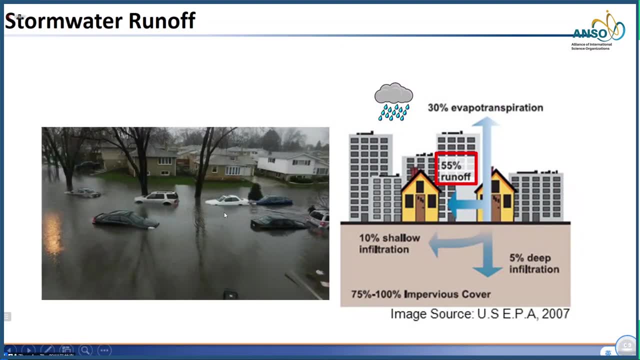 So this stormwater runoff, this 55% or five times more runoff, is going to generate problems like this, So like street flooding, basement flooding, And it is still happening right now. So this is from the quantity perspective. So how to deal with that? 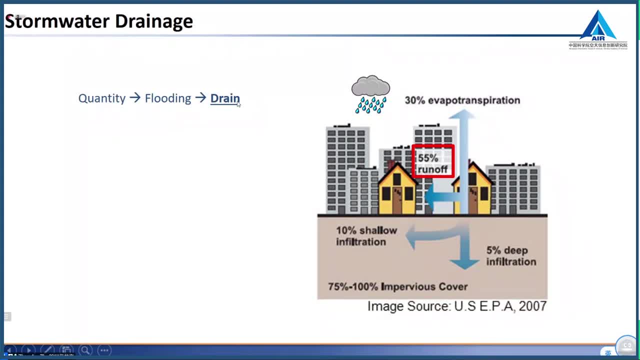 Again, we have to drain stormwater to somewhere. So this is the same concept as humans did back to 4,500 years. So when it rains, we need to drain stormwater somewhere, So we started to build a drainage system. So obviously we have better technology. 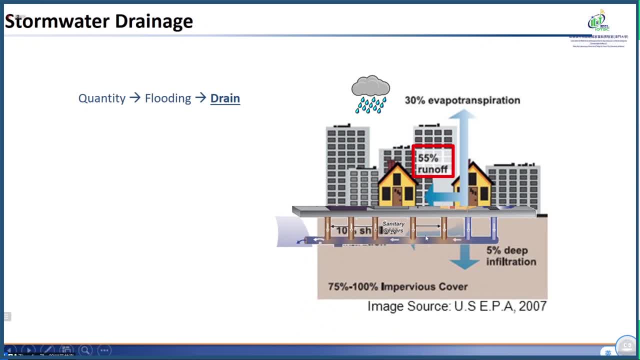 than 4,000, 5,000 years ago. So we can build underground drainage pipe network that will drain the stormwater runoff as well as as well as the sanitary from the urban environment go to surface water such as rivers and lakes. 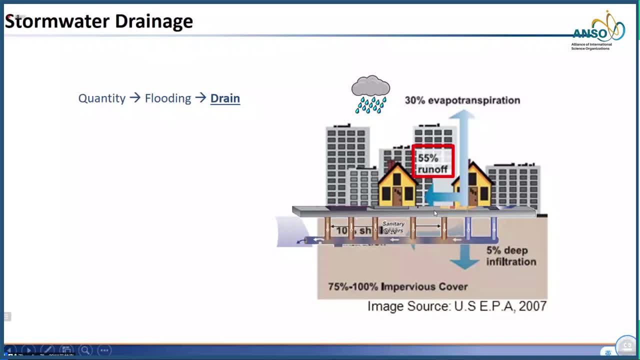 And the idea was to drain it as soon as possible, So then we will not have flooding issue. So for a very long time the focus was on how to engineer solutions to move rainwater rapidly away from urban areas to avoid damages. OK, 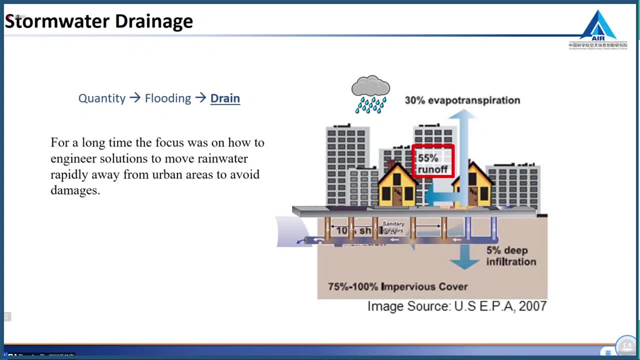 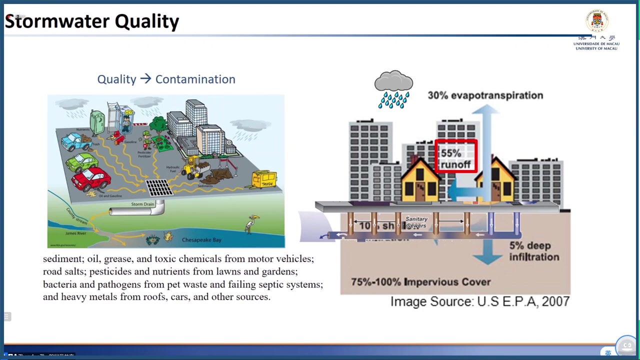 However, now there has been new philosophy developing that treat rainwater more valuable as a resource instead of as a hazard or disaster that needs to be moved away. So that's the quantity part of stormwater runoff. The stormwater runoff does not only cause quantity problem, such as flooding. 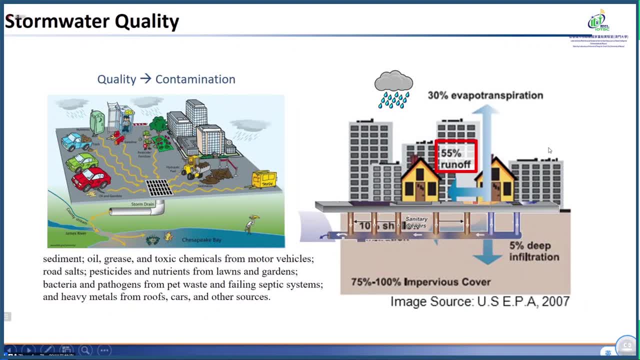 but also quality problems. As you can imagine, there are all different kinds of contaminants or pollutants that are built up on the parking lot, the street or in maybe also soil Right, And then when it rains, so those contaminants are going to be carried out by the stormwater runoff. 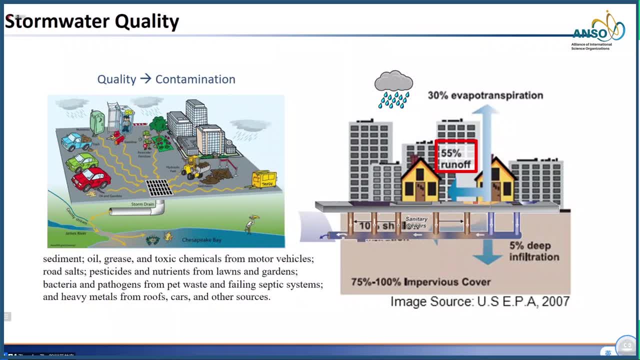 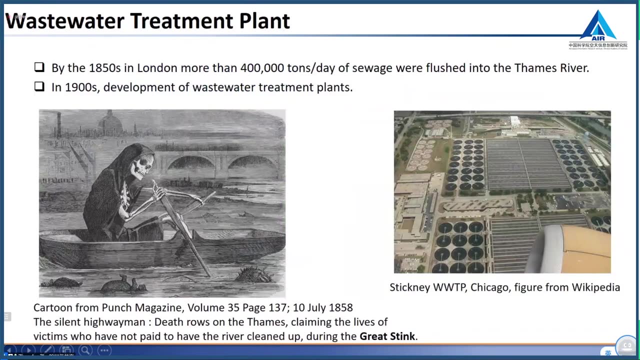 And finally, if you drain it directly to surface water, it's going to pollute surface water. So there are all kinds of pollutants there, as you can imagine. So by the 1850s, just as an example, maybe one of the famous examples in London. 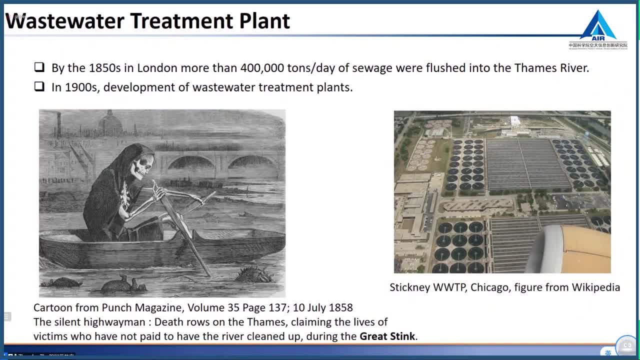 OK, More than 400,000 tons per day of sewage were flashed into the Thames River. So here on the left there is a cartoon published in 1858, which is describing what is now called the Great Stink. It's because in that summer there, 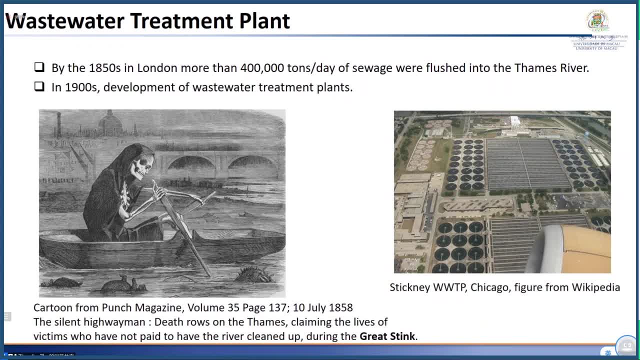 is a great stink of waste in the Thames River and which became a public issue, got a lot of public attention and finally people started to think about solutions or different approaches. So one of the most important approaches is actually the development of wastewater treatment. 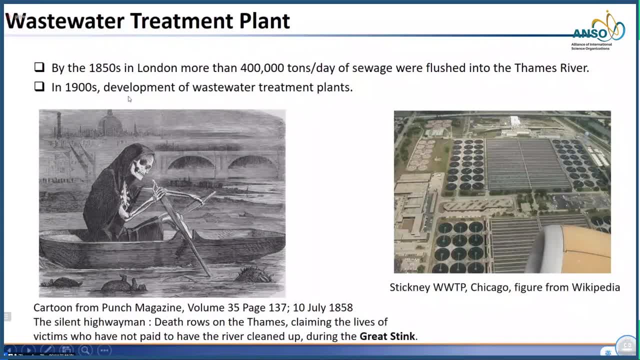 plants. So that is from the end of 1800s to 1900s. So there have been wastewater treatment plants developed. So here is one example of the largest wastewater treatment plant in Chicago. Again, this is taken from an aircraft actually, again remote sensing. 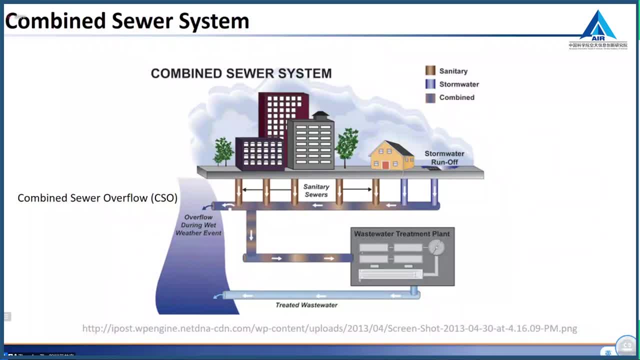 So, with the development of wastewater treatment After treatment plant, then what happened is, instead of drain stormwater and sanitary directly into surface water, now we first drain it to wastewater treatment plant And then, after treatment, the treated wastewater then will be discharged back to surface water. 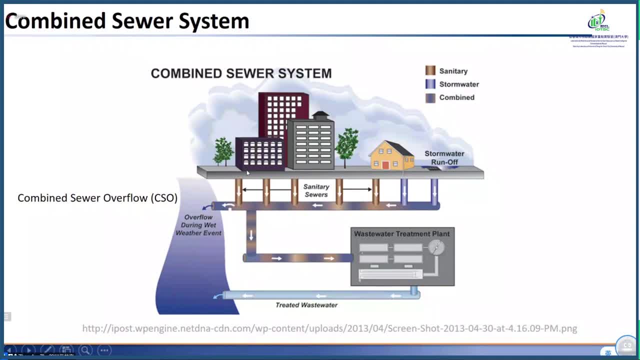 So obviously the treated wastewater is much better than the untreated wastewater. So yeah, So at the time there are two approaches people considered. One is this here called the combined sewer system. Basically, the stormwater ran off and the sanitary sewer goes to the same pipe. 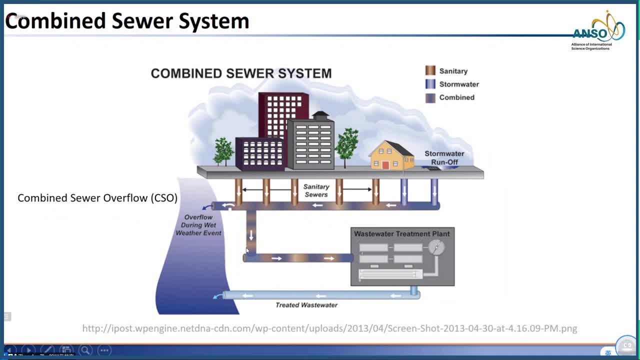 Right, And then this pipe from what is called interceptor goes into a wastewater treatment plant and then the treated wastewater goes back to Right, to surface water. There is an obvious drawback of this design. That is because under dry weather, everything is fine. Well, if the system works perfectly, everything is fine. 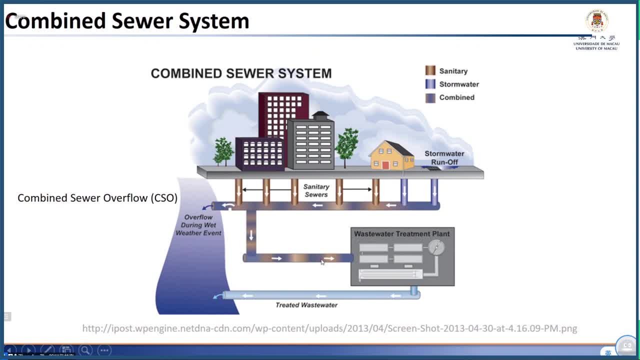 The sanitary sewer can be discharged into wastewater treatment plants and then got treated. However, when it rains, the combined storm water and the sanitary the flow can easily exceed the capacity of this combined sewer system. In order to prevent basement flood or street flood, we still have to let the overflow during wet weather event go into. 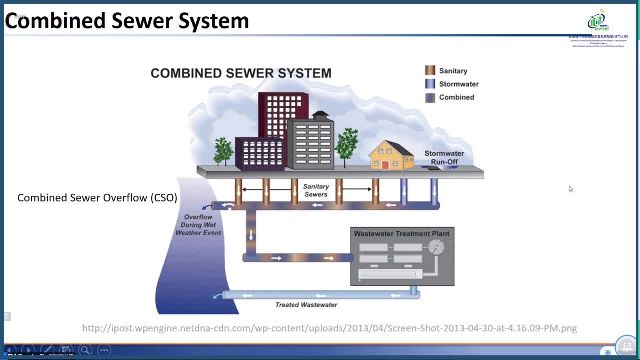 surface water. Again, this is not the only solution or approach people considered Even by the end of 1800 or early 1900, people actually discussed whether we should make it a combined sewer or we should separate them. So we should have two separate sewer systems, one for storm water only and the other for sanitary only. 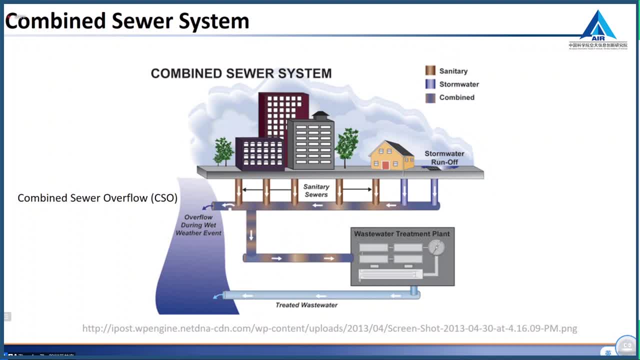 So people actually discussed these two approaches And back then many cities, their managers, after discussion, decided to follow a combined sewer system approach Because first it is cheaper And second people believed that this overflow- so basically what we call combined sewer overflow now- would not cause a significant 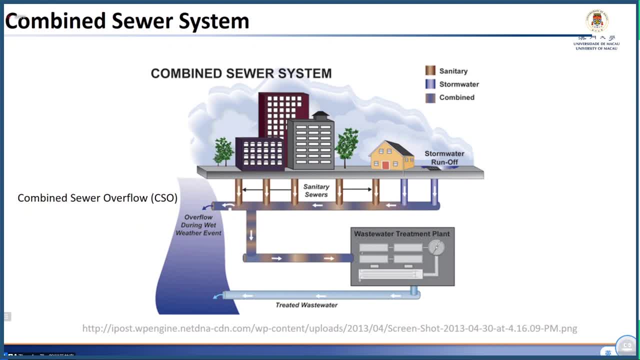 environmental problem. People believed so. Of course, now it is proved to be wrong, But it is always interesting to look back into the history and see how people made decisions based on a different understanding of the values of the environment and also the ecosystem. So, as I have introduced then the other 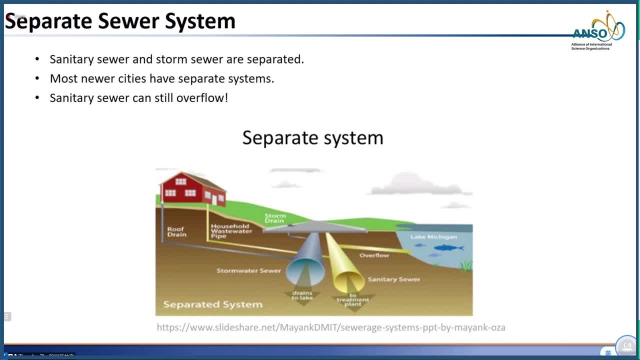 approach would be the separate sewer system approach. So basically two separate sewer systems, one for storm water and one for sanitary, And most of the newer cities have adopted the separate systems after realizing the development problems caused by combined sewer overflows. However, it doesn't mean separate sewer system doesn't mean in particular sewer system, doesn't mean the whole wave. 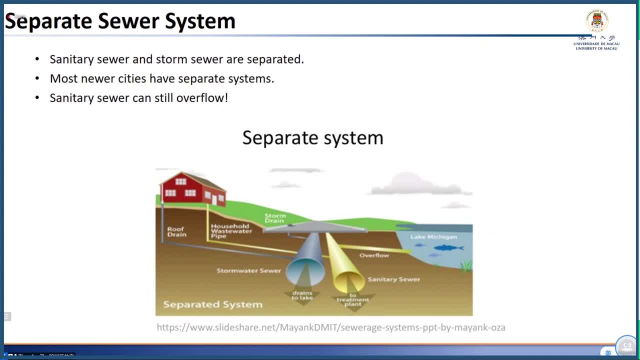 have an environmental problem. So often sanitary sewer can still overflow And in many cities, as I'm aware of, you know, there are construction problems which basically, you know, displace the sanitary sewer and storm sewer wrong. So there are still a lot of issues with separate sewer system. But 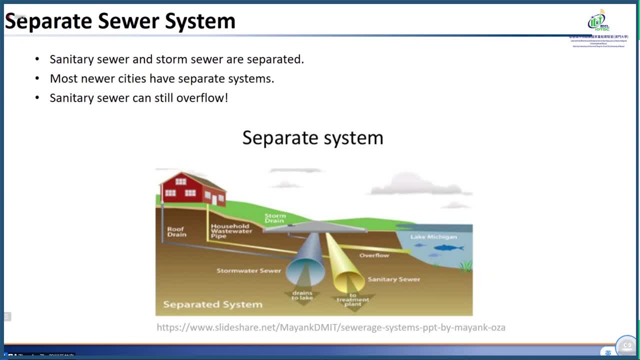 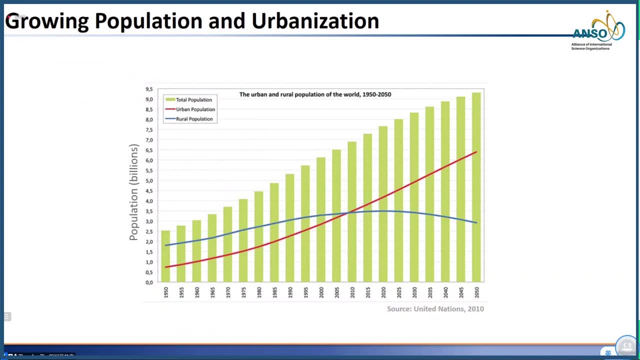 overall, it is better than the combined sewer system. So then, if you look at this number of population since 1950, right. so globally, we are facing a growing population problem and growing urbanization problem. So, by 2008, the urban population and the rural population on the 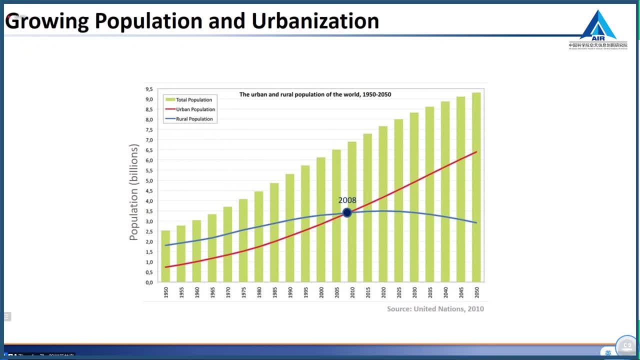 earth reached the same And after 2008,. urban population has continued to increase, while the rural population has reached the maximum and started to decrease Right And by the United Nations it is estimated or predicted that by 2050, more. 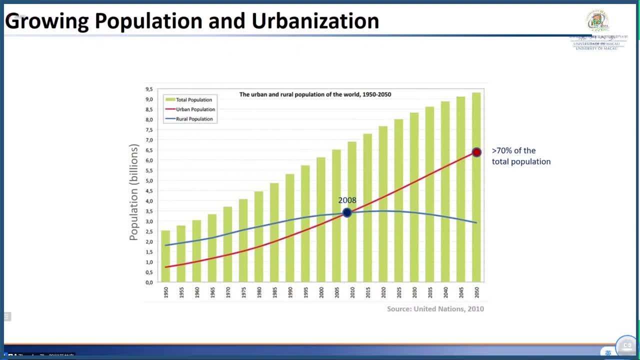 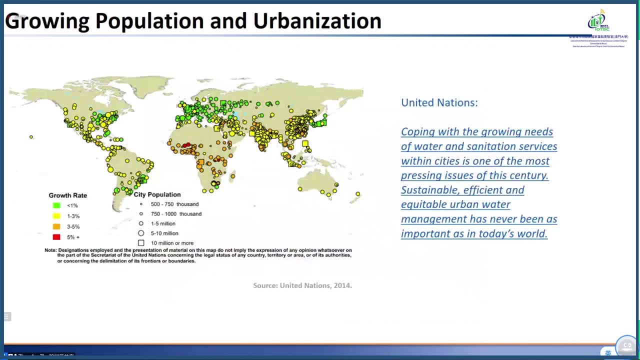 than 70% of the total population will live in urban environment rather than rural environment, And here is a report from United Nations 2014.. As you can see here, the size of the circles represent the city population and the color represent the growth rate. So, except Europe, Northeast United. 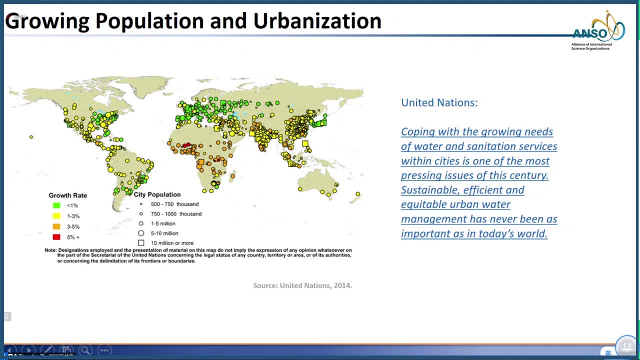 States and some other places, most of other places are facing a pretty fast growth rate, right So from three to 5%. you know, in Africa, in cities, China, India, and also there are more cities- that has a one to 3% growth rate. So in the same report, United Nations says: 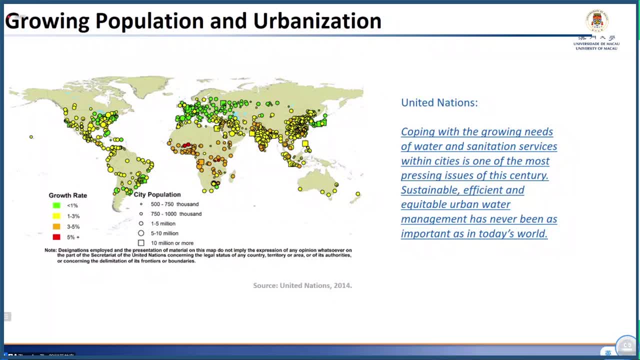 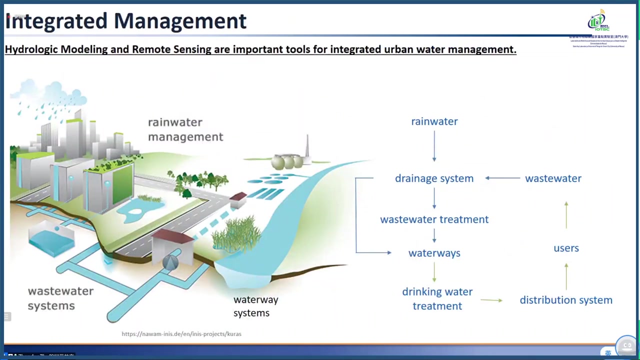 coping with the growing needs of water and sanitation services within cities is one of the most surprising issues of this century, And sustainable, efficient and equitable urban water management has never been as important as in today's world. So why do we need to talk about that? So, first coming back to the, the topic of today's 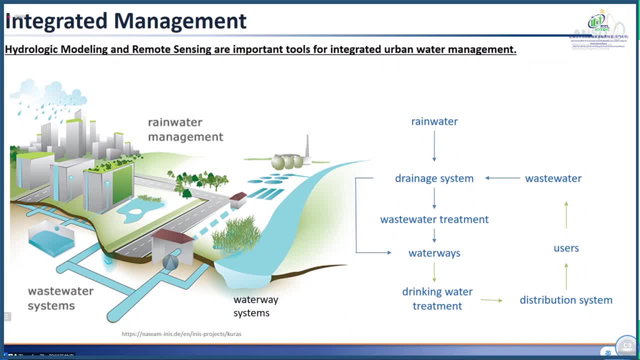 class. hydrological modeling and remote sensing are very important tools for integrated urban water management. right By integrated management, I mean the rainwater management, wastewater management and surface water groundwater management. all should be integrated And actually the are. I'm not going through the details of this cycle but, as you 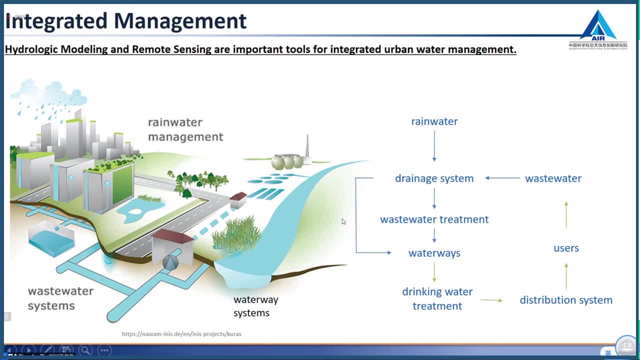 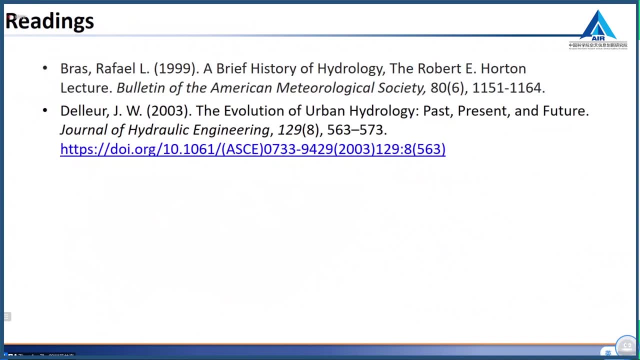 can see, the rainwater, wastewater and surface water are actually, you know, very closely connected. Okay is the chapter one, And I have two recommended readings for you. if you are interested, You know, in this brief history or in urban hydrology, you may want to read more about it. Okay, So. 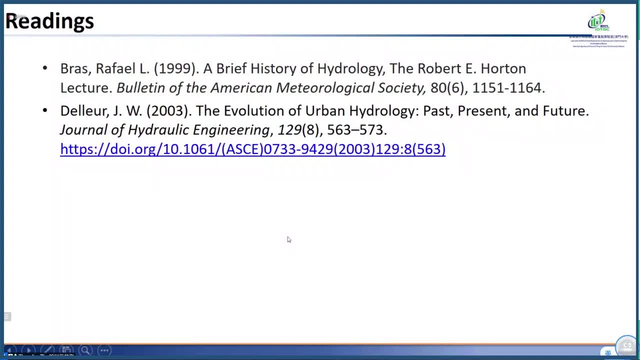 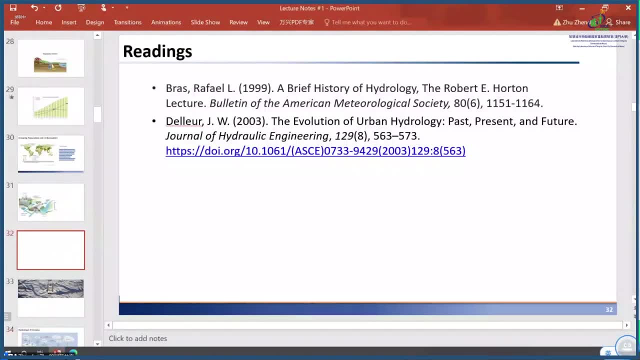 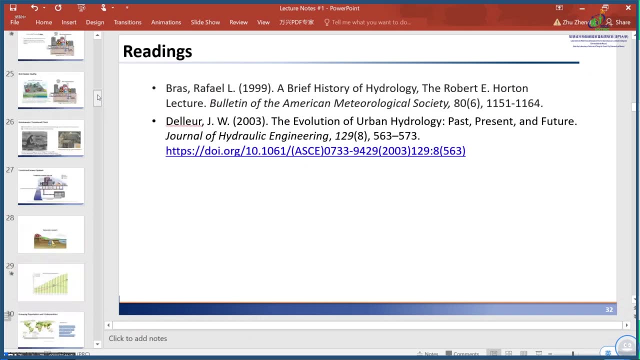 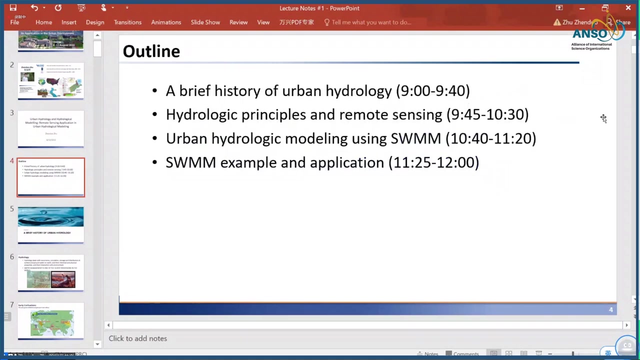 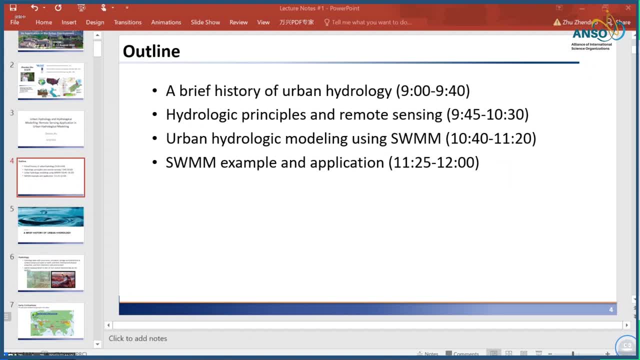 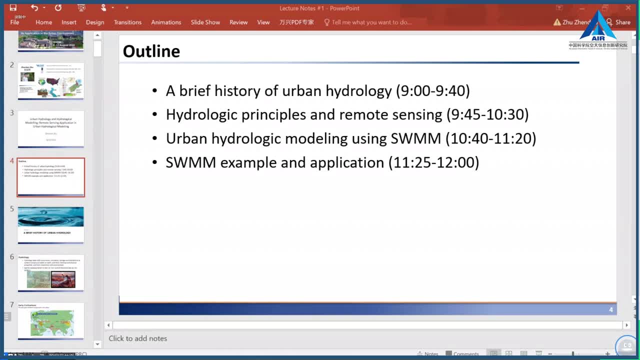 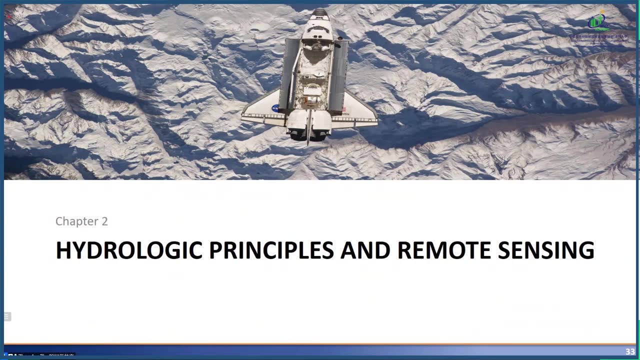 can come back at 955. Especially if you have been. I think a lot of things have been covered by different instructors, So I will try to go quickly here. So my goal for chapter two is not to introduce, like, the technical details of remote sensing. 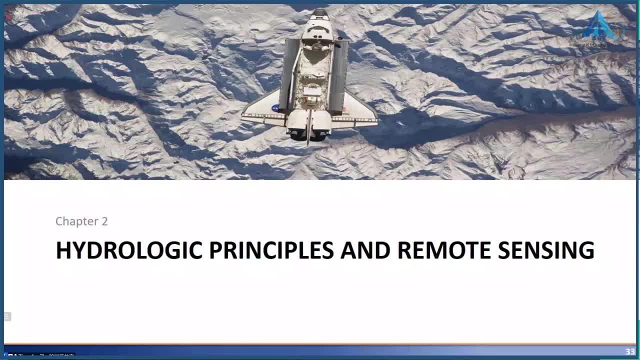 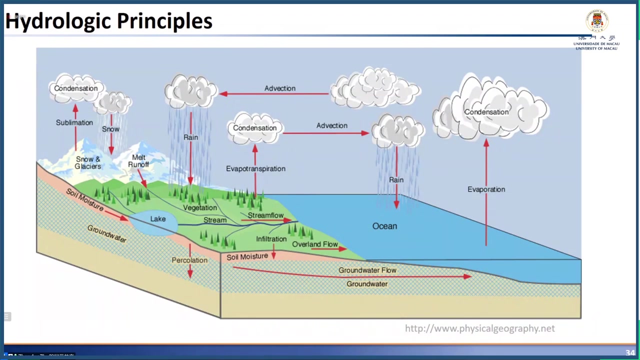 or hydrologic principles, but to introduce you that, how remote sensing can help with hydrologic principles And also we need to understand those hydrologic principles in order to do hydrologic modeling in the next chapter. Okay, So coming back to this figure of hydrologic cycle. 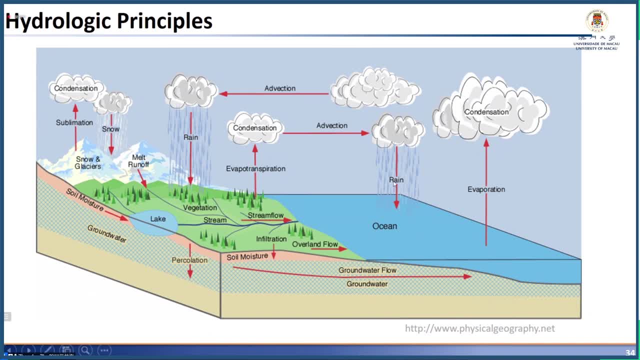 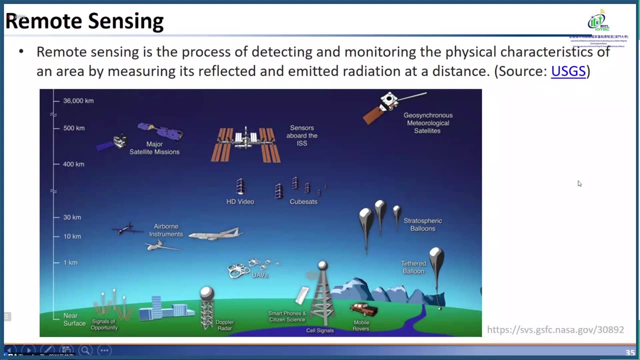 and a lot of those processes are actually quite important, So we basically have to understand each of them. So in remote sensing, as you may have known that this is the process of detecting and monitoring the physical characteristics of our area by measuring, is reflected. 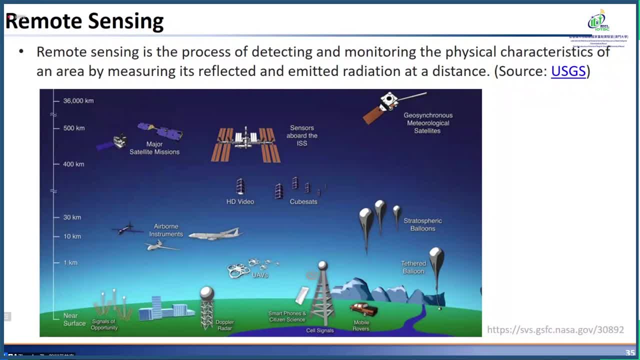 and the emitted ization at a distance. Okay, So, as you can see from this figure, they are actually a lot of our different technology in remote sensing, right? So if we see from the distance, above the surface, So near surface, we have radar, we have cell signals, we can even have 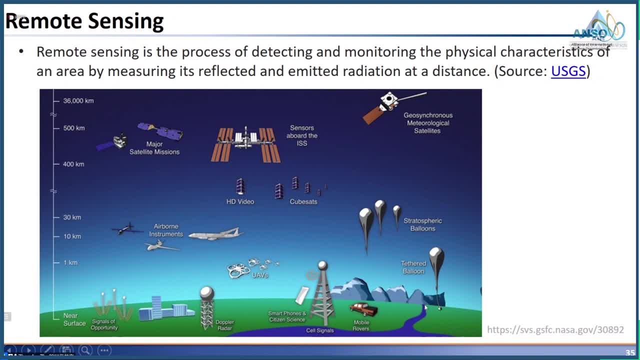 like mobile cars or like rovers balloon. This is a little bit far from the surface. And then, if we go further, we have airborne instruments, So there are like, obviously, satellites and so on. So all of those different remote sensing technology, again I don't think I. 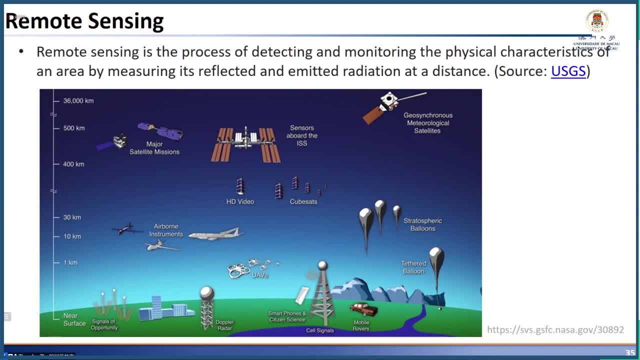 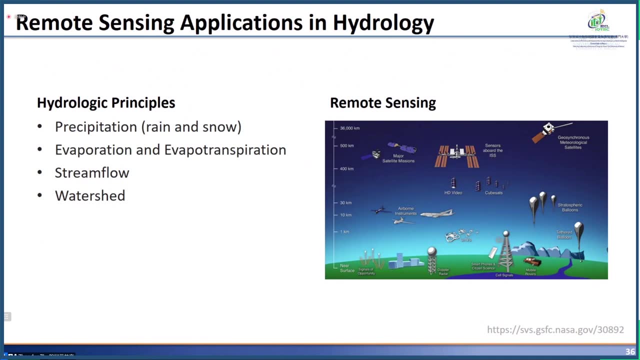 can cover all of them, but as you can see in the next couple of slides that they have been all very helpful for understanding hydrology, So I'm going to introduce one by one, hopefully very quickly, regarding hydrologic principles, including precipitation, both rain and snow, evaporation and evapotranspiration. 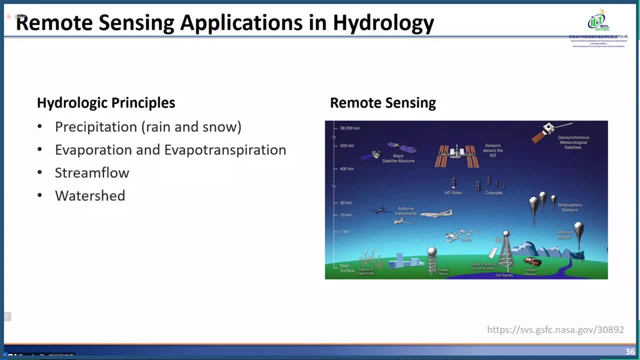 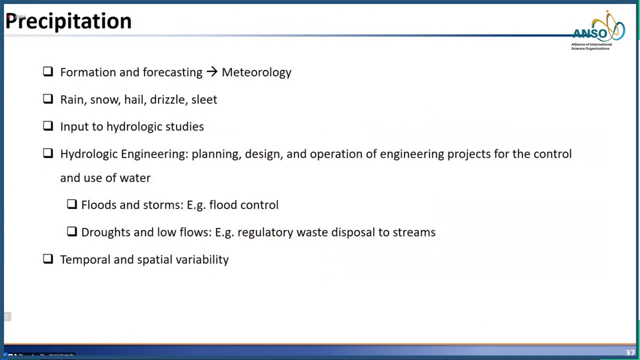 then stream flow, then watershed. Okay, so we will talk about how remote sensing can actually, you know, be applied to each of these hydrologic principles: Precipitation. So first, we are not going to talk about the formation or the forecasting. 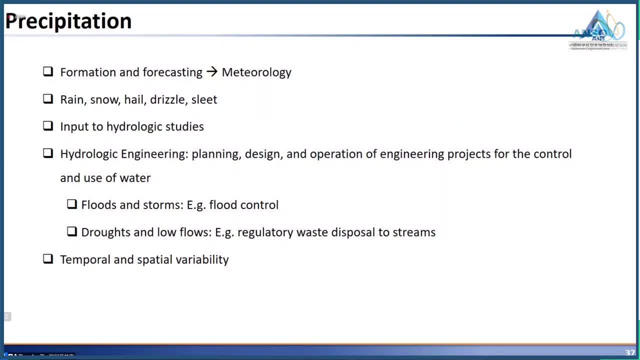 That belongs to meteorology. So then also precipitation includes different types, right. So rain, snow, hail, drizzle, sleet. So here we only focus on the two most common: rain and snow. So why we talk about precipitation? 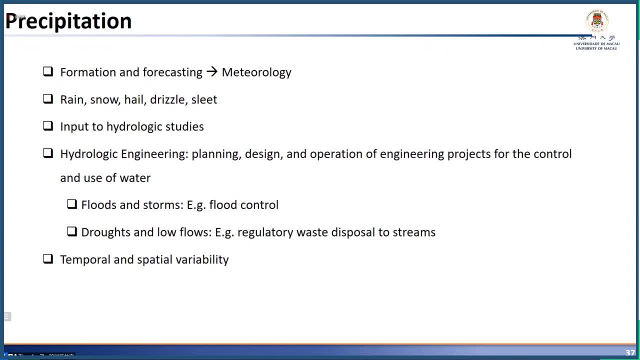 Precipitation first, because this is the first input to any hydrologic studies, right? So if you don't know precipitation, you know there is basically no hydrologic studies, right? So this is an essential input to hydrologic studies In hydrologic engineering. 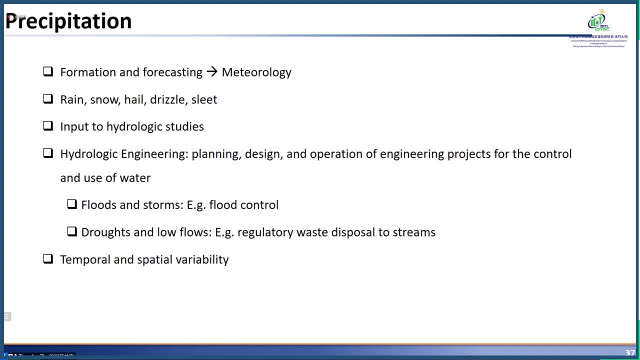 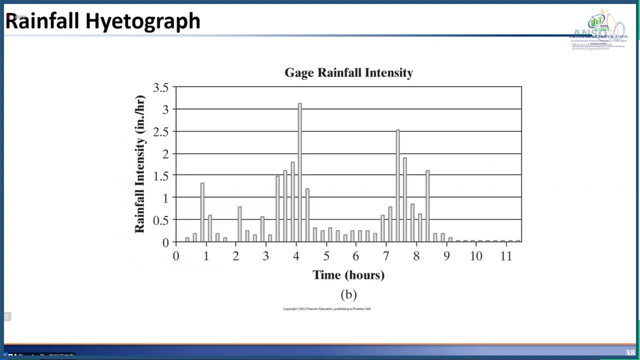 it is important for planning, for design, for operation. I will skip this. Also, we will briefly talk about the temporal and spatial variability and how remote sensing- you know techniques- can actually help to resolve some of that. Okay, So here, just to bring everyone. 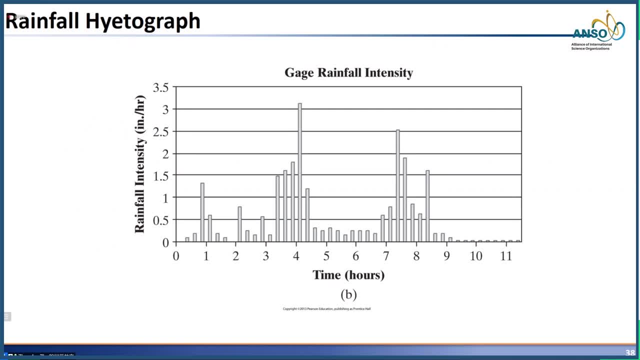 on the same page. I know many of you may have seen this or you know, have learned this before. So this is a rainfall hydrograph, right? So a rainfall hydrograph is a time series of rainfall intensity, right? As you can see, in the x-axis this is time in hours. In the y-axis it is rain. 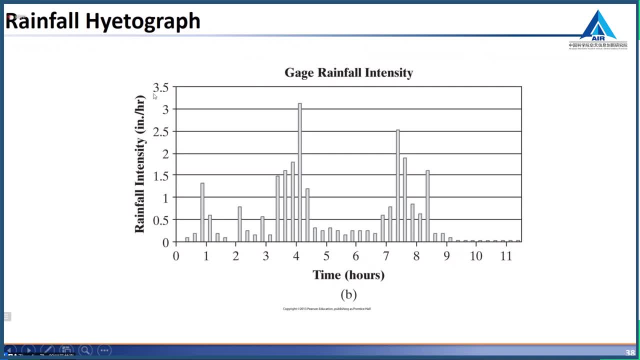 flow intensity Here is in the unit of inch per hour. It can be millimeter per hour, right? And if you plot it, plot this time series, this is a period graph, Okay, So obviously rainfall intensity is not uniform, right? So during one rainfall event it goes up and down, up and down, up and down, right? 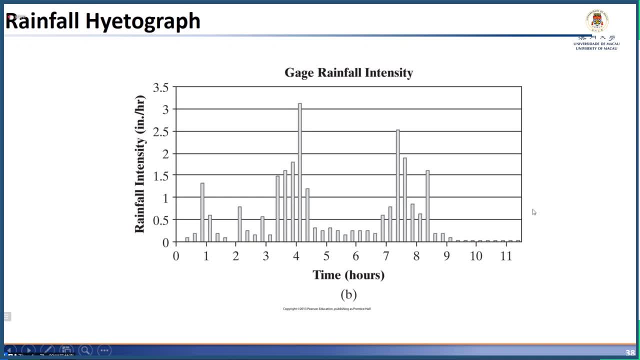 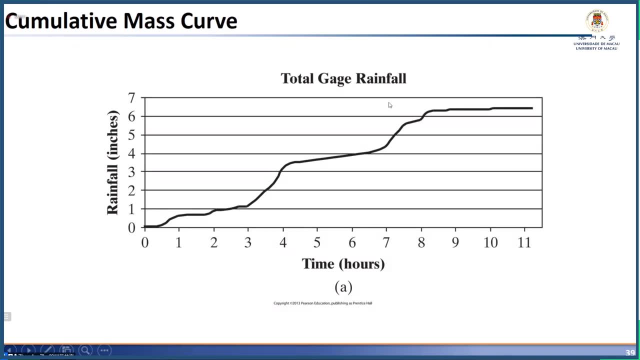 So rainfall intensity is uniform and during one rainfall event it goes up and down, up and down, up and down, down, up and down, right? So it is not a constant or uniform. So another way to represent rainfall is the cumulative mass curve, right. So again here, x-axis is the same, is time, but the y-axis 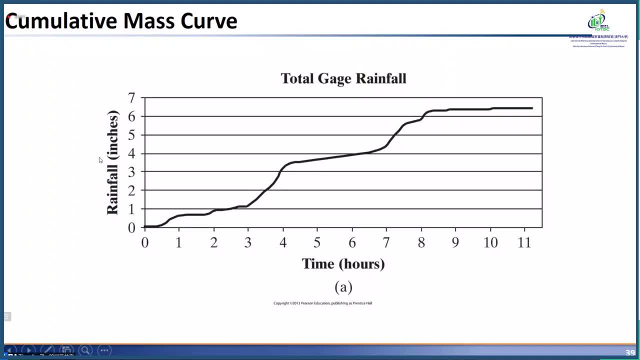 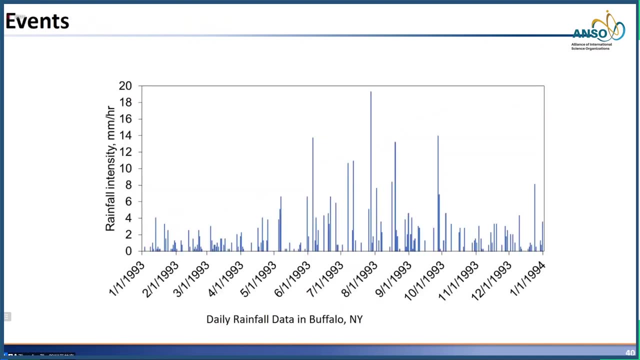 instead of rainfall intensity. this is the cumulative rainfall depth, right? So because it's cumulative, obviously it starts from zero and goes until the end of this rainfall event. So events okay If you look at a long time series of rainfall records, okay. so here is the example. 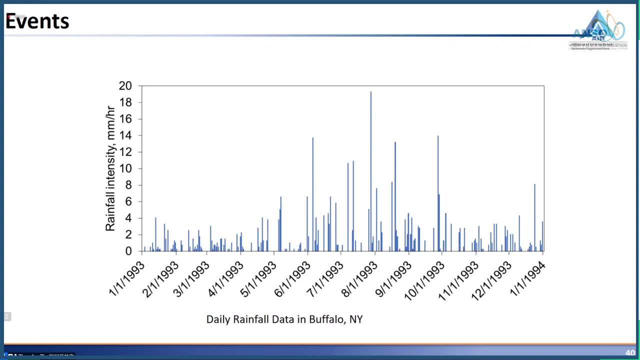 of the city of Buffalo in New York state in the United States In 1993, right, this is the time period from January until December of 1993.. And as you can see that, the rainfall intensity: right, so sometimes okay if you look at this as example. right, so this looks like one continuous. 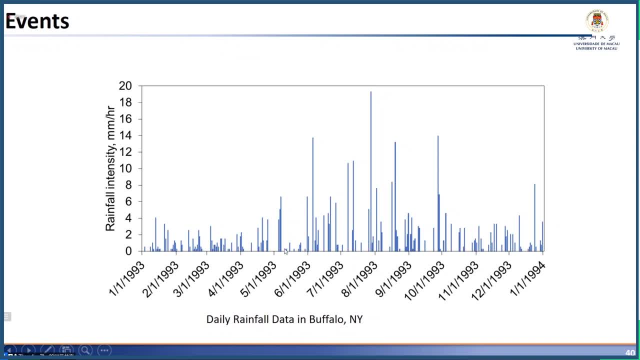 rainfall event- right. Then there is a dry period, then another rainfall event- okay, But sometimes it won't be that clear, right? So, for example, here there is a dry period which is very short, So do we consider this as one event or two events, right? 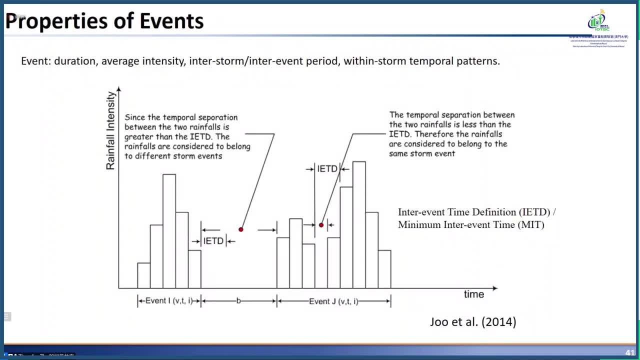 So this is a problem For determining rainfall event, right? so we need a concept called inter-event time definition, IETD, or a minimum inter-event time, MIT. okay, So this means if we consider these two events, right so? 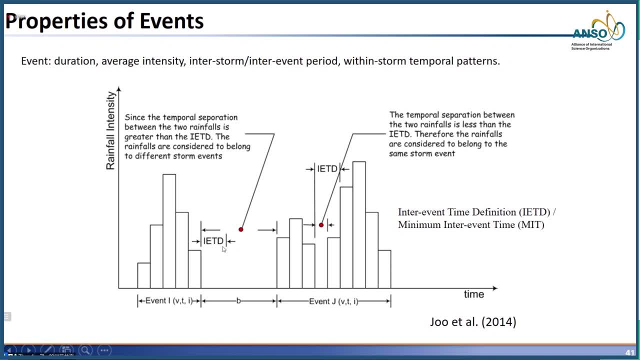 if the dry period B is larger than IETD, then they will be considered as two separate events, right? But if B is smaller than IETD, then here, for instance: right, so this dry period is smaller than IETD, then this will be considered as one event instead of two events, right? 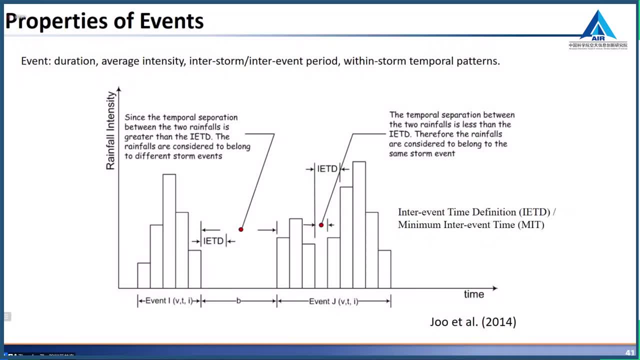 So we don't have much time to get into the details. There are actually something pretty interesting about this definition and I think a lot of research could be done. but for today, like it's just a brief introduction, And after defining rainfall events, 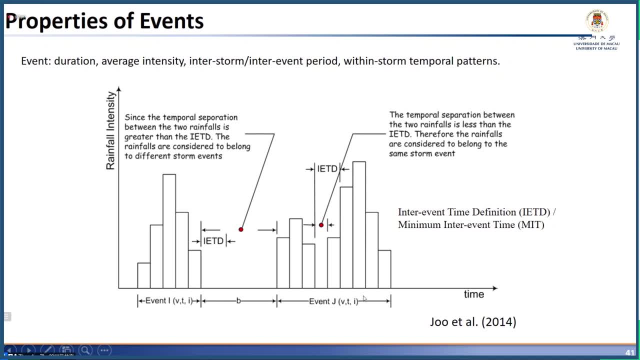 right after determining these rainfall events. so the properties of rainfall events include duration, intensity or the average intensity, so the inter-storm or inter-event period, and then also the within-storm temporal patterns, okay, So all of those are very important. 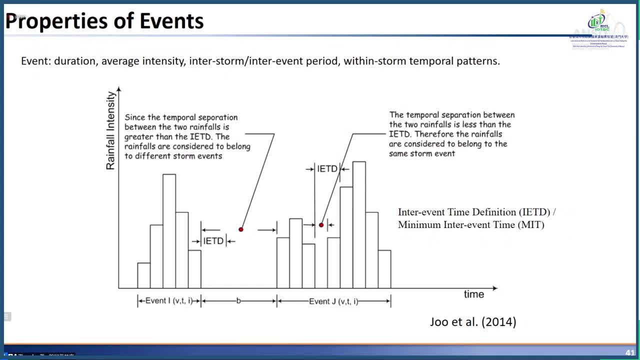 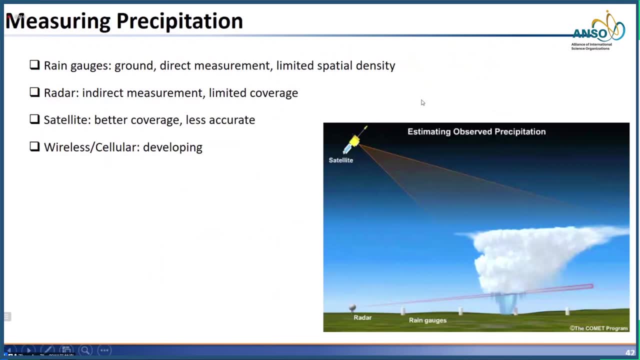 properties and when they are different. so for different rainfall events the hydrologic response can be pretty different, right? So for measuring precipitation, there are basically four types of measurement. One is rain gauges- right So, those are ground-level rain gauges. right So, those are ground-level rain gauges. right So, those are ground-level rain gauges, right So those. 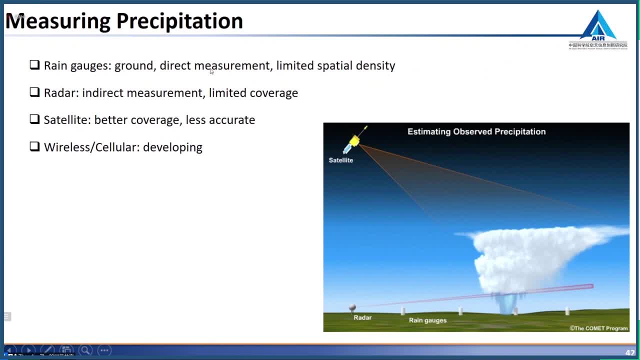 are ground-based and direct measurement. but obviously you know this is difficult to cover spatial density right, So it has very limited spatial density. Then the next one, radar. So this is indirect measurement. It still is limited coverage so you cannot rely on one radar to 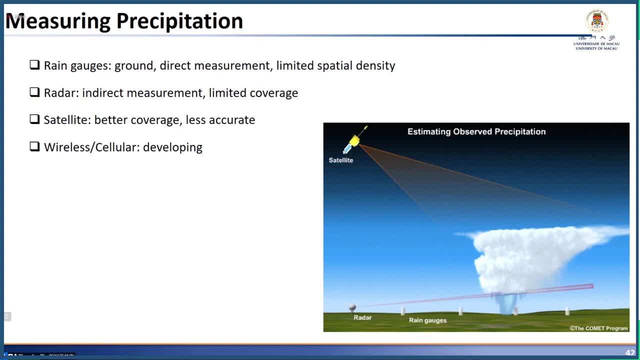 cover all area, right, You have to install a system, a system of radars, to cover a large area, right? So then there is satellite. Obviously, satellite has a larger spatial coverage than radar, but the problem or the drawback is it also becomes. 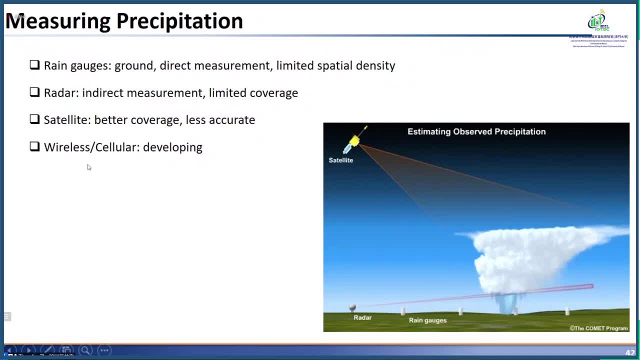 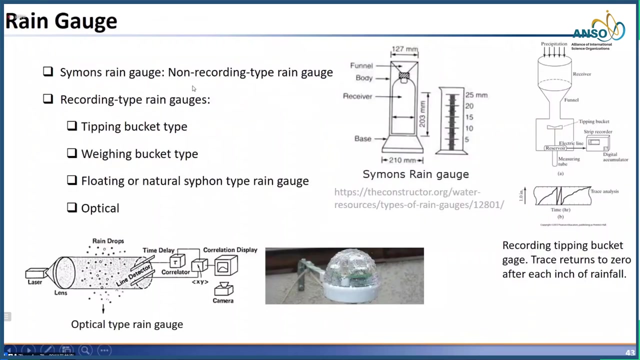 less accurate. okay, Finally, the last one is not discussed much, but I want to introduce this pretty interesting technology based on wireless or our cellular signals, but it is still under development. Li Zhouyang Zhou, Li Zhoujang, So the rain gauge. you know there are different types. I will go very quickly, right. 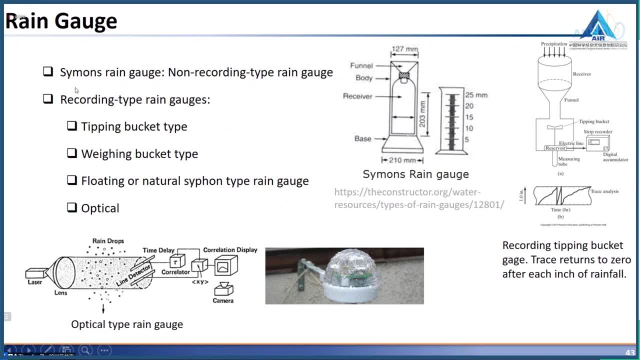 So the most simple one is a Siemens type rain gauge. This is a non recording type, So basically a Boto receiver: Li Zhoujang-Hui, Li Zhoujang-Hui An, Li Zhou' Kun, Li Zhoujang-Hui An. uh, then, after each rainfall event, uh, some, some, somebody has to go and check and read this right. 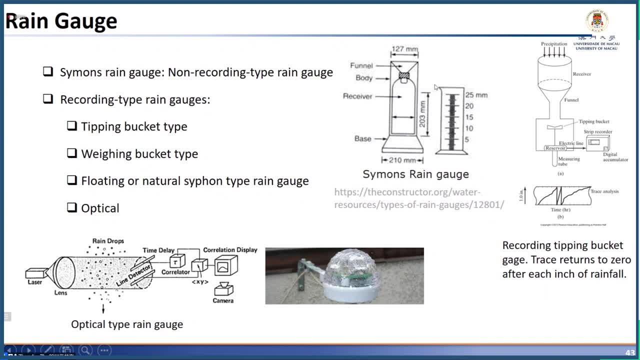 and, obviously, if the rainfall is more than the uh capacity of this uh, um then you know, uh, you, you will, you will not know the real uh rainfall depths, right? so then there are recording type rain gauges, uh, such as the tipping bucket type uh like this: so this tipping bucket, uh, basically. 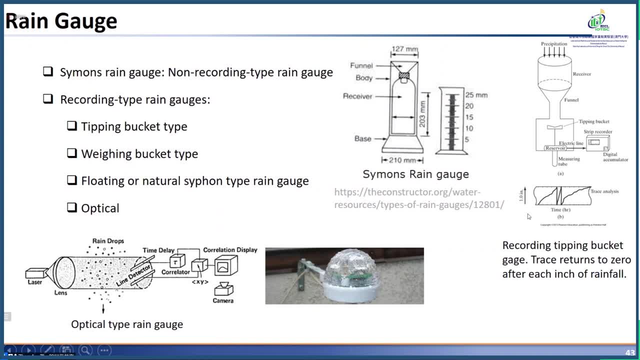 uh, every one inch, uh, it will reset. okay, so it goes from zero to one, then back to zero one, zero one, okay, uh, so all of these are recorded automatically. uh, and the wing bucket type, uh, then you know a floating uh tab, then the optical tab actually use a similar technology, the same technology. 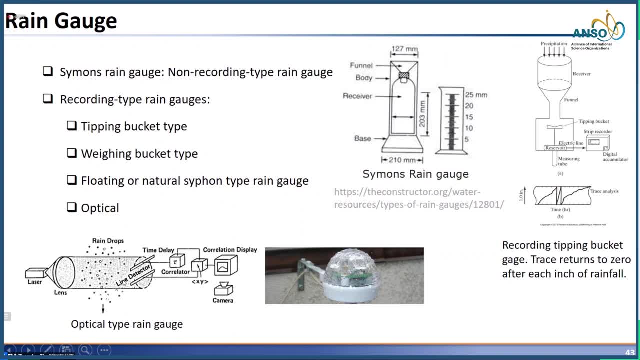 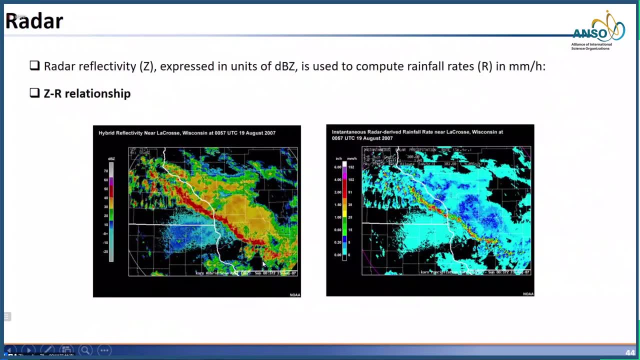 as remote sensing, right, uh, only thing is it's not quite remote, okay, uh, but uh, it is still based on the reflectivity uh. so those are the rain gauges uh, the radar uh, so based on the radar reflectivity, z uh, and then uh, by developing a relationship between z and r and the radar, uh reflectivity. 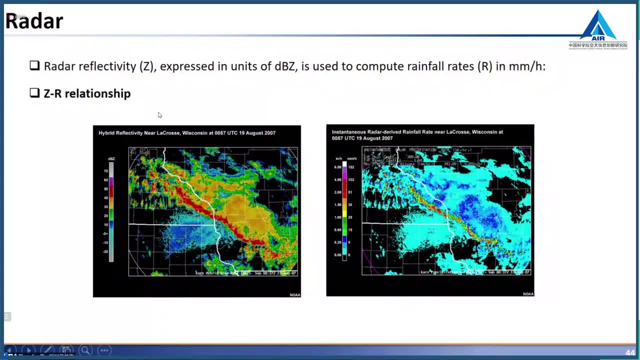 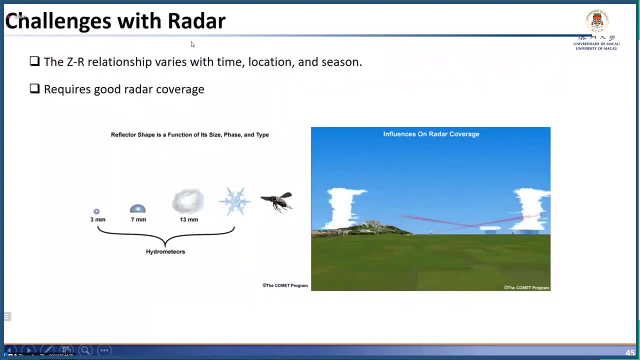 and the rainfall rates uh. then, by measuring uh reflectivity uh, we will know or we can estimate uh uh rainfall intensity. right, so this is the radar uh, the challenges with radar, or the problems with radar uh include uh. first, this relationship uh actually varies with time, location and season, so, uh, you have to be very 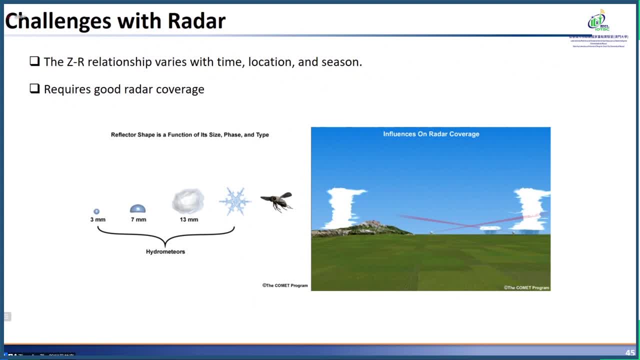 careful developing, uh, this relationship, and it has to be flexible and calibrated. uh, it also requires a good radar coverage, all right. so, for example, uh, as you can see here, right so, uh, if the event, the rainfall- is too far away from a radar, right then, this measurement is. 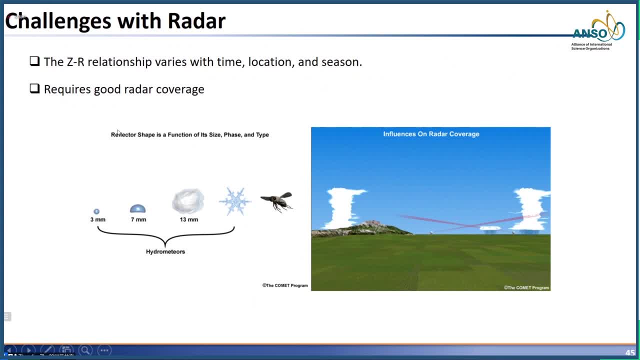 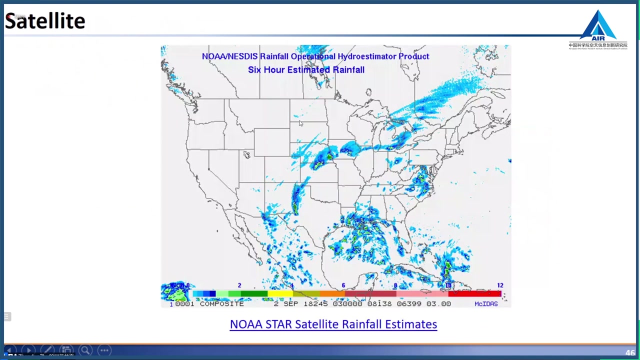 not going to be accurate. and also the reflectivity can be affected by uh different particles or different objects uh in the air, and not only uh rainfall, rainfall droplets, but if there is, for example, uh insects right, that will affect reflectivity as well. so for satellite, i will just quickly uh skip this similar, uh similar idea, as rather but. 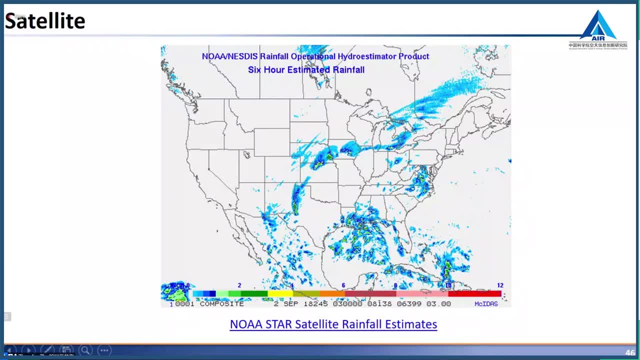 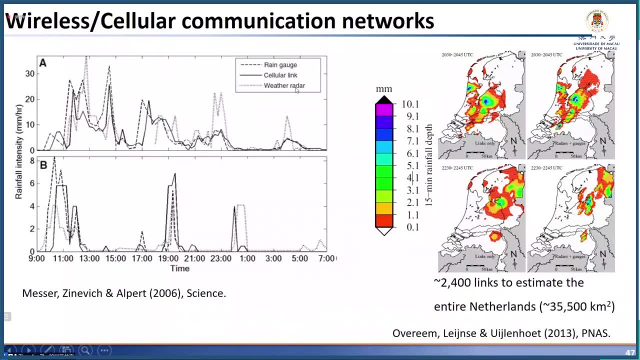 obviously this is uh with a better spatial coverage but, as we have said, uh less accurate. so the interesting one, uh is the process at home- is wireless or cellular communication networks, so basically based on the cell signal, right, so the cell signal is also affected by rainfall, right, and this effect could be translated, or? 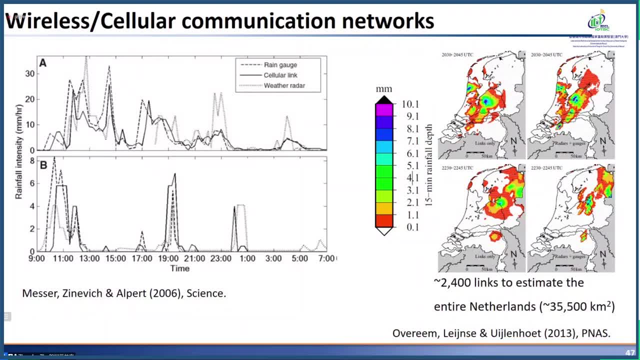 you know, calculated for rainfall intensity, okay. so the concept was kind of proposed and proved in 2006 and published in science. as you can see, for this ringage, the comparison between the ringage, the cellular link and the weather radar are pretty similar and actually for some of them the cellular link is better, even better than radar, right. 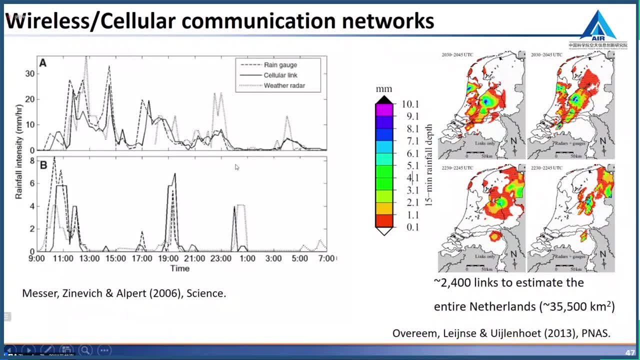 however, it is not very easy or convenient to adopt this technology then until 2013. so this is actually the first large-scale study using this approach, right? so this paper published in PNAS. so they started the entire Netherlands and used about 2,400 cellular links to estimate the precipitation or rainfall intensity. 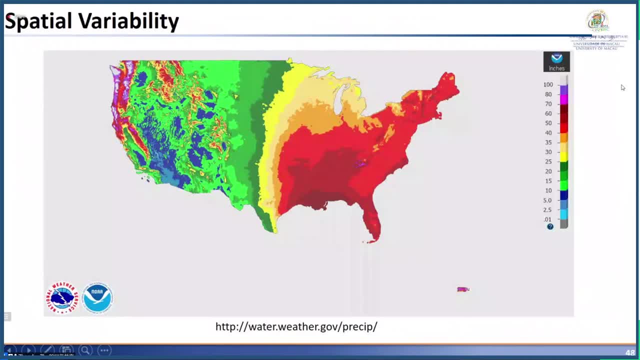 so for spatial variability, i think this is nothing new. here is an example of the United States. as you can see, this is the annual precipitation normal, a 30-year normal from 1981 to 2010. so obviously rainfall or precipitation is different at a different location. 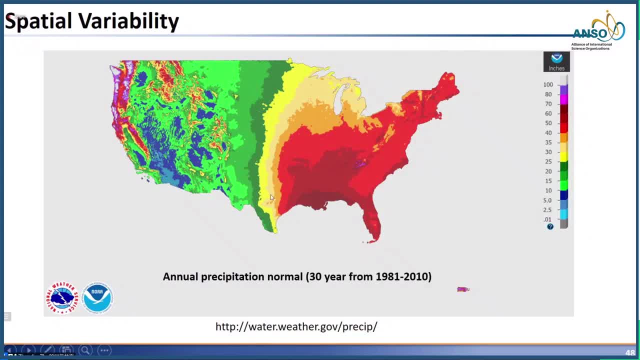 and this is more a new concept. it seems to be the case as well. yes, so let me give you a quick, brief introduction to the we know about the area. so when you think about the city, what you normally know about the city is that it is a super large city, right. so, like in the 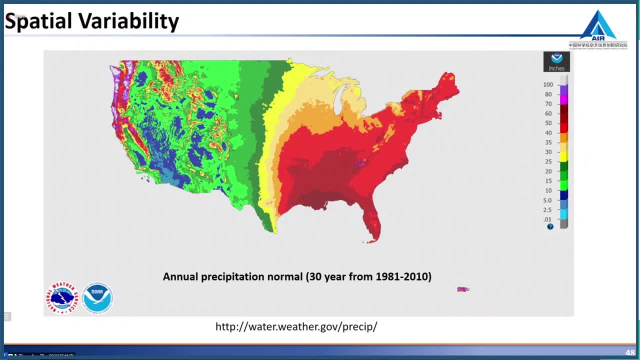 south of the field there is a large city. but you know, in the south of the city you might think the city is more like a city to set a standard in terms of transport and so on, but it is not the case. The city of England is not the hub of the city of England. 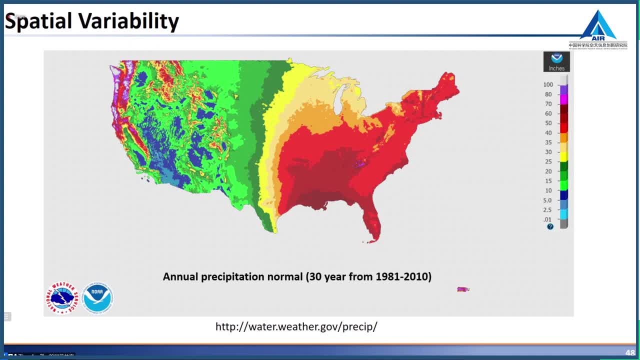 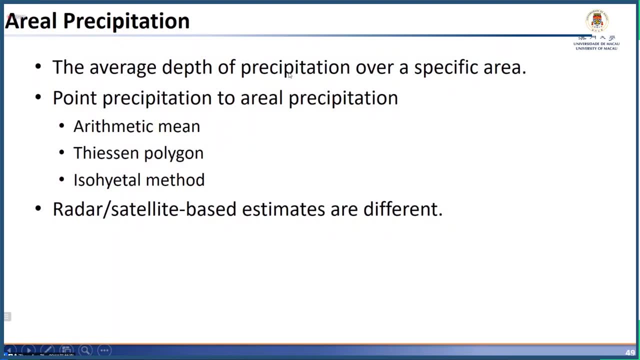 Okay, so if you guess it that way, I guess then the city of England is the hub of the city of England. Yes, a very big spatial variability. So for dealing with the spatial variability we have to, based on, for example, if it's the measurement of rain gauges, we have to do aerial precipitation. 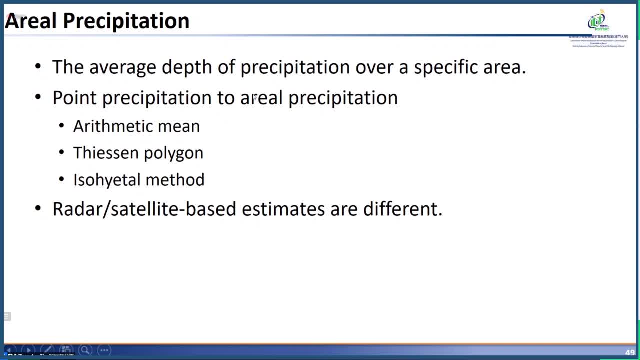 based on the point measurement. So there are different ways to do that. Again, I will just skip this very quickly. So arithmetic mean testing polygon, which is probably the most widely used. Arithmetic mean is pretty simple. This is the simplest, This is maybe the most. 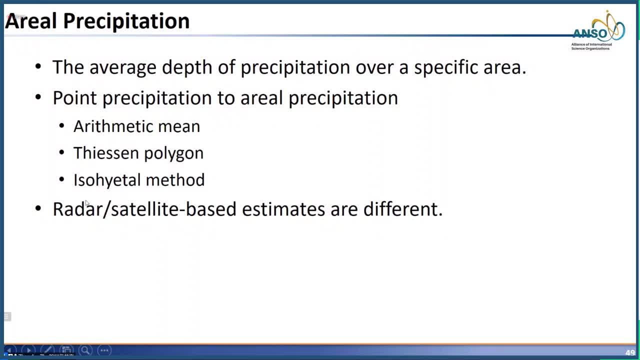 widely used Isohelter method is believed to be the most accurate, but it's not very widely used because it's not really convenient. So every time when the rainfall enters, the intensity or rainfall depth change, the isohelter lines will change. So this is different from 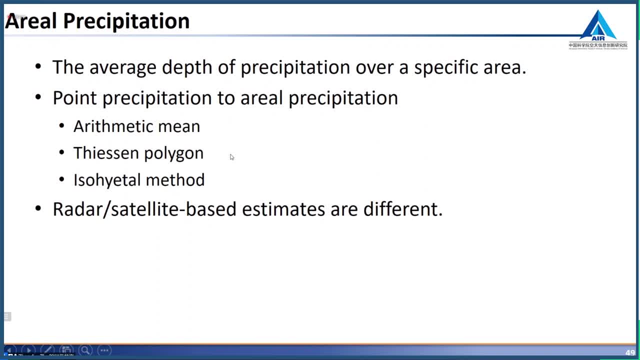 testing polygon, because testing polygon only depends on the location of the measurement, But isohelter, this will depend on the measurement itself. Obviously, the radar and satellite based estimates will at least part of the measurement. So what are the characteristics of the isohelter measurement? So the distance: 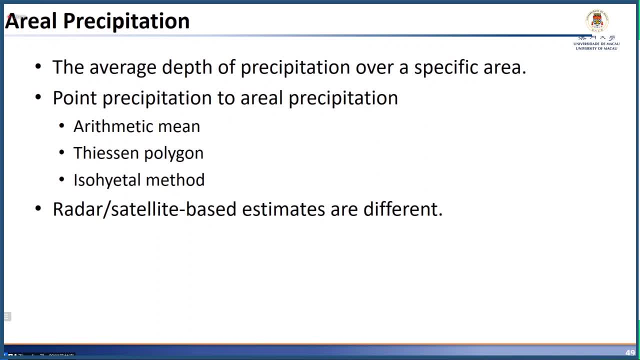 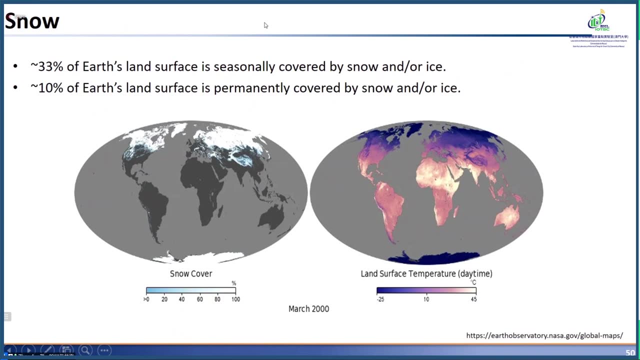 from. the заoilter of the measurement is the distance between the signal and the signal length. Smell is also based on the near distance between the signal and the signal length. This is theocal measurement Like this is a measurement here And then the distance. 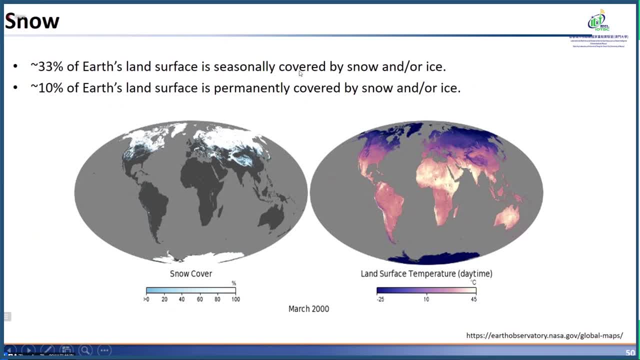 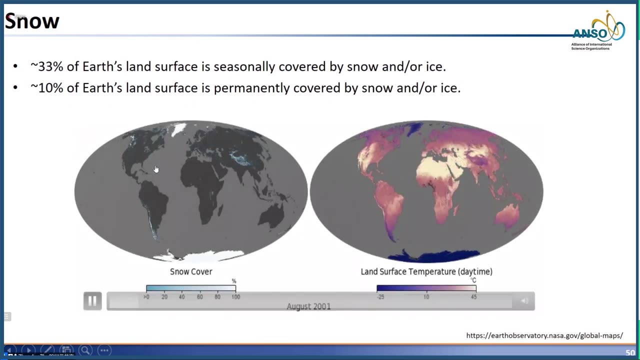 Let's make a little bit of an example of the area that we can use to estimate the judgment: snow or ice, And about 10% of the land surface is permanently covered by snow or ice. So here is a measurement Again. this is: 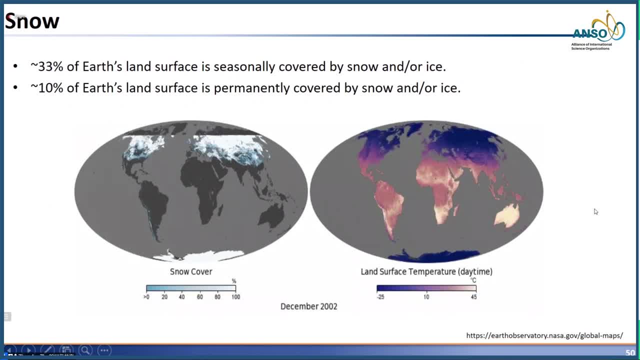 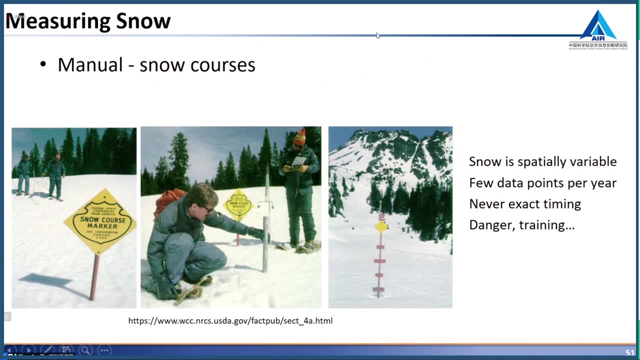 based on remote sensing. This is based on remote sensing measurement of the snow cover and land space temperature. So if you don't have remote sensing, measuring snow can be difficult. This is not an easy job, So the manual measurement is to use the snow causes. So those are like vertical marker that you 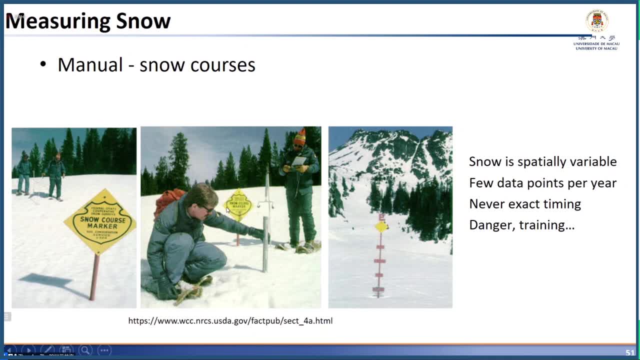 know you can put through the snow and then measure snow depths, right, based on those markers. So obviously it's not very accurate, right? Because the snow is spatially variable, right? So here you can only measure at one specific. 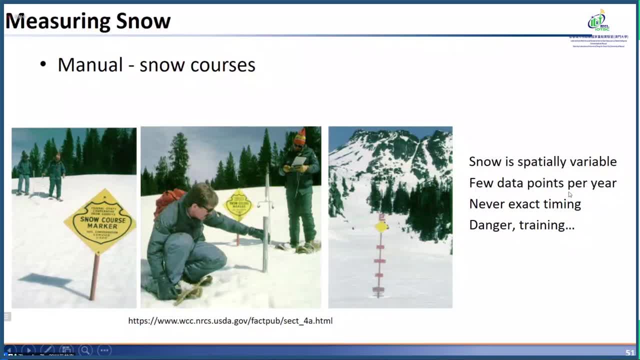 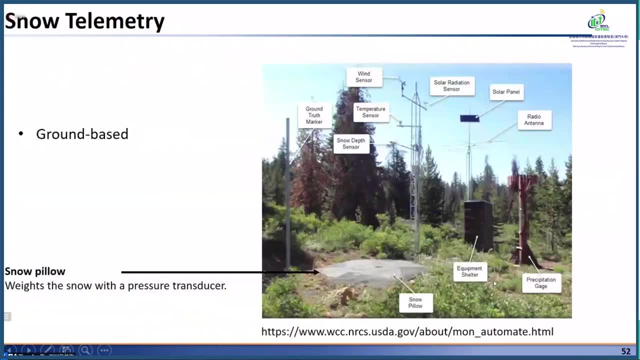 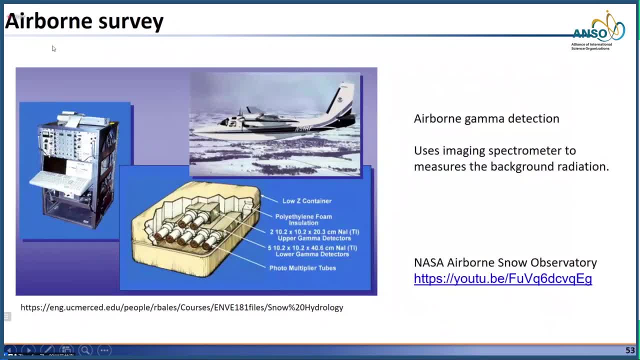 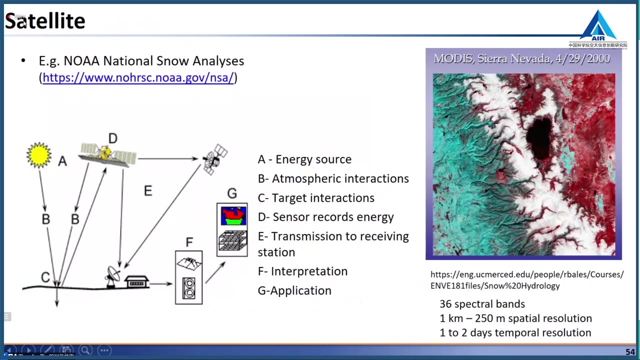 of sensors have been used for this And also the airborne survey, So these can be used for metro snow. So if you are interested, there is a pretty good video by NASA. talk about their snow observation project And also satellites. So just to. 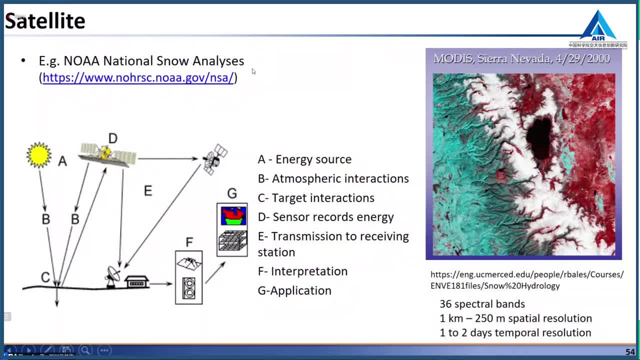 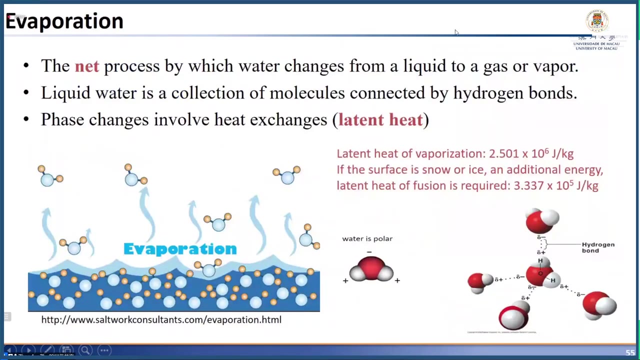 give one example. like NOAA has this national snow analysis based on satellite. And here is another example, you know, using the MODIS satellite images to measure snow depths: Evaporation. Okay, so evaporation is the net process by which water changes from liquid. 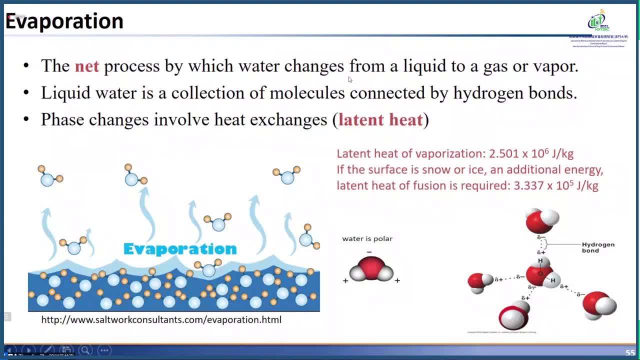 to a gas or viper. you are very familiar with this. now. One thing to point out is that the phase changes involve heat exchange, So this is called the latent heat, And obviously this needs energy. So from water to gas or vapor, it will need energy, And from snow or ice to gas or vapor, it will need more energy. 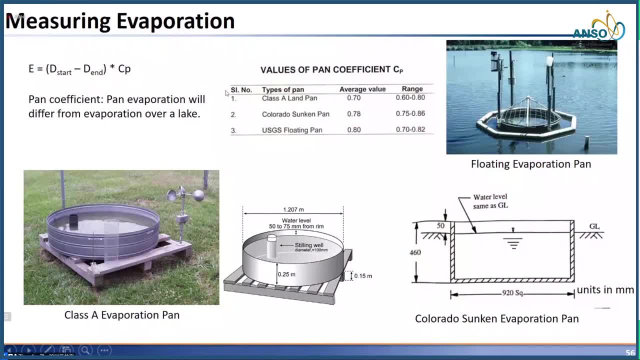 So the measurement of evaporation is to use PAN. So, as you may remember, even the first measurement of the Mediterranean Sea evaporation is using PAN or used PAN. So there are different types of PAN. So the class A land PAN. this is sitting on top of the ground. 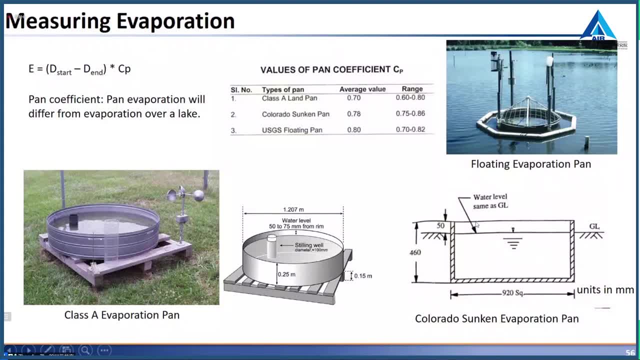 There is also a Colorado sunken PAN, which the water level is kept at the same as the ground level, So this is digged into the soil And then there is a floating PAN that is in the middle of the open water. So because of the measurement technique, so the evaporation from a PAN, 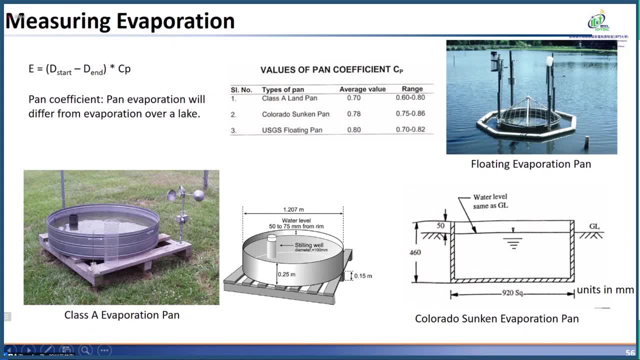 is going to be faster than the natural evaporation in open water. So therefore you need a coefficient to collect this measurement, right? So this coefficient is less than one, Right? It's because the evaporation in a PAN is faster, So this is more than. 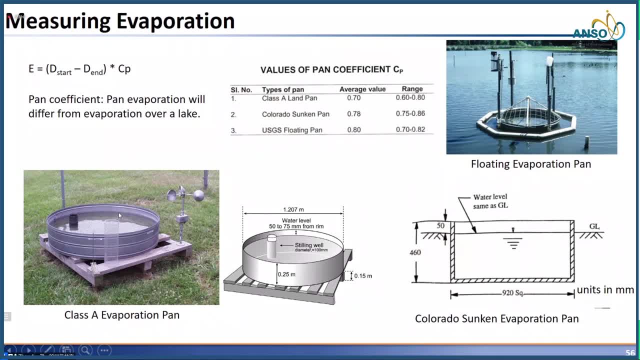 reality or more than open water evaporation. So the coefficient can change from 0.7 to 0.8 at average. Of course there is a range, So we can also usefine on lower Generalкую scale to measure evaporation. 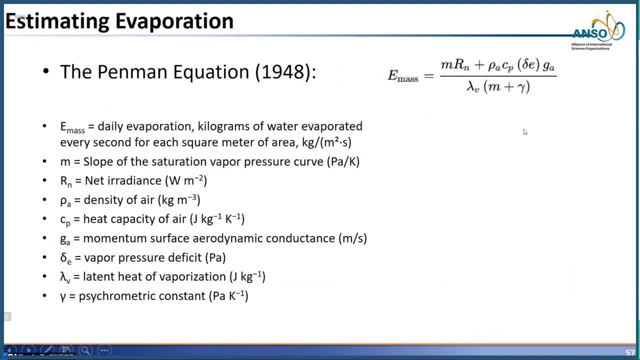 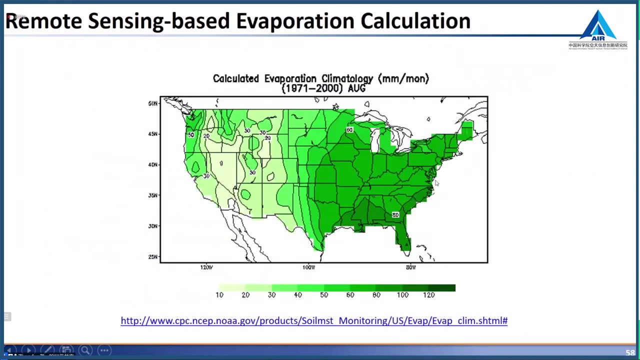 So we can also use a different. 1- use remote sensing technology to estimate evaporation using the Penman equation. So this is Penman equation. Those are the measurements you need to estimate evaporation. So I'm going to skip this. And here is a results right, here is a. 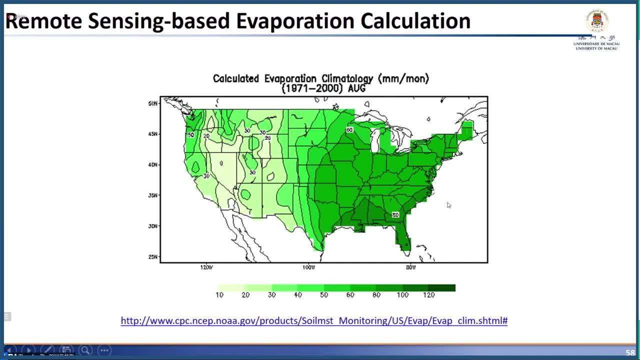 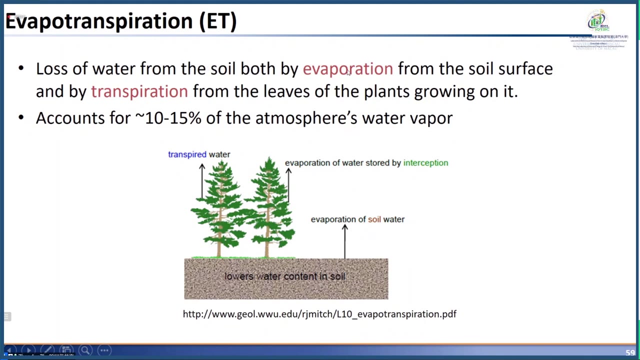 calculated evaporation over the US. So this is average in August from 1971 to 2000.. This is millimeter per month of evaporation. Evapotranspiration: this is a loss of water from the soil both by evaporation and the. 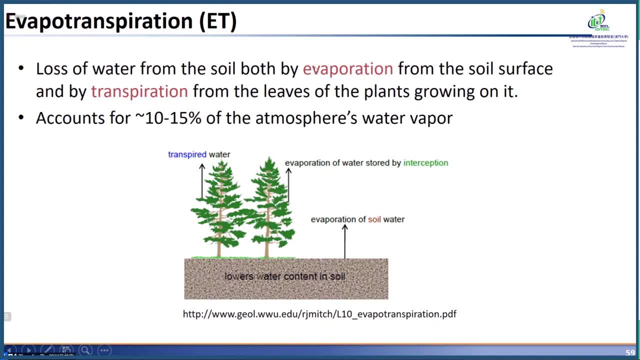 transpiration. So it's actually a combination of water and evapotranspiration. So it's actually a combination of water and evapotranspiration. So it's actually a combination of two processes: evaporation and transpiration. So evapotranspiration, or ET, is quite important. It accounts for 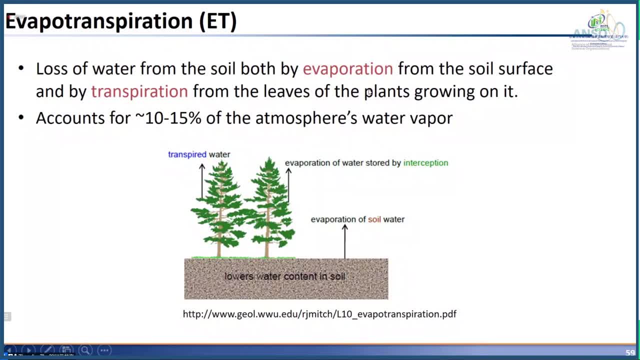 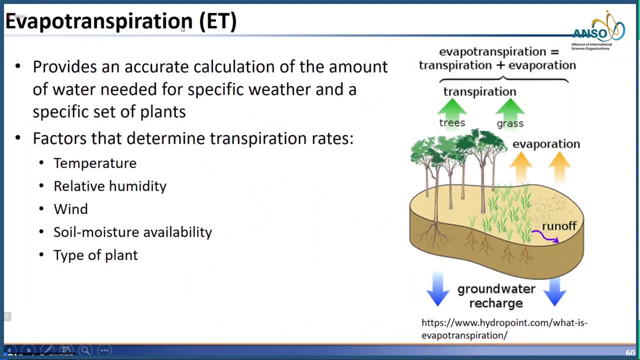 about 10 to 15% of the atmosphere's water vapor And to provide a ET also provides an accurate calculation of the amount of water needed for specific weather and specific set of plants. However, it is pretty complex because it depends on different. 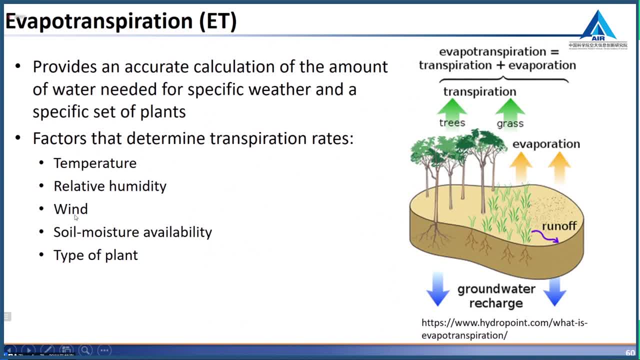 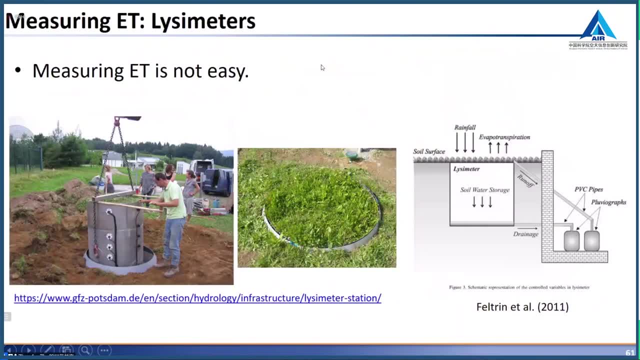 factors right, such as temperature, relative humidity, wind, soil moisture and the type of plant, And measuring evapotranspiration is really not easy. So, just to give an example, there is actually no like standard equipment. there is actually no standard equipment to measure this. So this: 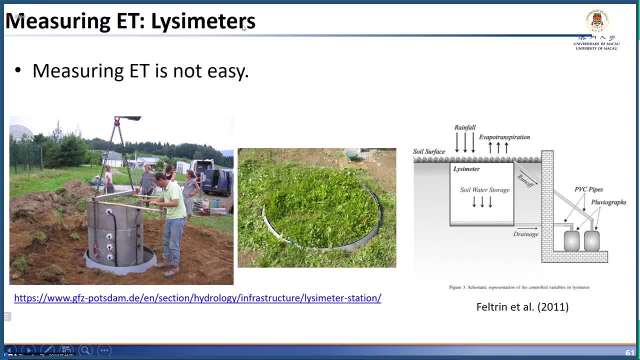 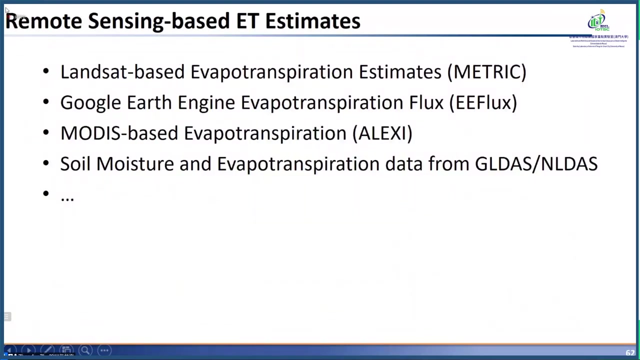 measurement is called less meters, So basically based on a water balance calculation. So you measure rainfall, you measure soil storage, you measure runoff, then, based on water balance, you calculate evapotranspiration. However, thanks to the remote sensing technologies, we can measure the. 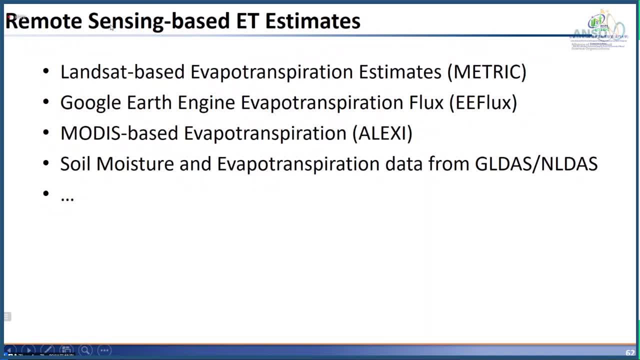 evapotranspiration. There are actually a lot of remote sensing based evapotranspiration estimates, So I'm just giving examples here: the Landsat based Google Earth Engine models based, and there are also data from GLDS or NRDS for soil moisture. 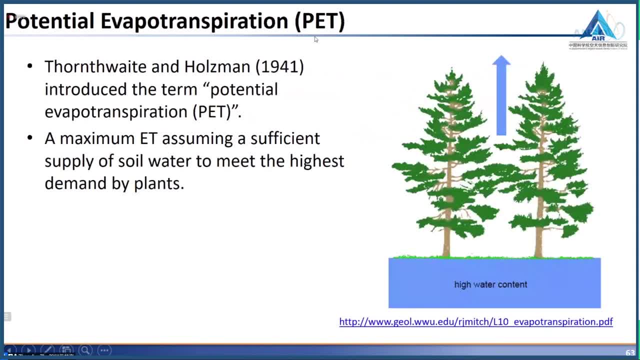 and evapotranspiration. So potential evapotranspiration is an idea introduced in 1941 by Southweed and Holtzman. So the idea is: imagine if you have a sufficient water supply, if you have a sufficient supply of soil water, so the maximum evapotranspiration will be the 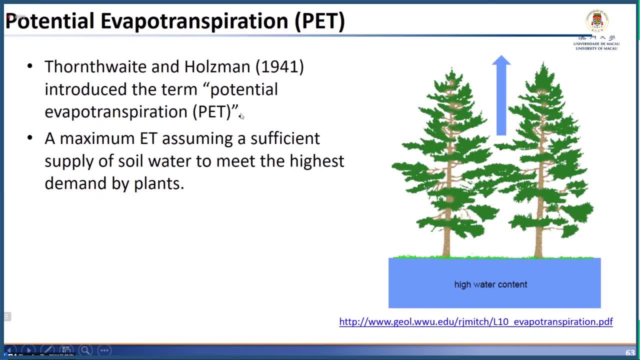 potential evapotranspiration And the idea is knowing that hopefully first knowing potential evapotranspiration is easier than knowing the time-varying actual evapotranspiration right, And then you can try to develop a relationship between potential evapotranspiration and actual evapotranspiration. 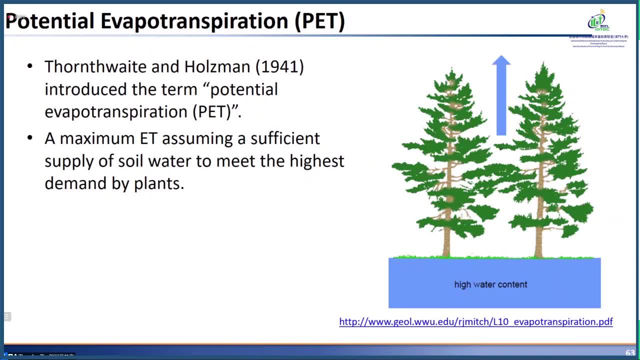 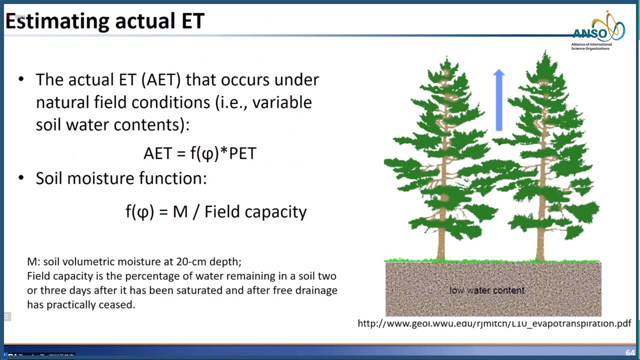 Then based on that, you can estimate the actual evapotranspiration right. So this is the whole idea why this potential evapotranspiration is introduced. So the actual evapotranspiration, or AET, that can be a function of phi times, PET. 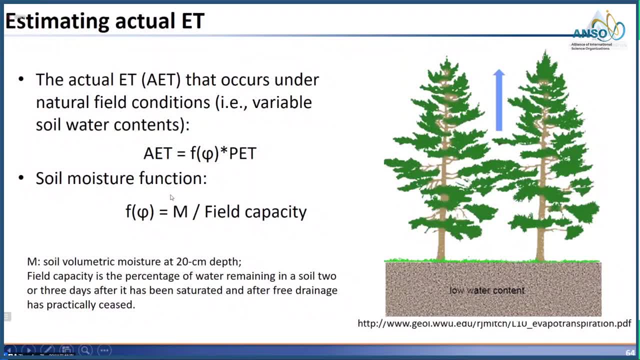 which is the potential evapotranspiration, And this F-phi is called as the soil moisture function because it mostly depends on the soil moisture right. So this M is the soil volumetric moisture at 20 cm depth and divided by the field capacity. 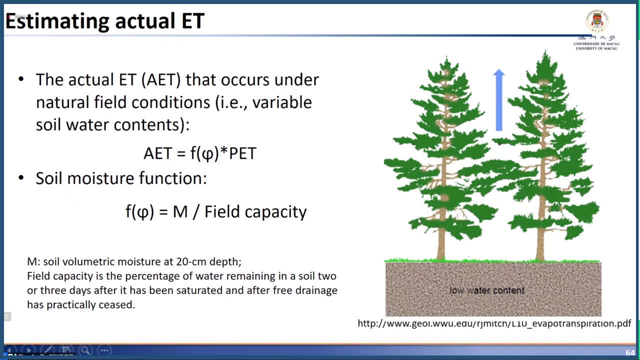 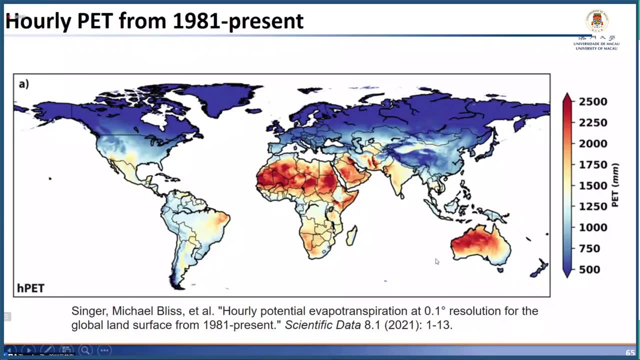 So this M is the soil volumetric moisture at 20 cm depth and divided by the field capacity. So this can be an estimation or a formula to calculate actual evapotranspiration based on potential evapotranspiration. And here is a database, again just as an example that we have: hourly potential evapotranspiration. 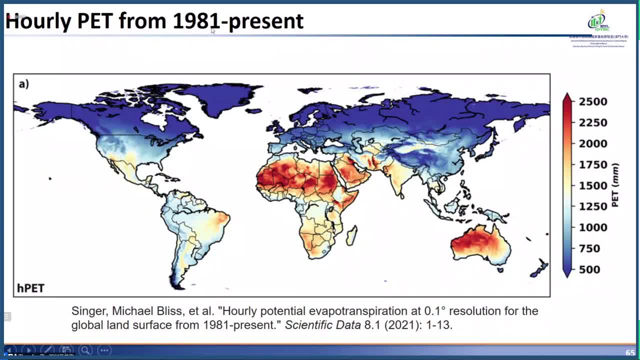 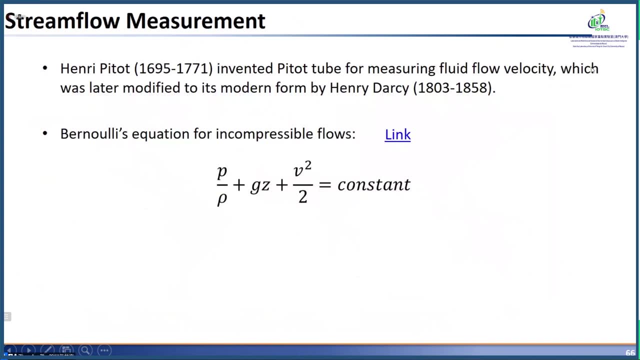 data globally from 1981 until present. If you are interested, you may want to check out this paper. So this is at a 0.1 degree resolution for the global land surface. So stream flow measurement. as we have said, Henry Pitot invented the Pitot tube for measuring. 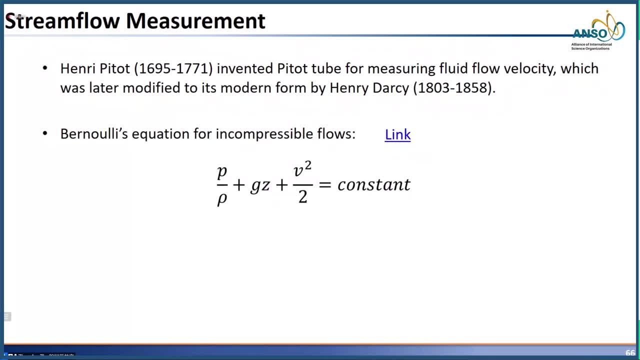 flow velocity. Since then we could have accurate flow measurement. So this Pitot tube is based on the Bernoulli's theory or Bernoulli equation. I'm going to skip this. There is a link here goes to a YouTube video. 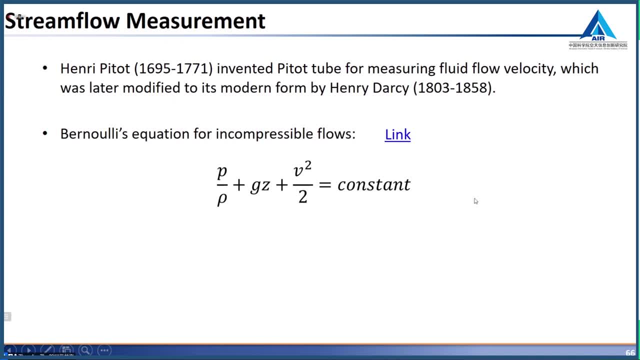 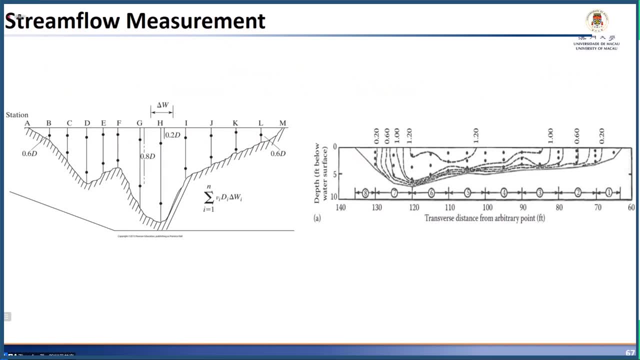 If you are interested, you can look at the explanation of the Bernoulli equation. When you measure stream flow in a river, keep in mind that you have to measure at different depths So you can measure at different locations of the cross-section. 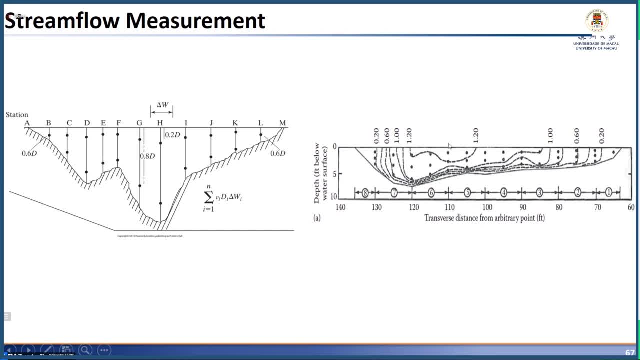 So that is because the water velocity is different from surface to the bottom and from the middle of the river to the bank of the river. So why they are different? in this need hydraulics. so it will need more time to explain that, But just keep in mind. 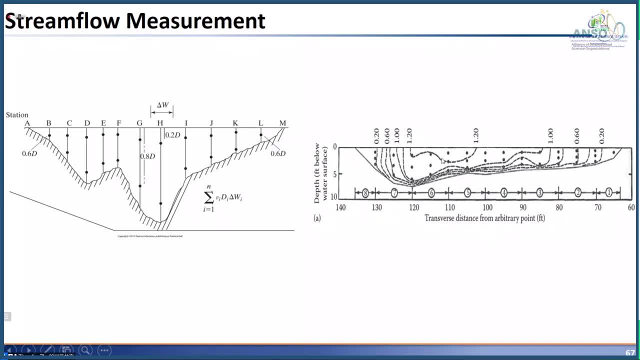 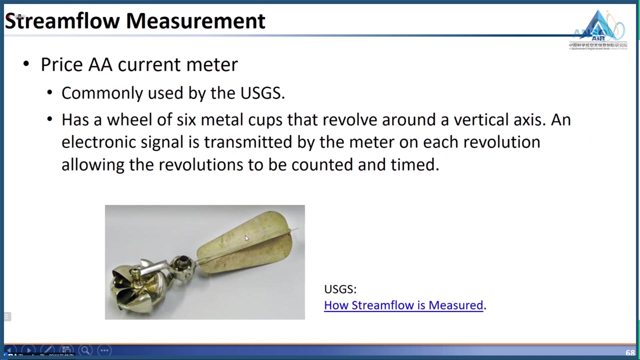 Because the water velocity is different. Because of this velocity distribution, in order to measure flow discharge at a cross-section you actually have to measure different places, which is quite time consuming and difficult. So this is like the manual measurement. So the measurement equipment. this is commonly used by the USGS, US Geological Survey. 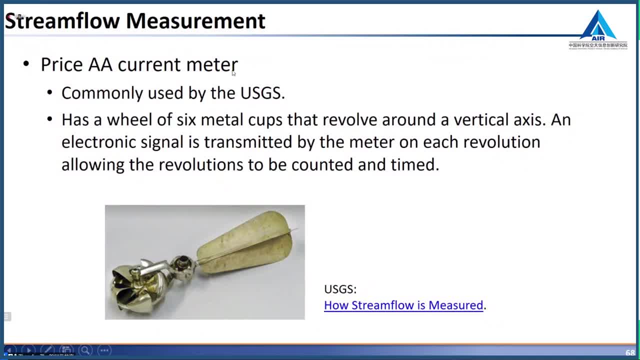 It is called Price-double-A current meter, So basically it has a wheel of six metal cups. then it automatically records how fast you know this. actually you know it will time and count how many revolutions. Okay, So if you are interested, there is a link for more information. 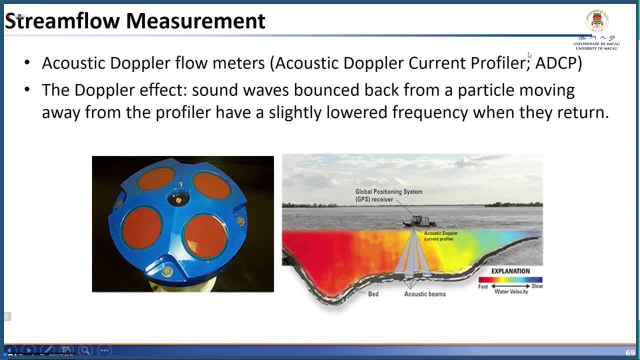 Okay, Thank you. Thank you. So then, the acoustic Doppler flow meters are called acoustic Doppler current profiler or ADCP. So this is based on the Doppler effect, which is the sound waves bounced back from a particle moving away from the profiler have a slightly lower frequency when they return. 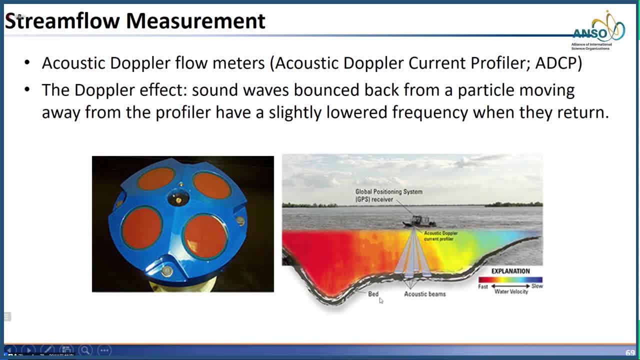 So by this, ADCP can actually measure area of a cross-section simultaneously. So yeah, simultaneously, almost simultaneously. So you don't have to take measurement at each location. And, by the way, keep in mind, when you do it manually, you have to measure for a certain time period, normally a couple minutes at. 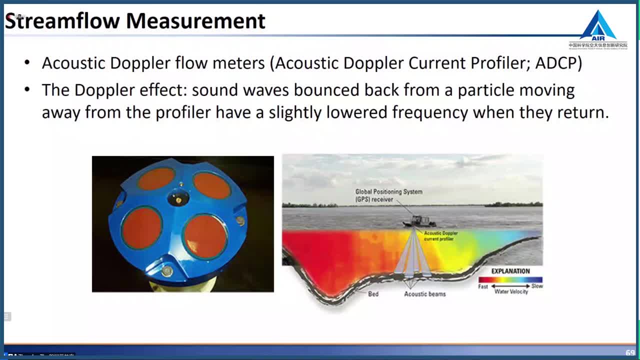 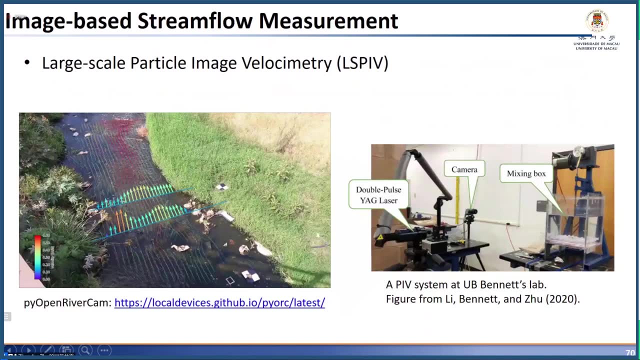 least in order to get the average flow velocity. So now you can get instantaneous measurement. Also very interesting is image-based streamflow measurement. So again, this large-scale particle image velocimetry, or LS-PIW, is still under development. 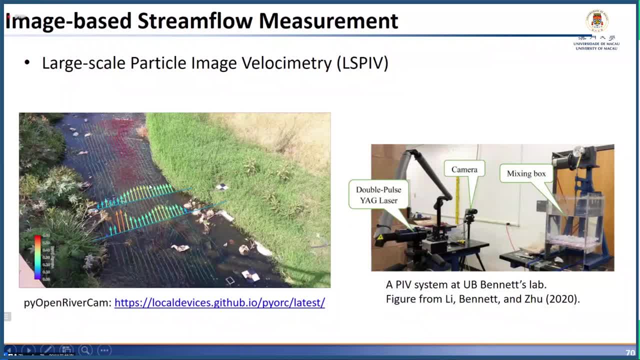 It's quite interesting, although the technique has been already widely used for a long time in the laboratory. So this is a typical PIW system at our lab. It's a very popular university that you can measure flow velocity at a very fine resolution and very good accuracy in a lab scale. However, using a similar 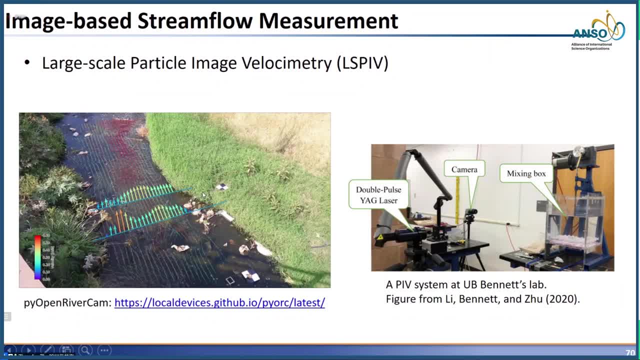 technique at a large scale like this, like on the left, I think this is still a very interesting idea, Seems promising, But it is largely under development. So, if you are interested, this is one example called the PIW Open River, Cam, So you can see what people have been doing. 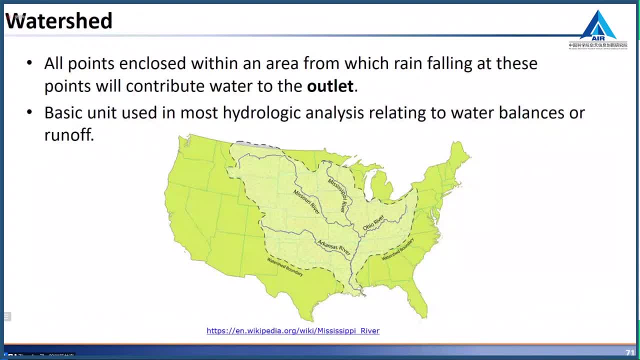 for this. So the watershed- A watershed- is basically all points enclosed within an area, from which rain falling at these points will contribute water to the outlet. So this is a very popular idea of the Mississippi River watershed. So why it's important is because 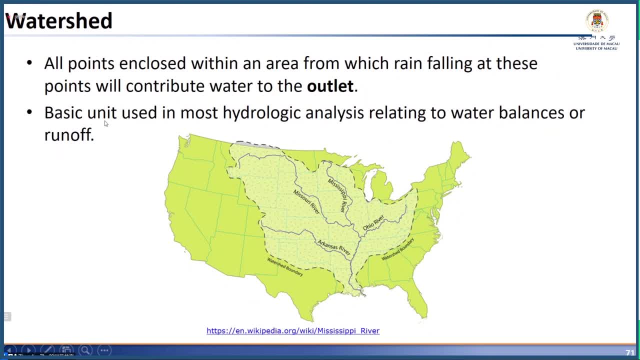 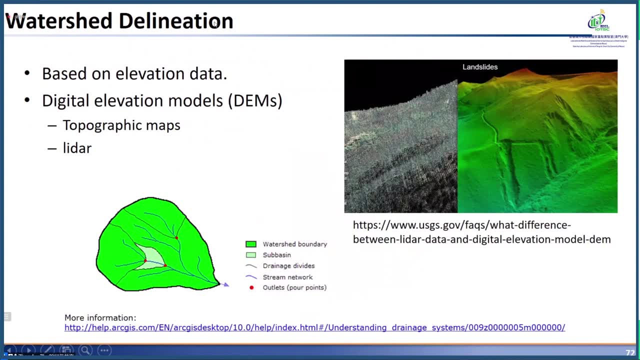 watershed is normally used as a basic unit in most hydrologic analysis, So watershed delineation is based on elevation data. So actually the DEMs, the Digital Elevation Models, can be used to either manually or automatically delineate watersheds. So I think this might be very familiar to most of you. So the DEMs can. 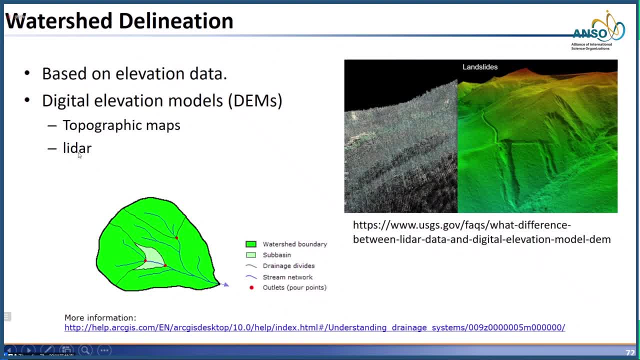 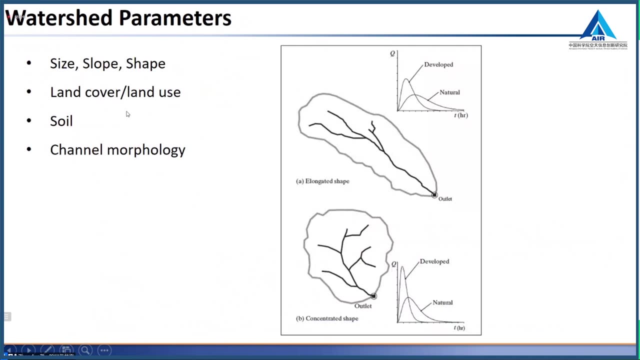 come from topographic maps and or also from ladder right. So this is an example of ladder Okay. So think about the important watershed parameters: the size, the slope, the shape. So once we have the delineated watershed and based on the elevation, it's actually pretty. 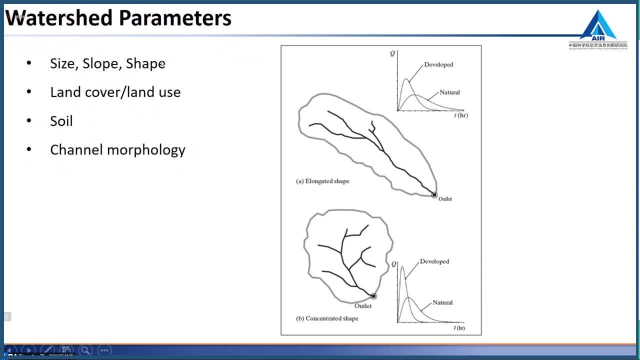 convenient to get those right. The size, slope and shape Land cover, land use is also important for watershed. The soil property is important. Then the channel morphology is also important. Here is just showing an example for two similar areas of watersheds but different shapes. 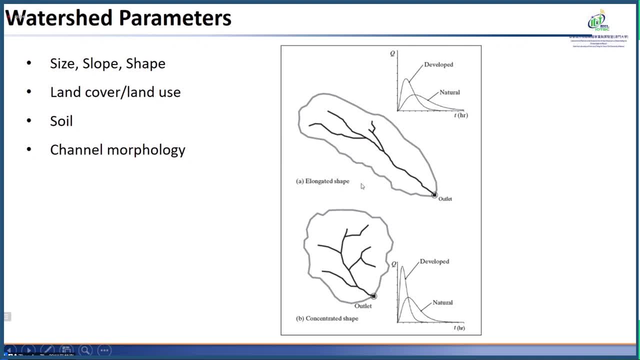 right. So obviously the elongated shape has a longer travel time, right, And this concentrated shape has a shorter travel time. So under the same rainfall event, these ones the peak discharge will come earlier, right, And also expected to be higher than this one. 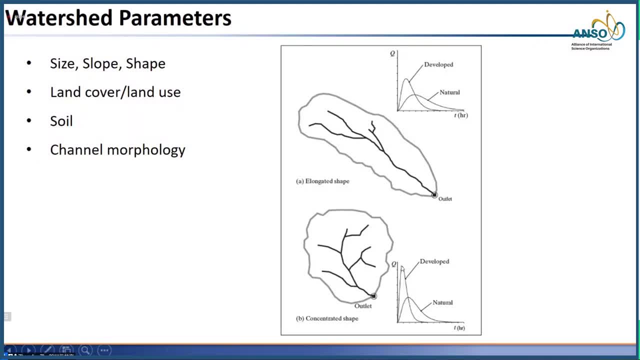 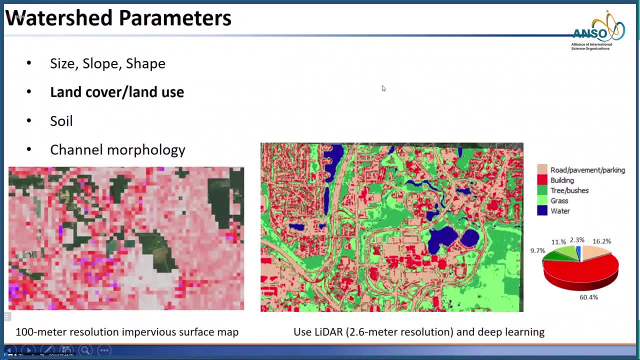 right And also between the natural and the developed. the peak flow is expected to come earlier and higher right. So land cover, land use obviously is also a big application of remote sensing right. So here I'm showing again just two examples. One is a: 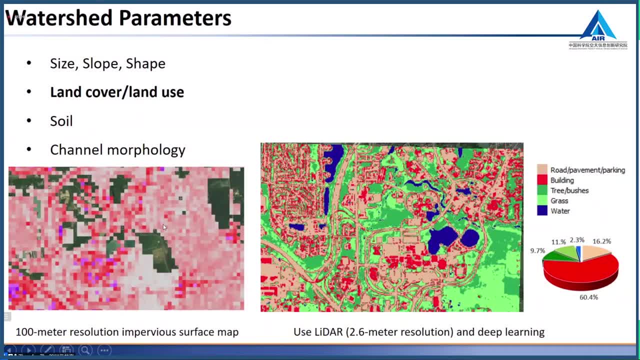 satellite-based DEM, DEM, And this is a 40 meter or 100 meter resolution for impervious. This is given by USGS. This is something we did at our research group- that you can actually use LIDAR data with 2.6 meter resolution And, as you can see, like this, land cover, land use classification. 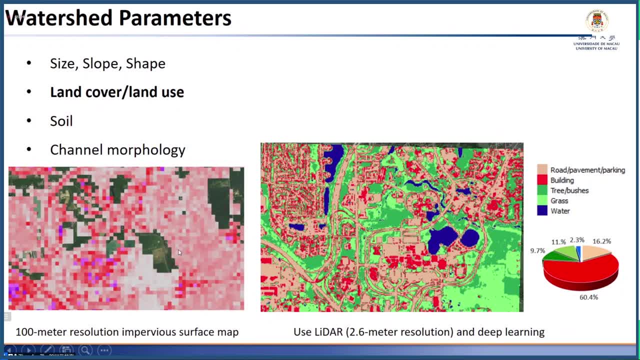 obviously the resolution is much better than this one. Obviously the resolution is much better than this one. So in the SPO you can see you also might have a little bit of image of the pretty largezena Glendalepti this one. But again, this is just as an example to show how remote sensing can be applied. 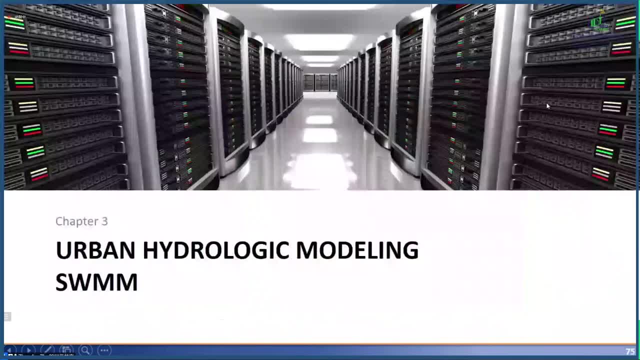 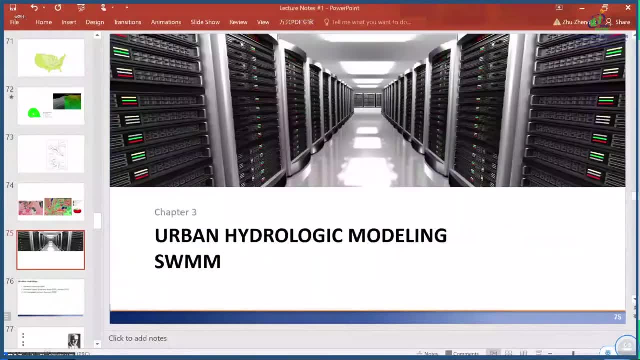 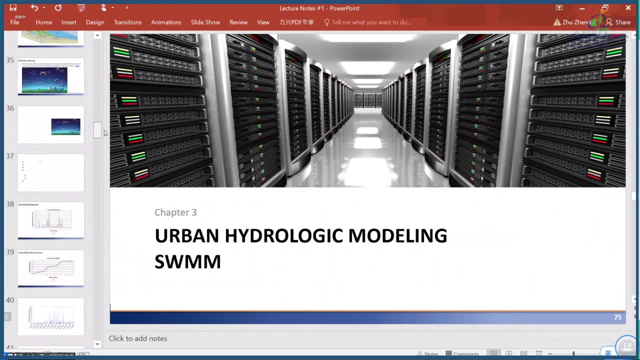 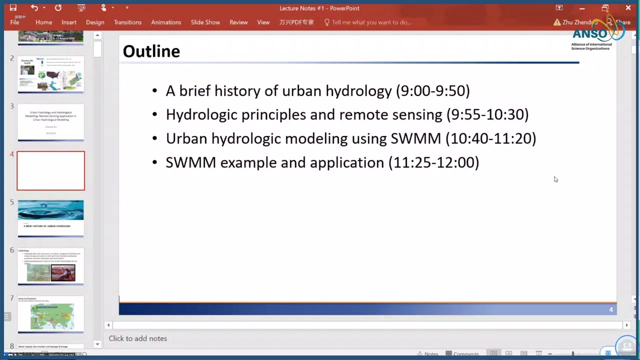 for this kind of knowledge. Okay, So hopefully let me see what time we are: 10.30.. All right, So we think successfully come back to our planned schedule. So let's take a break of 10 minutes, then we'll come back at 10.40.. 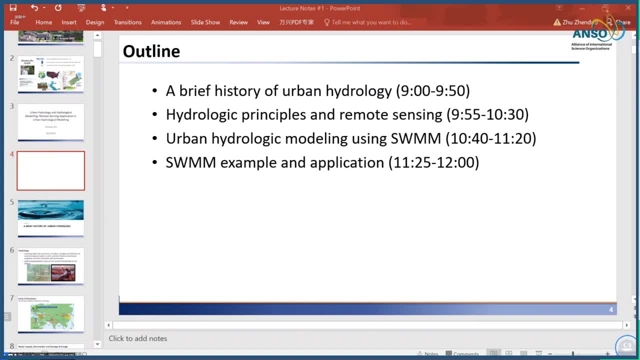 Okay, See, most people are still here. It's good. There's one question in chat asked by Amit Kumar. Thanks for the question. So how can we determine runoff by remote sensing? So hopefully that question will be answered in this coming chapter, that we can do it. 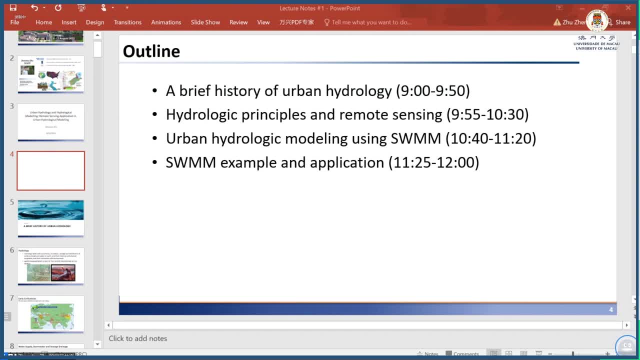 using hydrologic modeling or hydrologic analysis. So let's see. Okay, Let's get started. So this chapter: by the original schedule it will be 40 minutes, But I think it may be. it will maybe like be longer than that, So we will see. 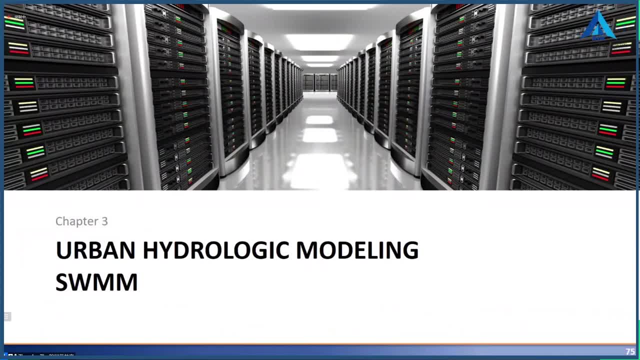 Okay, So chapter three: urban hydrologic modeling, or SWIM. So SWIM will be the modeling package we use to introduce urban hydrologic modeling. I should clarify that SWIM is not the only modeling package And there are other packages that are available, But it's one. SWIM is one of. 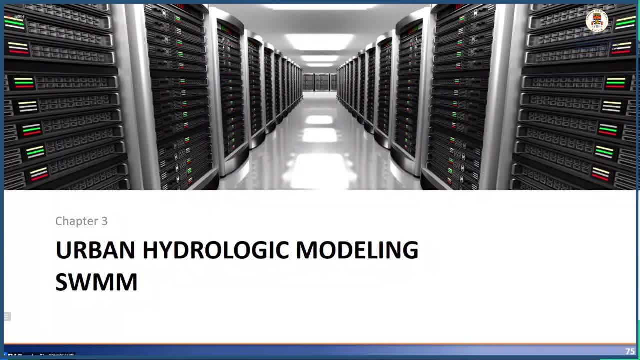 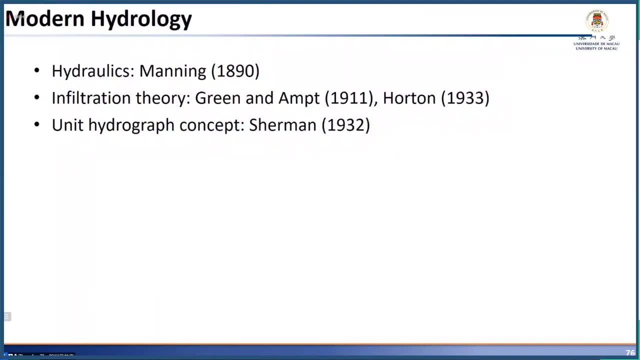 the most widely used urban hydrologic modeling package now? So I'll continue to answer that question. There are many different models that are available. As I said, we're really excited to show you where those models are of this kind Talking about before we go into modeling, I want to just very briefly. 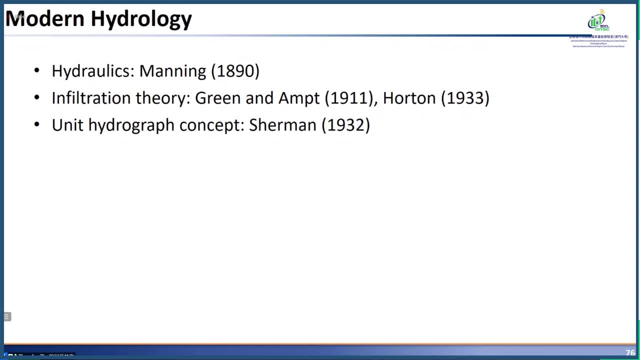 remind everyone, like where we are or where we were in the early 1900s, right. So for hydraulics, you know about early 1900s, the infiltration theory by, you know, Green and Ampt 1911,. 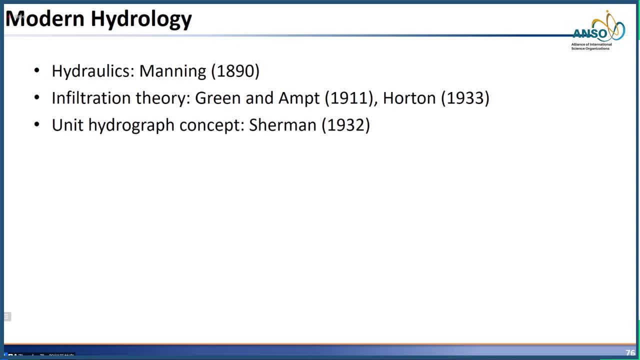 Houghton's formula 1933. And then Sherman also proposed the unit hydrograph concept or unit hydrograph theory in 1932. So until 1930s or 1940s, finally, hydrology became a more quantitative field. that you know, people can actually start to compute, you know. 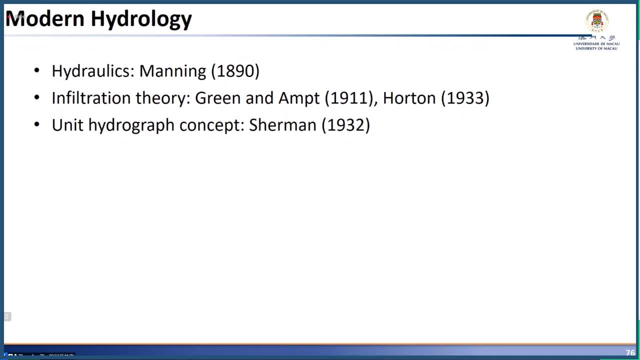 such as runoff like, such as, you know, streamflow right. So basically, the rainfall runoff calculation. you know, we had these tools, we had the theories to do that. However, that's not enough For modeling right, especially what we call model now is referred to as computer modeling. So 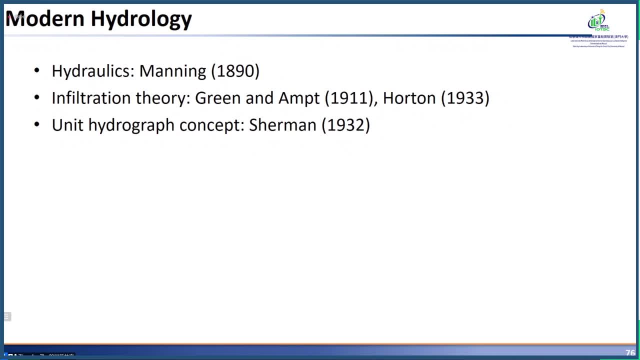 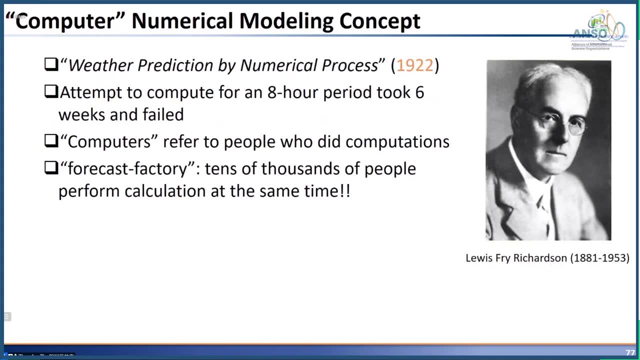 in order to have the first computer model we have to wait until the first computer was invented. However, before that there was very interesting computer numerical modeling concept, proposed as early as 1922, by Lewis Fry Richardson- So he's British- so in his book Weather Prediction by Numerical Process. 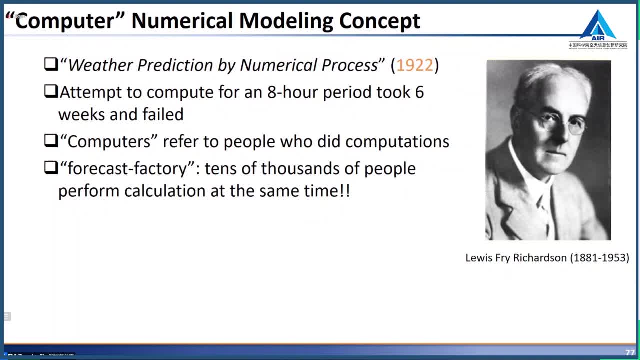 so he proposed, and also he tested his idea by attempting to compute for an eight hour period long of weather calculation for the British, which finally took six weeks and failed. okay, However. so the concept, this numerical process concept, is pretty similar to what we are doing nowadays. 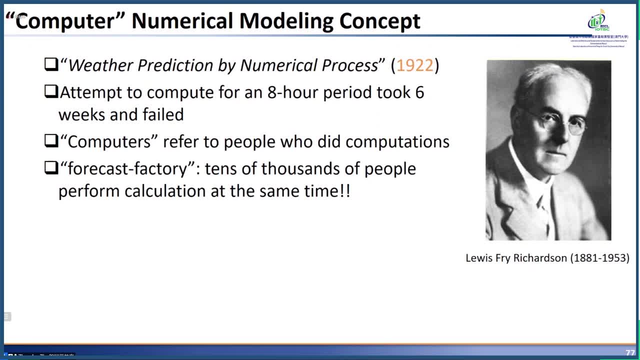 And this is probably one of the most crazy ideas I have heard- that actually worked, of course like later by a different technology, But it finally worked. However, back then Richardson failed And, interestingly, in his book he used the word computers okay, And 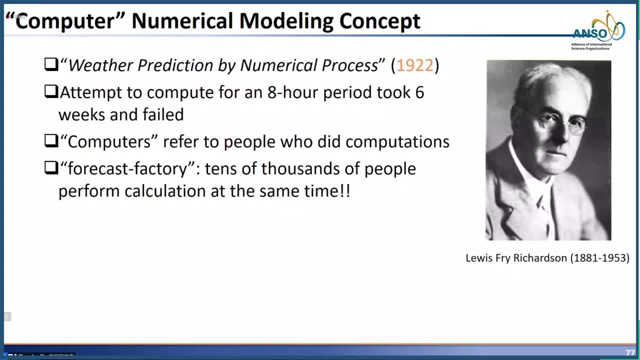 at the time, computers refer to people who did computation, Definitely not the computer we mean right now. And what he proposed? that, although his attempt failed, he believed that if we can build a forecast factory right and hire tens of thousands of people to perform calculations, 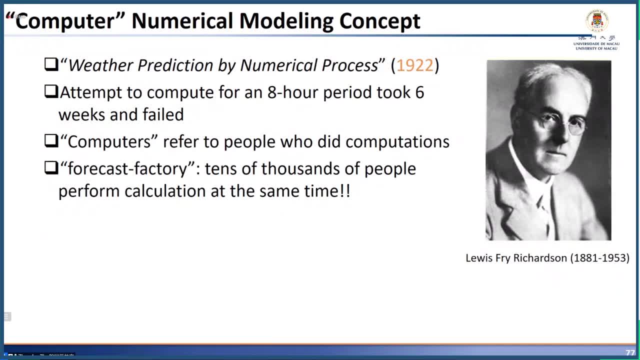 at the same time, he believed that this approach could work. Okay, So again, I think you know, when you read the history of science, we are always surprising stories, and I hope these can be inspiring as well. Alright, that's also an interesting topic. 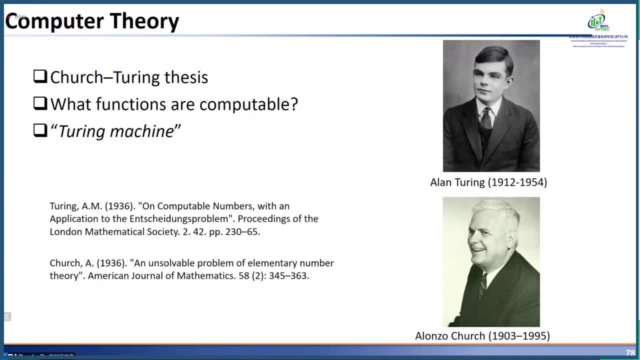 Are there any more questions for people or comments, Or is there a small question Don't like to answer? Okay, One more question from films. We haven't seen the는데요, I think for the whole台 until 1930s. So obviously in 1920s Richardson couldn't do what we are doing now, because 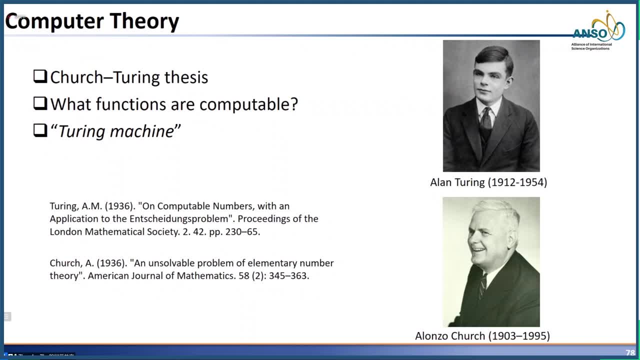 even the computer theory came in 1930s, independently by Alonzo Church and Alan Turing, So this is called the Church-Turing. this is more often referred to as the Turing machine. So Alan Turing and Alonzo Church were trying to answer a question that what mathematical? 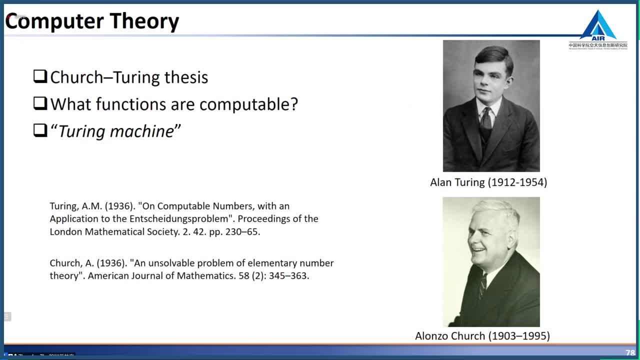 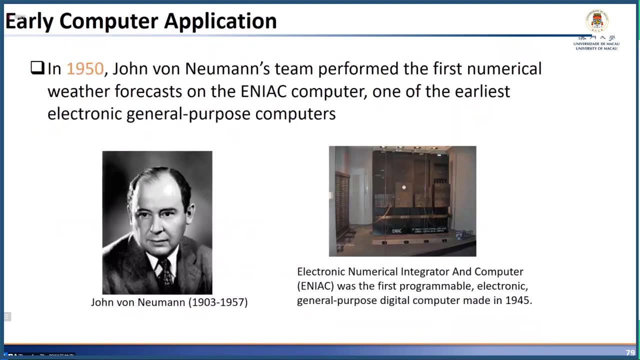 functions are actually computable. And in order to answer this question they actually built up the foundation of the modern computer theory. Of course, the first modern computer didn't come out until actually 1940s, So in 1950, another important man, von Neumann, so his team, performed the first numerical weather. 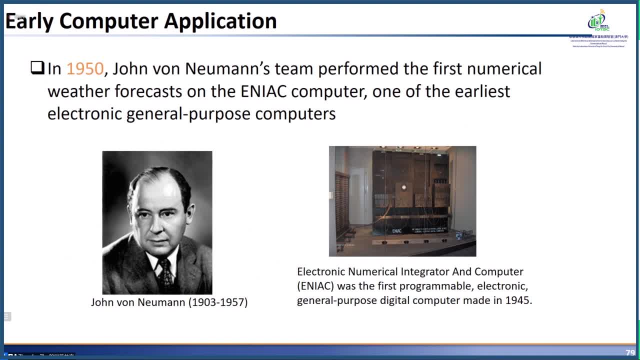 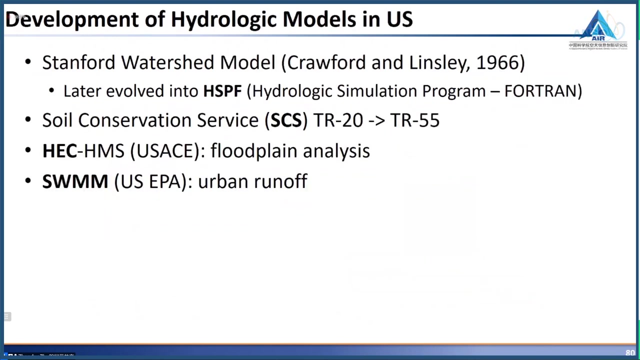 forecast on the ENIAC computer, So, which is one of the earliest electronic general purpose computers, And finally proved that the concept by Richardson- 1922, actually could work, but not with human computers, but with electronic computers. Then later, in 1960s, computers became more accessible to researchers, Although it's 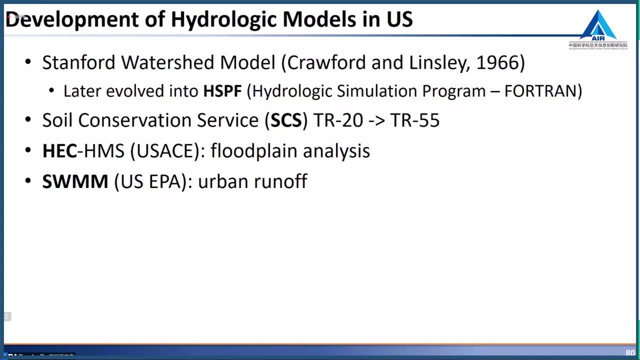 not that accessible to the public, but it at least became accessible to research institutes or universities such as Stanford. In the 1960s, Crawford and Lindsley developed the Stanford watershed model, So this is one of the earliest hydrologic models. And, by the way, here I'm only 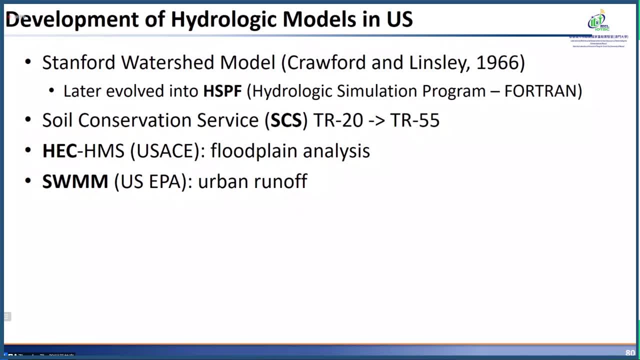 focusing on this history, the development of hydrologic models in the United States. So they are actually, of course, like in Europe, in Asia, different countries. they are also development as well. So then later, there is the Soil Conservation Service, SCS. they developed a method called TR20, which later evolved into TR55. 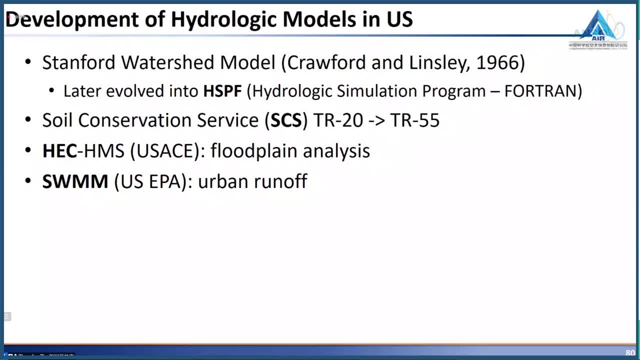 Then US Army Corps of Engineers developed the model HEC. This is a family of models and one of the family members, HEC-HMS, is widely used for floodplain analysis. Then the US EPA lead this development of SWIM, which we will focus on today. that is designed for calculating urban runoff. 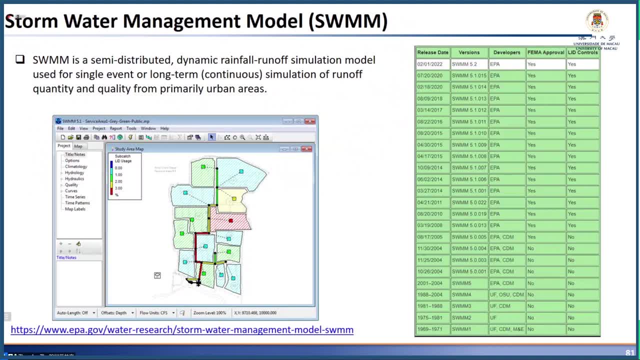 So SWIM is short for Stormwater Management Model, So SWIM. this is a semi-distributed dynamic rainfall runoff simulation model. It can be used for single event or long-term simulation. So the first version was again developed by the US Army Corps of Engineers and the US Army Corps of Engineers. 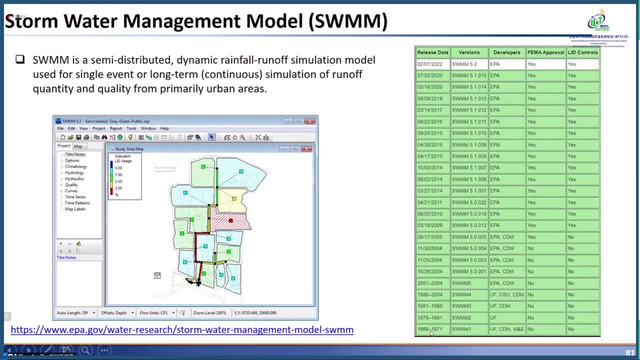 Then the second version was developed in 1960s, so late 1960s, early 1970s- But since then it has been evolved and improved a lot. So the most recent version is 5.2.. And I believe the most recent update is actually 5.2.1,, which was updated in this month, August 2022. 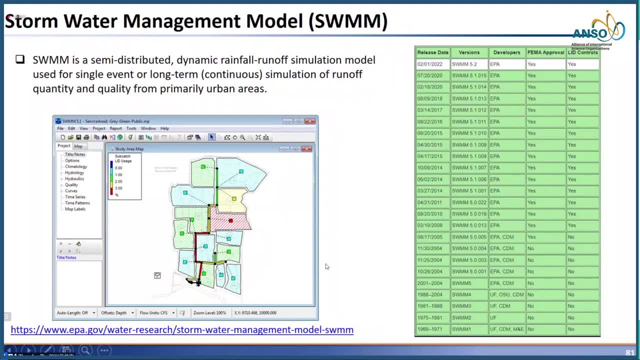 So here is a graphical user interface. It has our first's and most recent functions. So here, read on. so let's read the representation of this model. So this is a model in package and if you are interested you can go to this website. 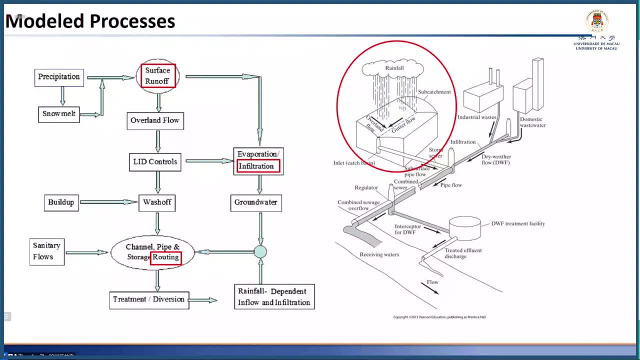 It's a very good user reference user menu and then very good reference menu. So of course we don't have enough time to go over all details. precipitation: if it's rainfall then you know it goes to surface runoff directly. 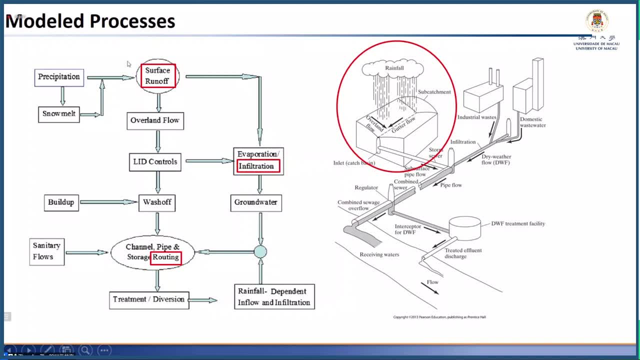 If it's snow, there is a snowmelt process, then it goes to surface runoff, Then surface runoff gives overland flow, then also evaporation, infiltration, groundwater channel routing and so on. Okay, So we today will only focus on three parts, because I think the others 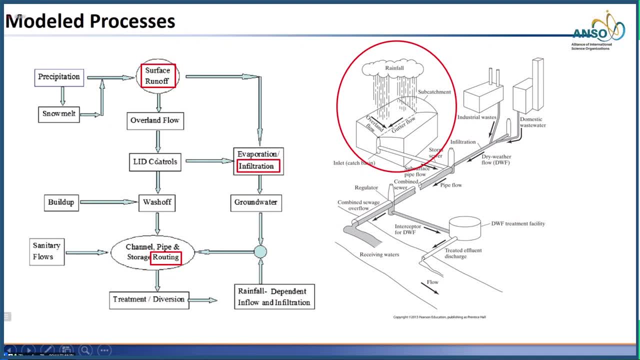 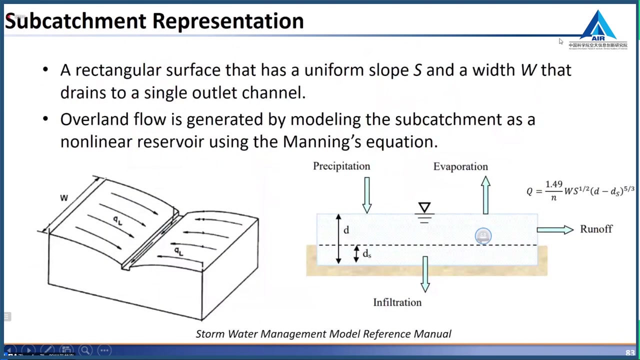 are either like, more water quality oriented or the LID control. we will talk more tomorrow And, yeah, the other processes, I think, are more straightforward. Okay, So let's look at how surface runoff was calculated. Okay, So, first, subcatchment is represented in SWiM at a rectangular surface which looks 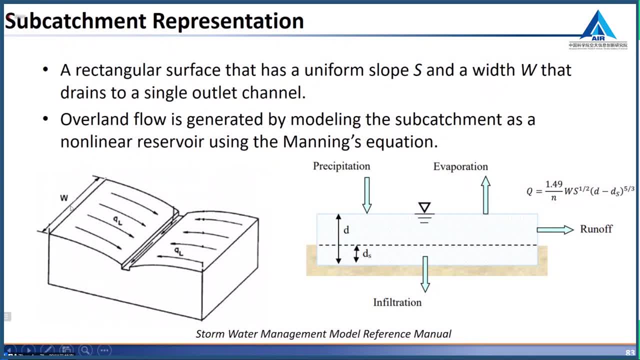 like this: There is a uniform width, uniform slope, and then it turns to single outlet, channelала q. So this is one subcatchment in SWiM. So basically, the overland flow is generated by modeling the subcatchment as a non-Trade. 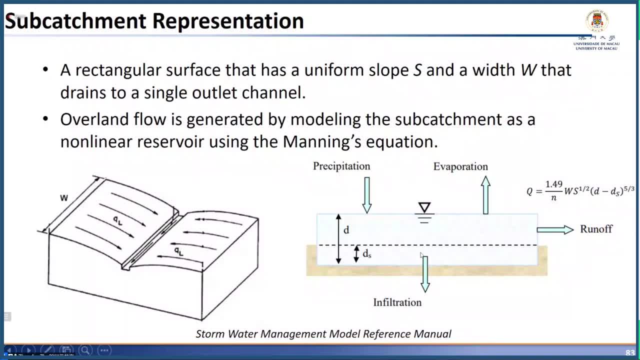 curve as a nonlinear reservoir. So here, as you can see, the whole watershed is considered as this reservoir with storage. This is a depression storage. Then when it's higher than the depression storage, then it can start to generate runoff right. 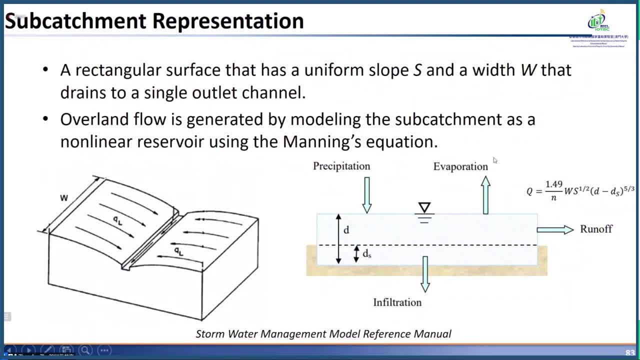 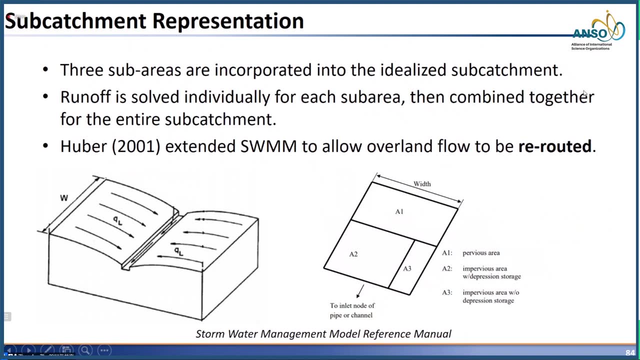 And obviously the input is precipitation, then there can be evaporation loss, Then the runoff is actually calculated using Manning's equation. right So here? width, slope and delta H, right So the conceptual model in SWIM actually divides the one subcatchment into three subareas. 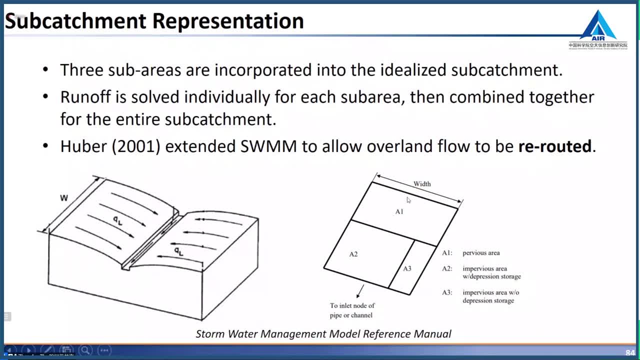 So those are A1, which is a pervious area, and A2, which is an impervious area with depression storage, and there can also be impervious area without depression storage. okay, So I should clarify. you don't have to have all of the three subareas, right? 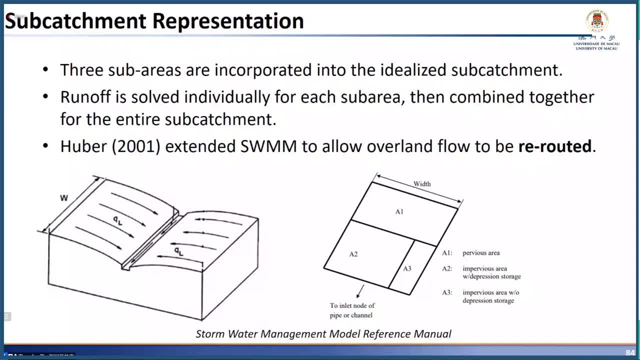 So, for example, one subcatchment can be 100% pervious or 100% impervious, Or even with separation of pervious and impervious, you can have two impervious areas, with or without depression storage. You can also have only impervious area with depression storage or without depression storage. 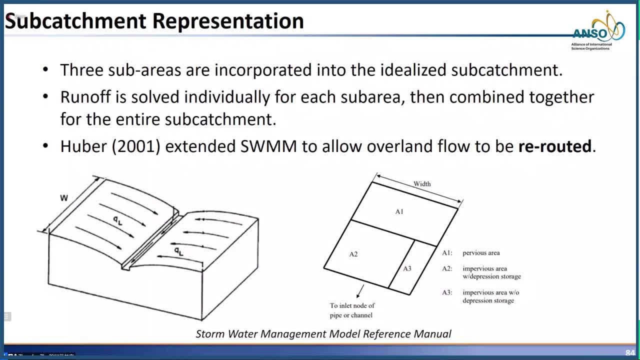 So there are different options there. So the runoff is solved individually for each sub-area, then combined together for the entire sub-calculation. So that's the original runoff calculation. So later in early 2000,, Huber extended SWIM to allow overland flow to be rerouted. 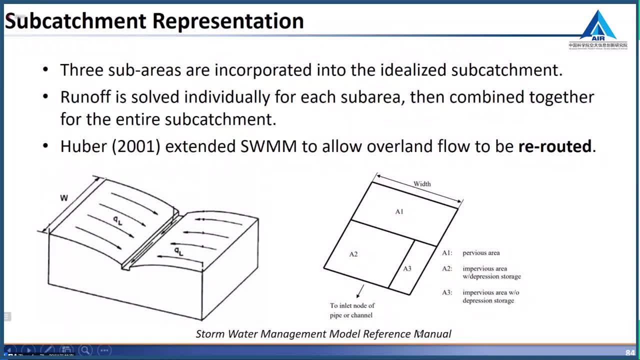 By rerouted it means the runoff or overland flow from A1 can go to A2 before going to the inlet node of the pipe or channel, or it can go to A3 before going to the inlet node And also the overland flow from one sub-calculation can first route into another sub-calculation. 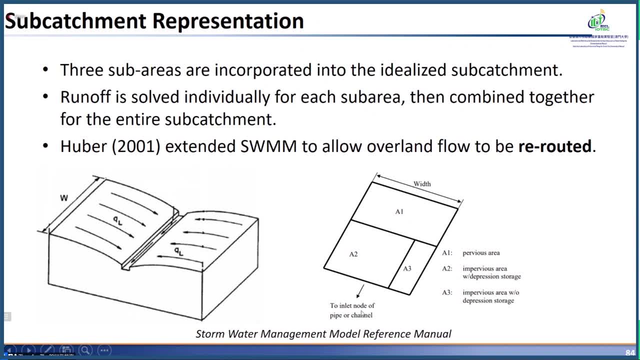 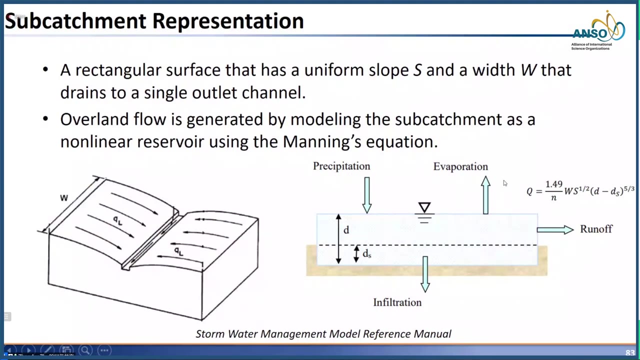 Then from another sub-calculation it goes to a node or channel. So that's what it means by rerouting or rerouting, So infiltration, as you can see here, that precipitation and evaporation we have talked about, so those can be measured and those can be input into the model. 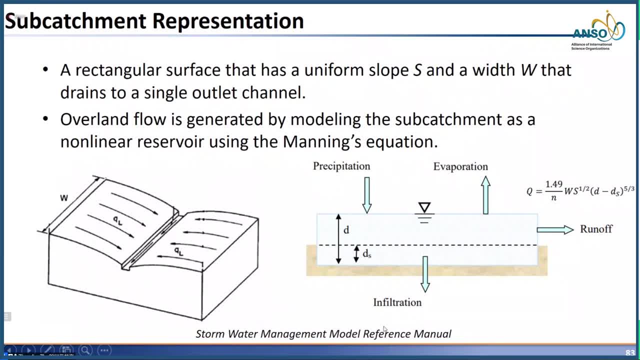 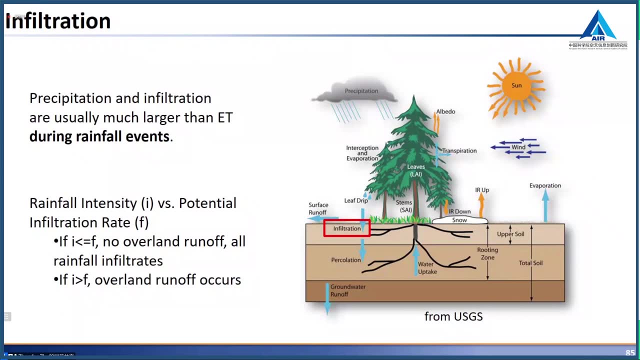 And the runoff can be calculated based on that. But one thing, One more thing we need to calculate is infiltration. So how much water can actually infiltrate? So that has to be modeled as well. So, by the way, precipitation and infiltration are usually much larger than evaporation or 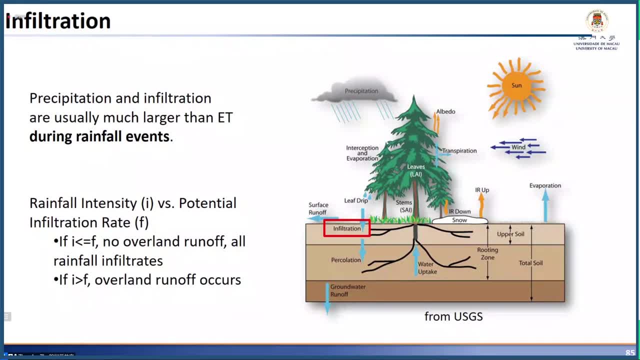 evapotranspiration during rainfall events. So that's again: infiltration is very important for calculating runoff. So during rainfall events you could neglect evaporation, evapotranspiration, but you cannot neglect infiltration. So if you consider the rainfall intensity versus the potential infiltration rate, 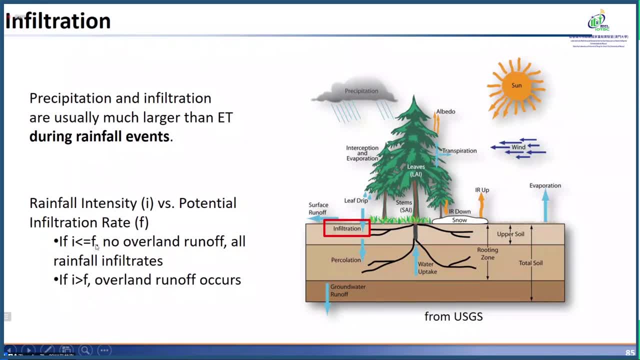 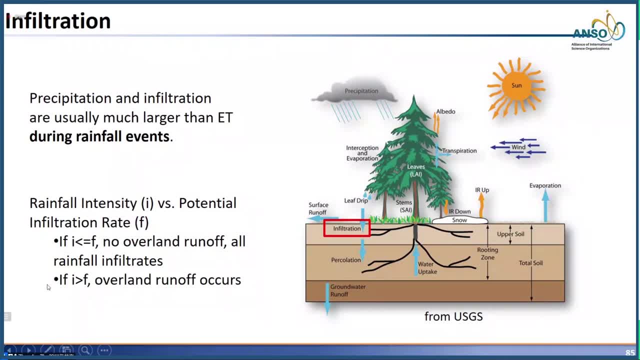 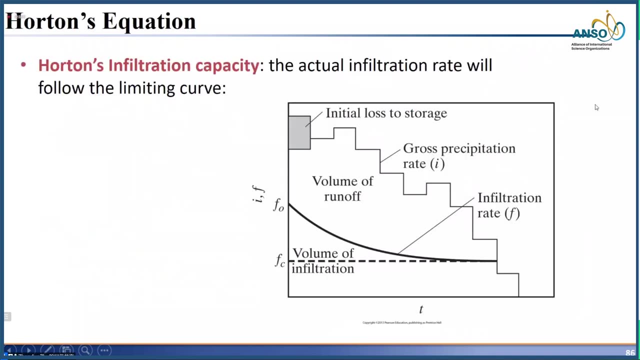 Right Or no runoff, Because all rainfall can infiltrate. So only if the rainfall intensity i is larger than the potential infiltration rate f, then the overland runoff or surface runoff can happen. So for calculating infiltration rate we will introduce the two most widely used methods. 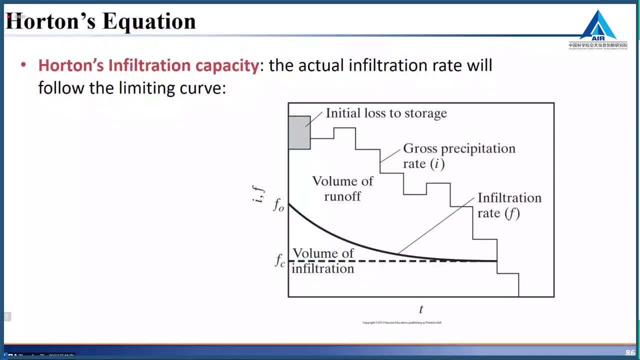 Right. One is Houghton method, The other is Green-Apt, So Houghton's equation is an empirical formula. So basically, Houghton proposed that the infiltration capacity is actually follow the limiting curve, which basically decays exponentially from F0, which is the initial infiltration rate, to 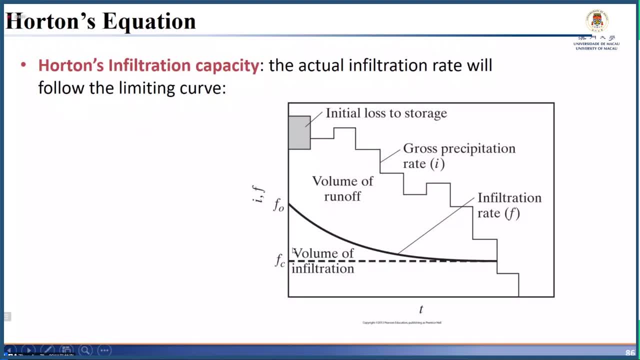 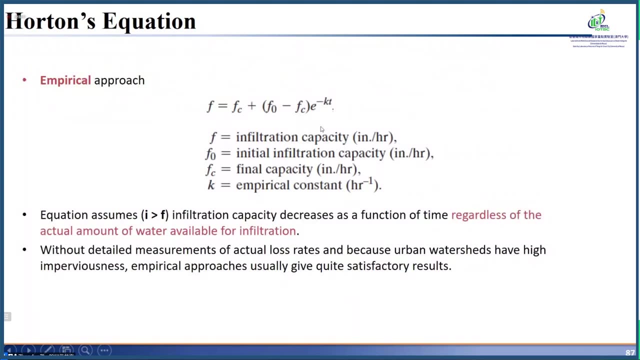 the Fc, which is equilibrium, Right infiltration rate, And between f0 and fc. this is proposed as an exponential function of decay. So the function or formula looks like this: f equal to fc plus f0, minus fc times the exponential function which decays. So basically there are three parameters here: fc, f0, and k. 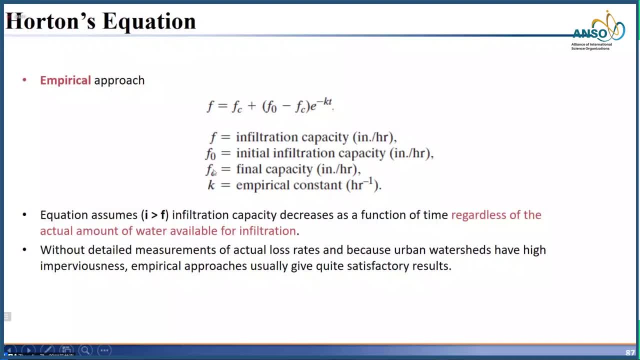 So f0 is the initial infiltration capacity, fc is the final capacity and k is an empirical constant. So this equation or this method has some assumptions, and one of the assumptions is it assumes I is larger than f, Or it assumes like 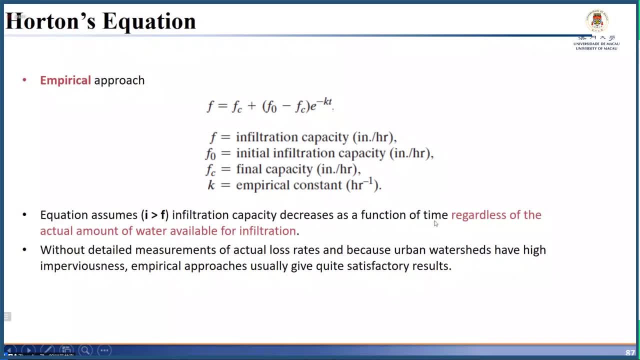 you know, this infiltration capacity decreases as a function of time, regardless of the extra amount of water available for infiltration. So, in other words, it assumes that there is always water pounding on the surface of the soil. So this assumption can be corrected or can be modified by considering: 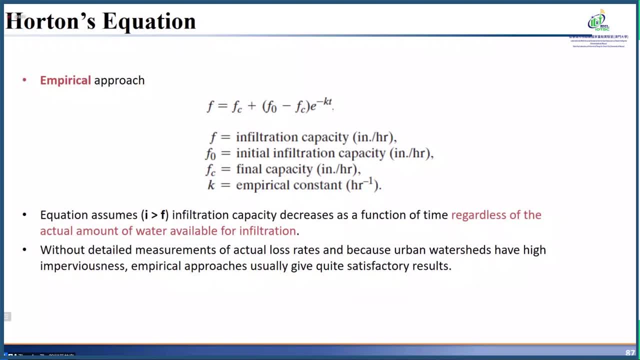 an initial loss. So before applying Holden's equation, you could first apply an initial loss. By initial loss, you basically take consideration of this, you know, before or pre-pounding period, and then after that you can apply Holden, which is after pounding. 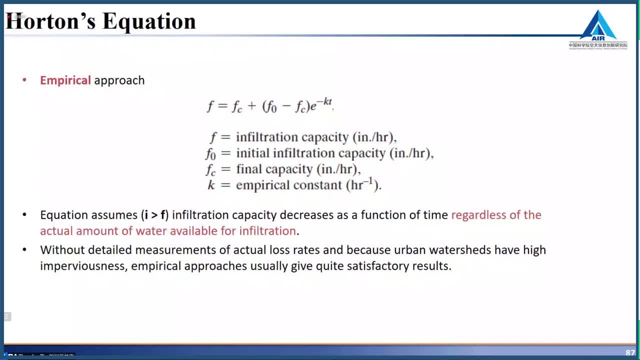 Okay, a big difference. when you see green-empt, you will see that green-empt actually can deal with pounding by itself without that correction or modification. So, given that said, because they are normally not very detailed measurements of actual loss rate and also the urban watersheds, 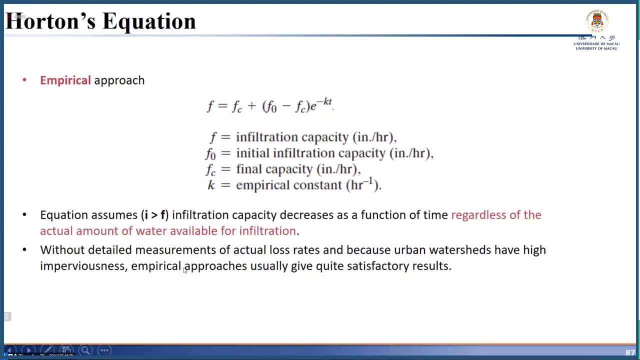 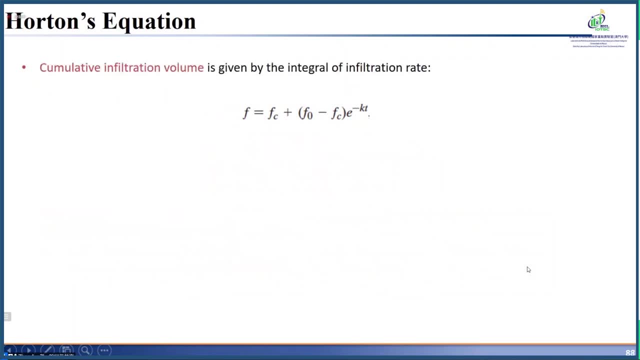 have high imperviousness. so this empirical approach usually gives quite satisfactory results. That's also why it is so commonly used. So there are some calculations you could do, For example the cumulative infiltration volume. that will be the integral of infiltration. 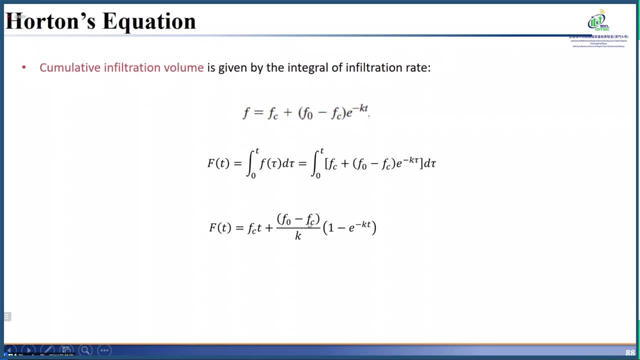 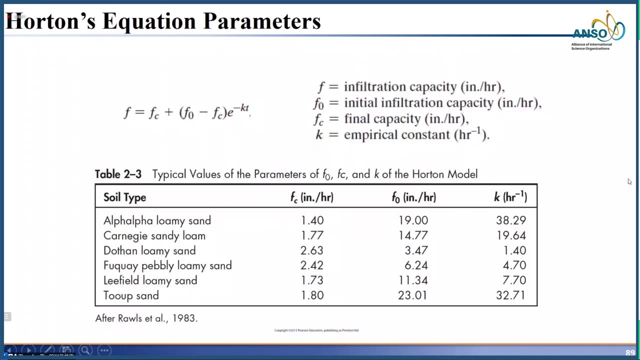 rate. So, for this example, this is our capital F. that will be a function of this. Why we want this? Because, again, when you compare it to green-empt, green-empt actually is a function for capital F instead of infiltration rate F. 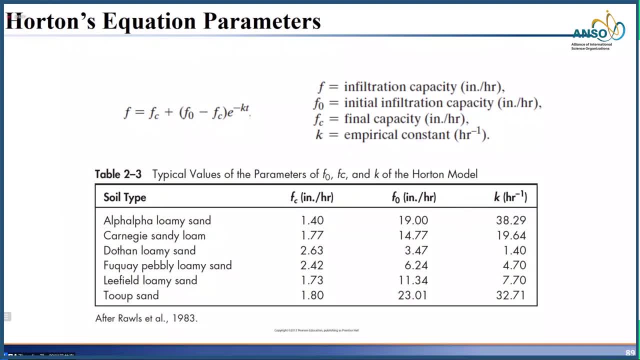 So for the three parameters, depending on different soil types, these three parameters will be different. So Ross in 1983, has summarized this and suggested those values for different soil types. However, in hydrologic modeling, keep in mind those are or could be considered as a 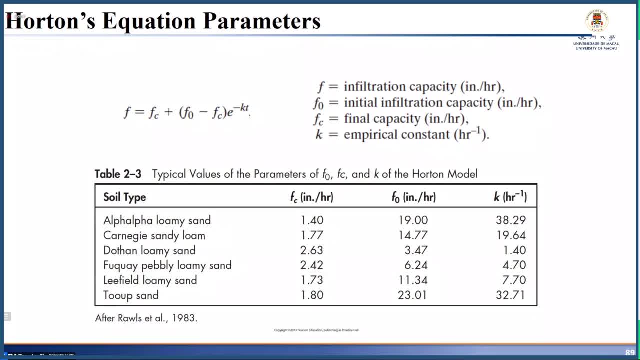 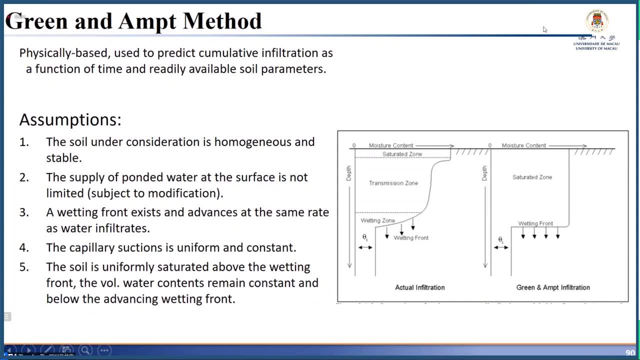 calibration parameter. What does it mean by calibration? we will introduce later. Okay, so Green Ampter method is the other widely used method for infiltration. So, different from Houghton, Houghton is an empirical approach. Green Ampter is actually a physically based. 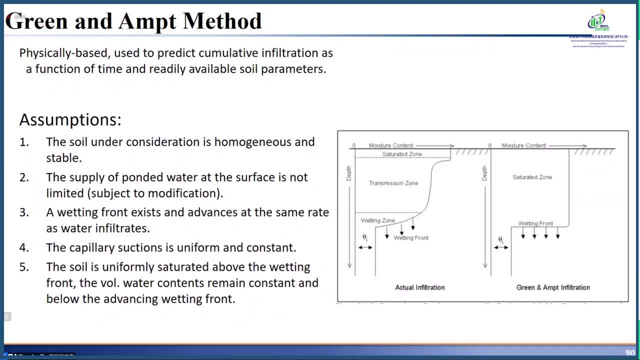 approach. It's based on the Darcy's law. Of course, it takes a lot of assumptions, And one of the biggest assumptions is that it assumes there is a wetting front And above the wetting front there is a perfectly saturated zone, And then below the wetting front then there is just initial 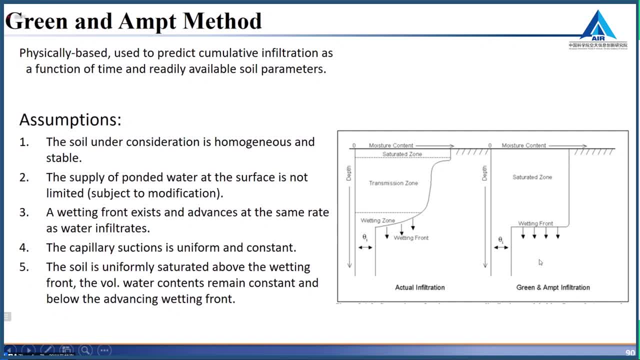 moisture, basically without any infiltration. Obviously, this is different from reality, right? So the actual infiltration: there is a saturated zone, but between the saturated and not being affected there are actually a large area of transmission zone. So, as you can see, 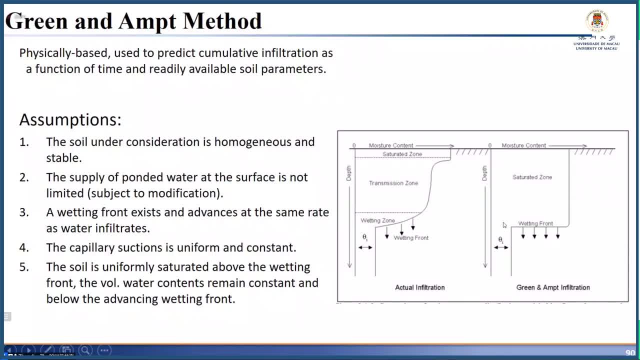 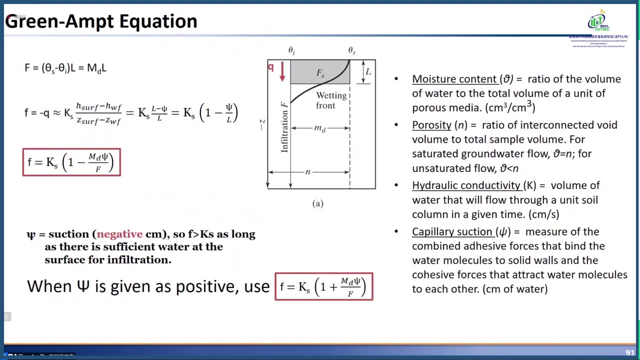 like those are not really clearly horizontal wetting front like this. However, based on this assumption, so Green Ampter could derive a formula for calculating infiltration rate. So for the time being, I think I will just simply introduce the idea. So, basically, 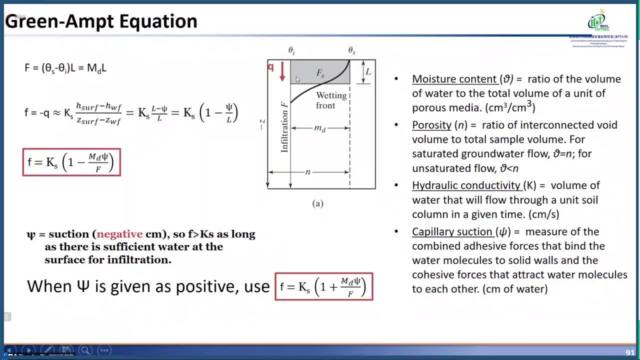 if you think about the water volume or the total infiltration in the soil, right capital F. so that's the difference between the saturated moisture minus the initial moisture, then times the depth of this. So basically this is the wetting front right. So theta S minus theta I. 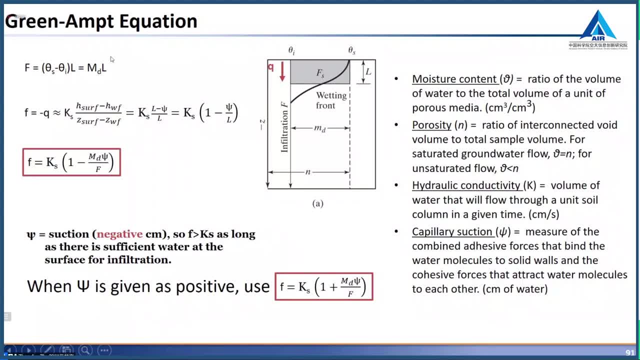 can be noted as MD right. So this is MD times L, And the infiltration rate or the rate the velocity of the wetting front right depends on, basically, the infiltration rate right, And here it's assumed that the infiltration rate can be calculated by Darcy's law. 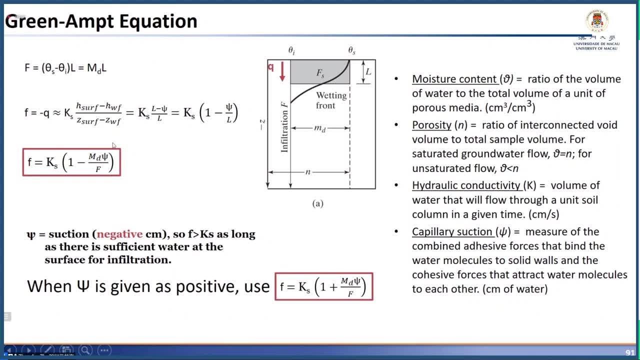 right, Which is delta H over. so this is KS times the difference in water head minus, so basically the gradient of the water head right. So then this becomes KS times Y minus phi over L, And then you know, basically this became. 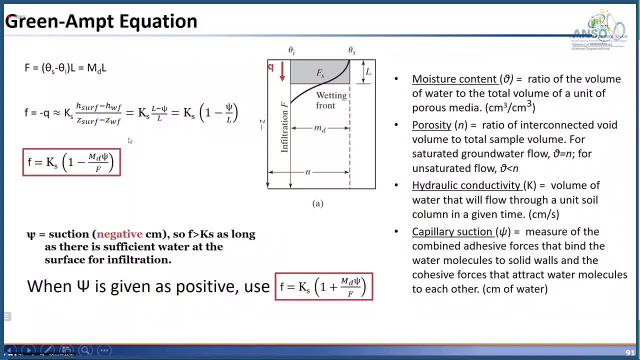 greater than F, as Kann 4 saying this formula right And it's in the green amp formula right. So, as you can see, green amp does not give infiltration rate or infiltration volume explicitly, but it actually gives a relationship between F and KF. however, 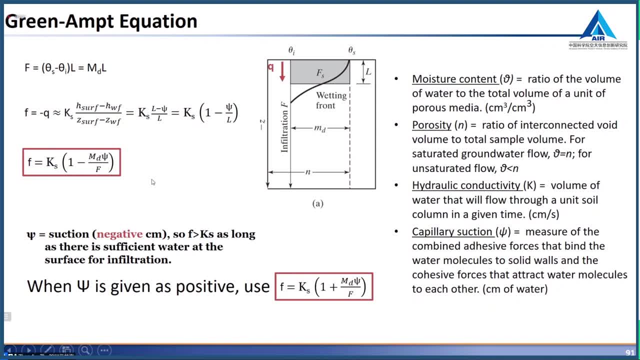 based on the relationship, it is not difficult to get either F or F Okay. Unknown Speakerev. 00 00 00 00 Laszlo Ogo 01 Sonano, 01 Soldino. 00 00 04. Unknown Speakerev. 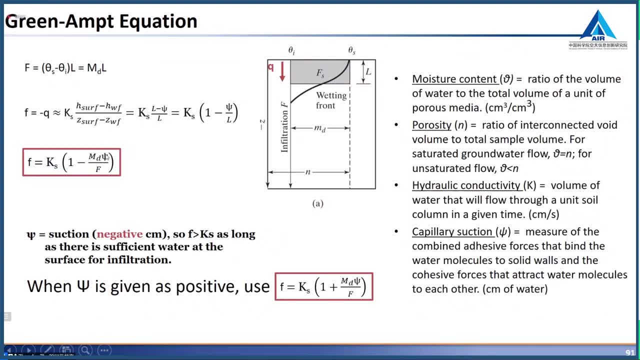 02 Sonano 01 Demo 01 Samadll 02 Malo. note is this: Phi, which is the capillary section, should be a negative value. In some cases you may find in literature or other resources that Phi is given as a positive value. So 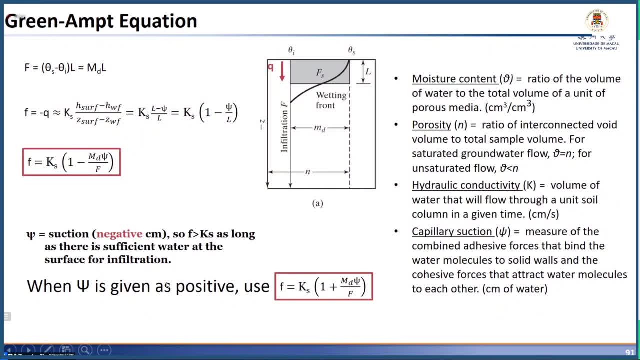 in that case you either have to change it to be negative or you use the plus instead of a minus if Phi is a positive value. So basically, the calculation of F: because Phi is a negative value, MD is positive, F is positive, so this is a negative value, Y minus. 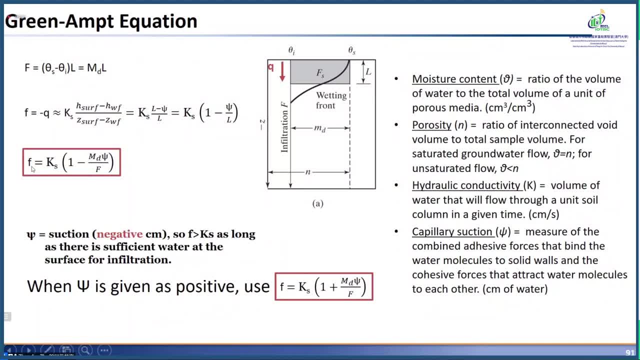 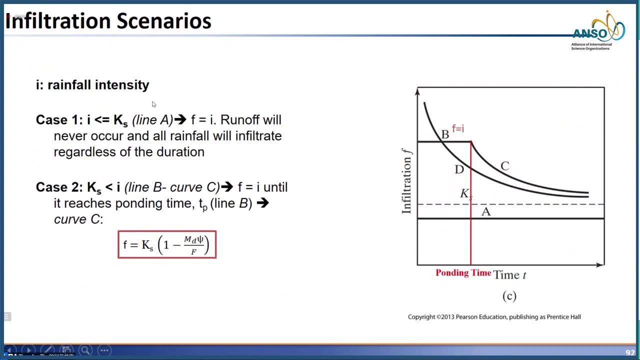 negative value is larger than Y, So F should be always larger than X And KS is the hydraulic connectivity. So there are different infiltration scenarios when you apply Green Amp. So first case is if the rainfall intensity is even smaller or equal to hydraulic connectivity. obviously all of the rainfall can infiltrate, So infiltration. 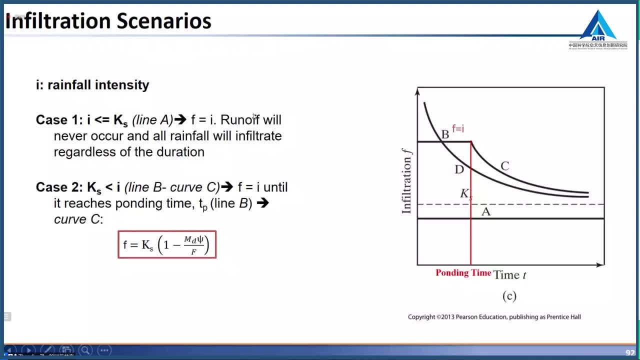 rate simply equals to rainfall intensity and there will be no runoff. And then when the rainfall intensity is larger than KS, larger than hydraulic connectivity. so, as you can see from the formula, if you calculate F based on this formula, when capital F is very small, close to zero, then F actually goes to infinity. So again, which means based 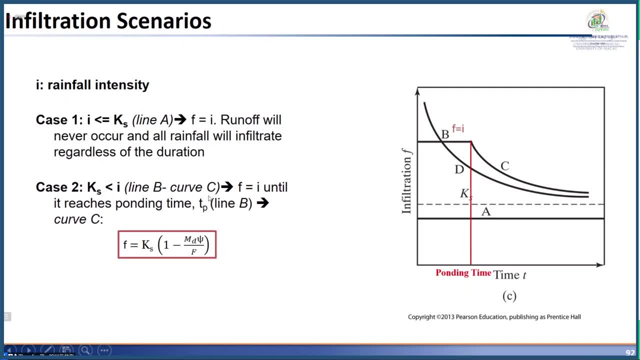 on Green Amp method or based on the assumptions in Green Amp method at the very beginning of the time. so there is always that the potential infiltration capacity can be larger than the rainfall intensity. So then F equals to Y until it reaches what is called the pounding time. So then after: 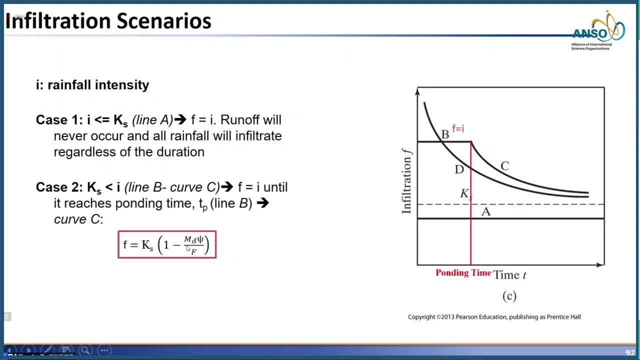 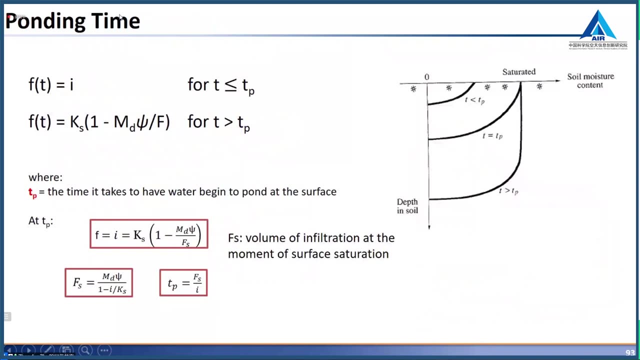 the pounding time it starts to follow this formula: Okay, Okay, So first is the horizontal line B and then decay as curve C. So how do we determine pounding time here? So, because we know at the pounding time first F equal to I and then F also. 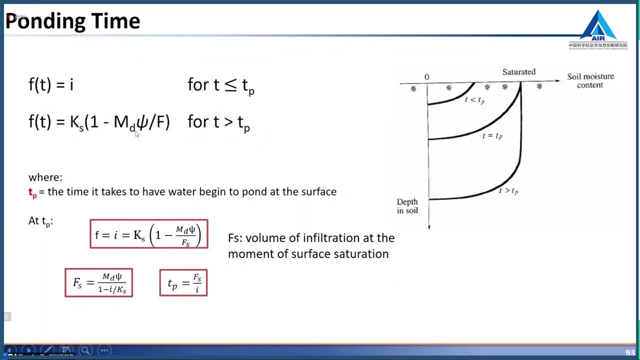 equals to the Green Amp formula, right? So then, basically, I equals to this. So then, based on that, you can calculate F3.. Okay, So this is F sub S, which is the volume of infiltration at the moment of surface saturation. 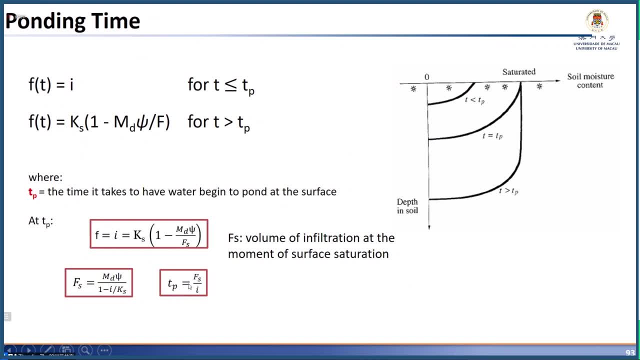 or at the moment of a pounding, Then TP equals to capital F sub S divided by rainfall intensity. right, So this is the pounding time, This is the volume of infiltration at pounding time. So, again, if you go back to this, as you can imagine when you compare this with: 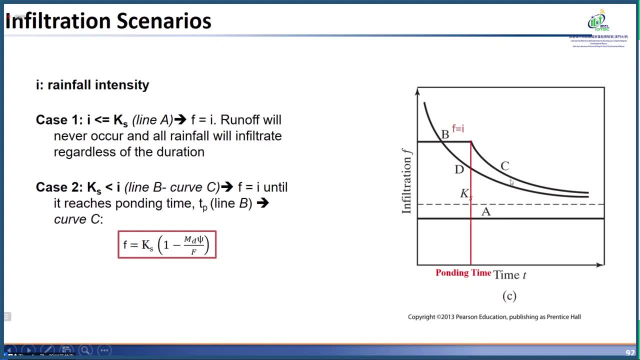 Houghton. right, so Houghton is always a decay function, right, So Houghton is always decay. Again, that is because in Houghton it assumes that there's always pounding water. Okay, But if you apply Green Amp to actually, it will first need to reach the pounding time. 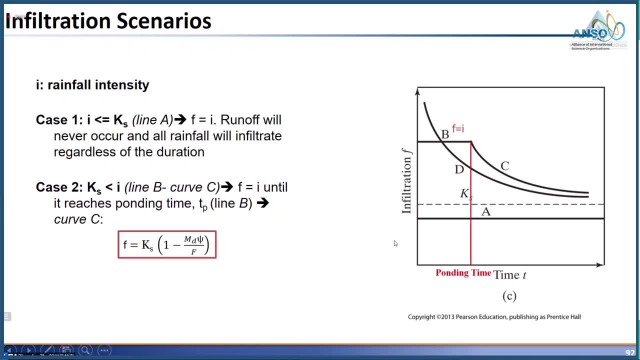 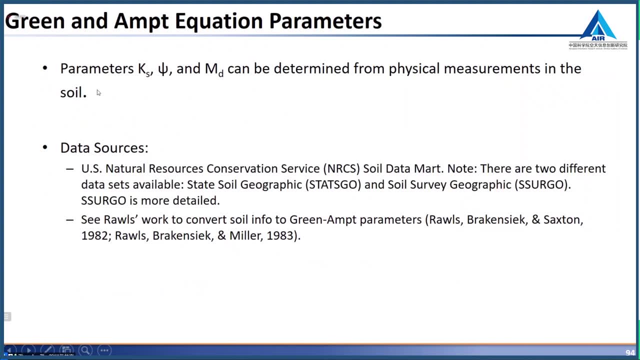 then it follows a decay. Okay, So in Green Amp there are also three parameters right, The same as Houghton. However, those parameters all have physical meanings So theoretically it can be determined from physical measurements And those are all soil related physical properties. So actually these can. 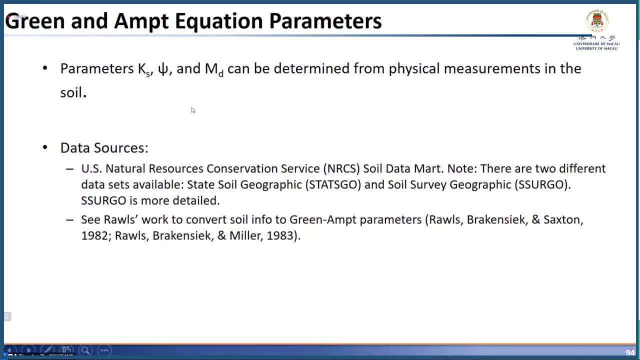 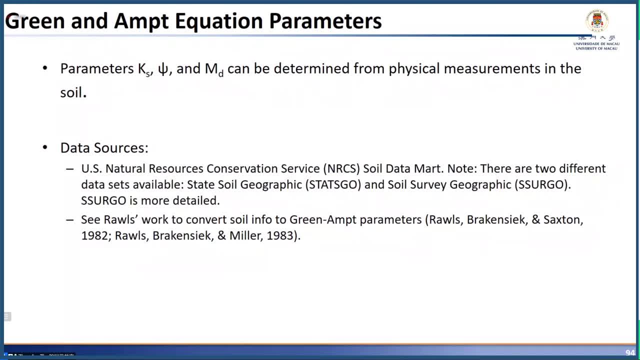 you can see that the parameters are not always the same. So you can see that the parameters are not always the same. So you can see that the parameters are not always the same, And the reason for that is because Green Amp method is derived based on those important 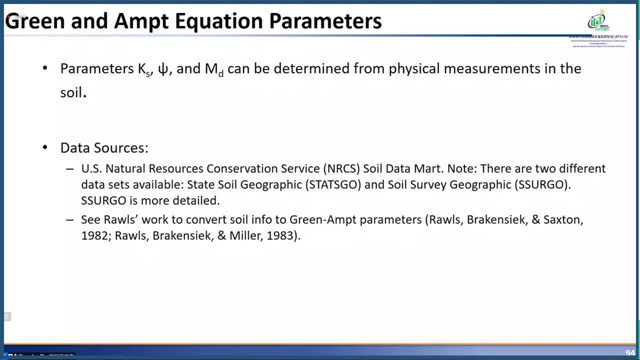 assumptions. So directly measuring the parameters do not necessarily mean that your model will be perfect, right, So you could have perfect physical parameters by measurement, but those cannot guarantee that your model will be good as well. well, You know what I mean, because there are assumptions in the model. 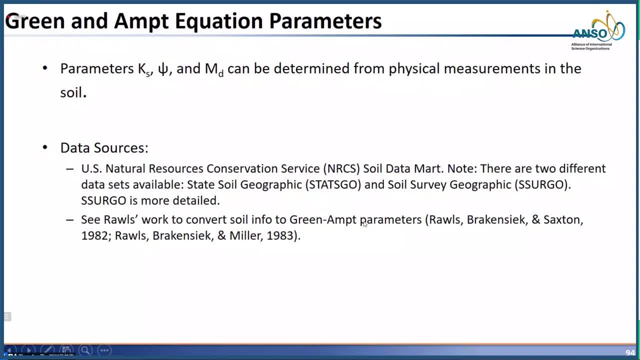 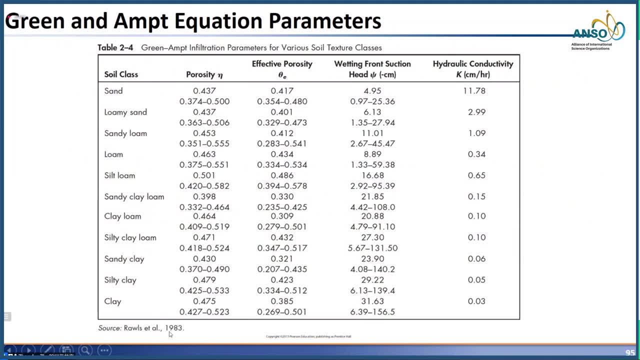 So to find the parameters, there are different data sources here. only giving you one example Again, it's based on the work of Royce in 1983.. So depending on the different soil type, I can have different values of the parameters. 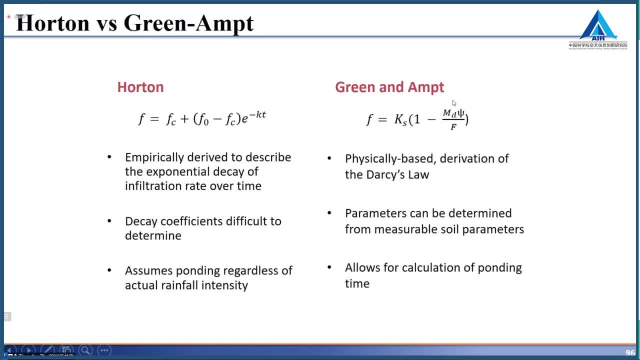 So if you look at Houghton and Green Ampt side by side, one is empirical formula, the other one is physically based. One like the decay coefficient in Houghton is difficult to determine. Then, Green Ampt, the parameters can be determined from directly. 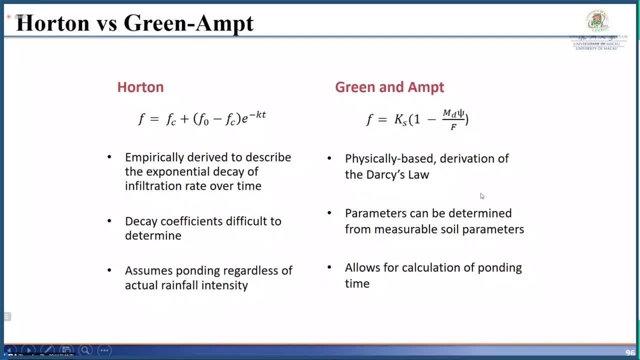 measured soil parameters. But again, keep in mind those measurements are subject to calibration. So then Houghton assumes pounding regardless of actual rainfall intensity, and Green Ampt allows for calculation over pounding time. Again, Houghton, by a correction or modification, it can address this assumption of pounding. 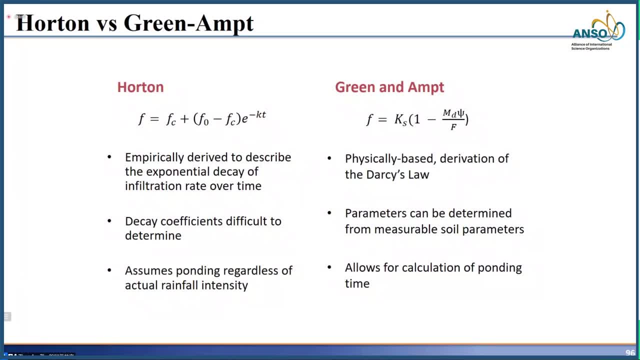 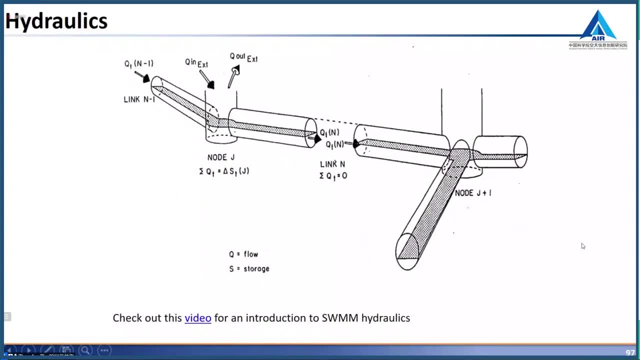 at least to some extent. So by introducing initial loss. So the hydraulics in SWIM. well, if we want to go to the details, it will take a lot of time. So here you can check out this video for introduction of SWIM hydraulics. 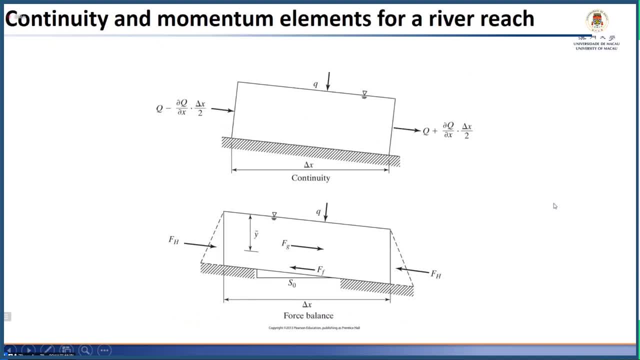 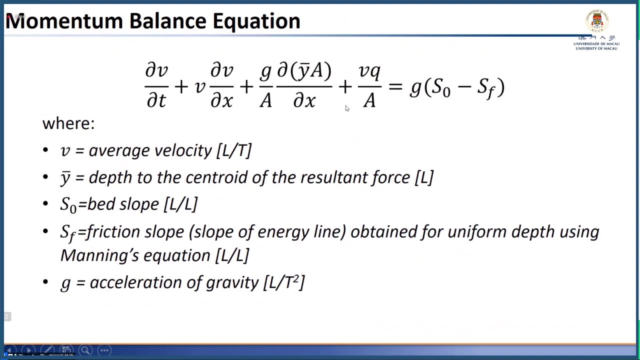 So basically it's based on open channel hydraulics. So continuity and the momentum equations. if you think about continuity equation, which looks like this, then the momentum equation looks like that. And for momentum equation, if we assume the channel is wide enough and there is no Q, which is like external source, then the momentum 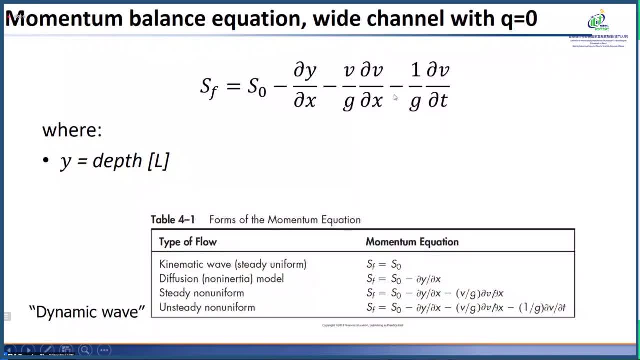 equation can be simplified like this: Although simplified, but it's still quite computationally expensive. So sometimes we do not solve all of the terms. If we solve all of the terms- that is called dynamic weave method- right, And if we assume like it is a steady uniform, then it 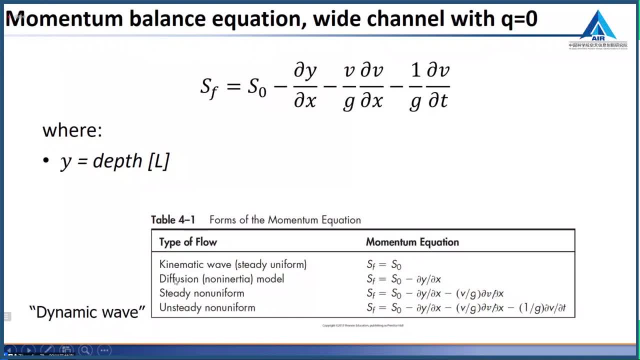 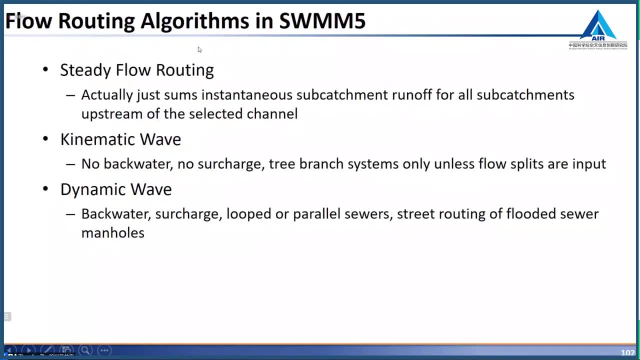 becomes the simple kinematic weave method, right? So yeah, For SWIM. there are actually three options in SWIM, right? So two of them are kinematic weave and dynamic weave. The third one is even simpler than kinematic weave, So it simply doesn't consider any. 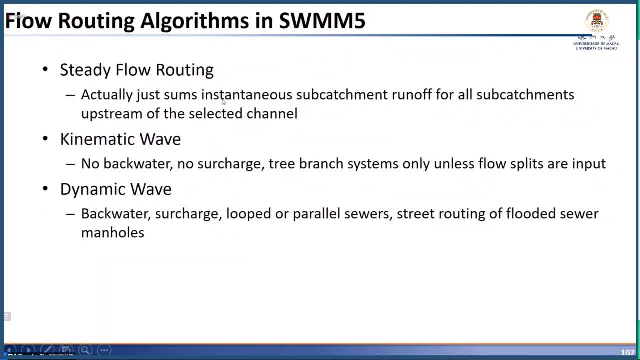 routing. It just sums instantaneous sub-catchment runoff. That's it okay. So this is like purely steady for the whole system. Although kinematic weave, the method is assuming steady flow. However, in SWIM, because the input is time dependent, right? So even though you apply, 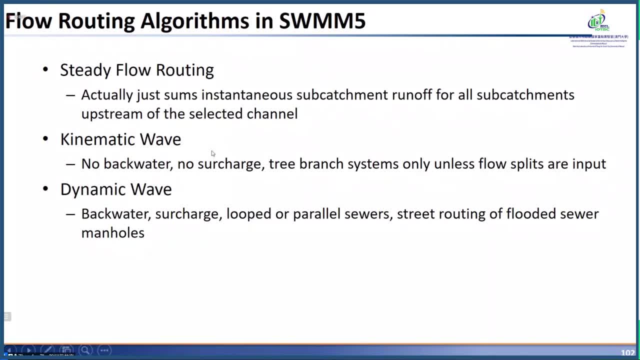 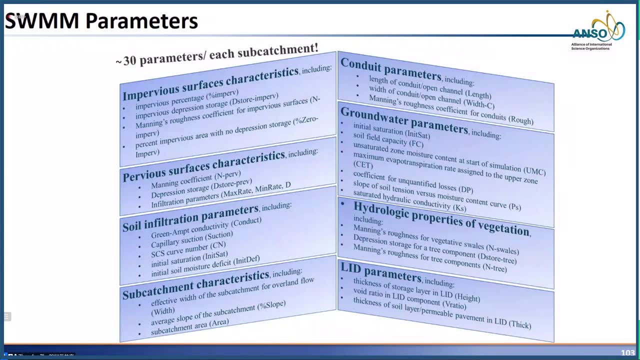 kinematic weave method, you still get a time dependent or somehow unsteady flow results, right? Okay, So in a quick summary, there are about 30 parameters for each sub-catchment in a SWIM model, right, You don't have to read into every single one, but those are a lot of parameters. 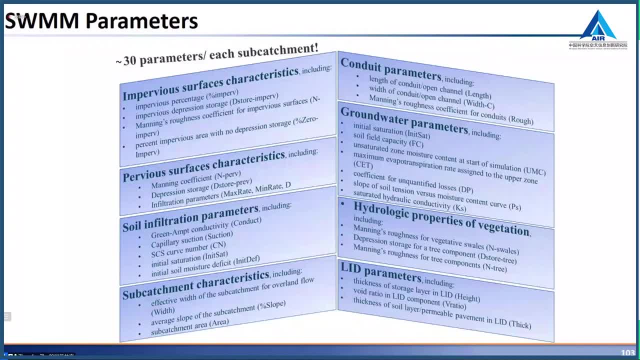 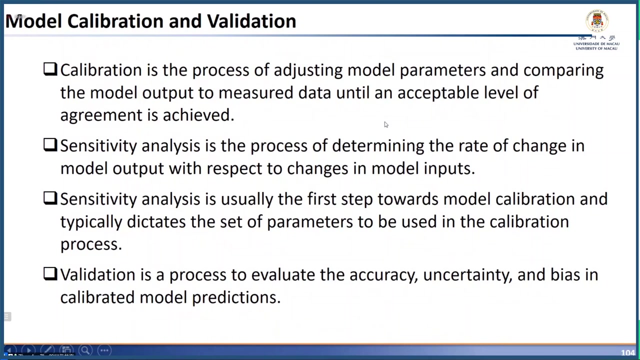 Many of them are not very sensitive, but some of them are quite sensitive. So we have to pay attention to the parameters and the calibration and validation of the model. So by model calibration and validation I mean. calibration is the process of adjusting model. 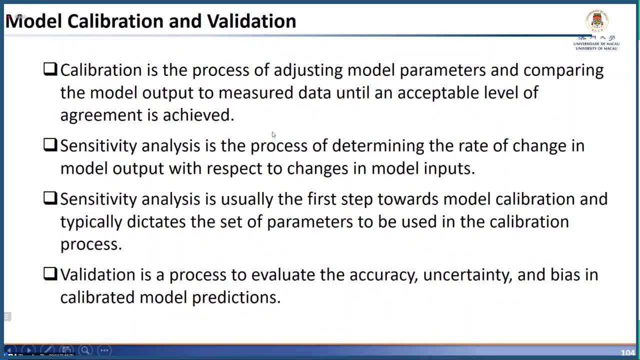 parameters and then comparing the model output to measured data until it reaches a satisfactory or acceptable level. okay, So a pre-step of calibration is normally sensitivity analysis, That is, the process of determining which parameters are more sensitive. right, Because it can save us time, that we don't have to waste our time on. 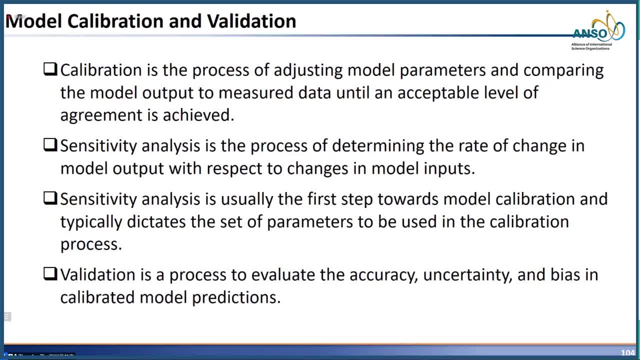 calibrating some parameters that are not sensitive right. So after calibration we also need to validate the model. So the model validation is a process to evaluate the accuracy, uncertainty and bias in calibrated model predictions. So again, today we do not have too much time to go through all of these details here. 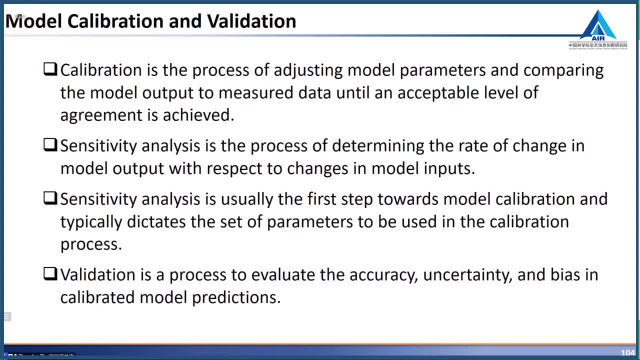 So actually there are a lot to talk about model calibration and validation. So in the next chapter I'm going to go to the next slide. So you can see this is a model calibration and validation that is not an easy task. Again, only touch the surface of this topic. 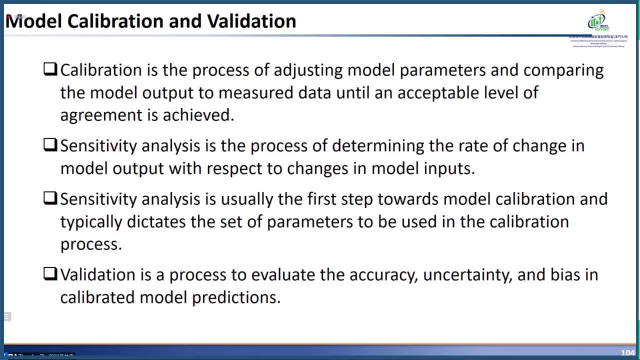 But again, because there are so many parameters in SWIM and there can be also many sub-catchments in SWIM, right, so calibrating such a model is not an easy task. okay, Although model calibration and validation are still a very widely accepted. 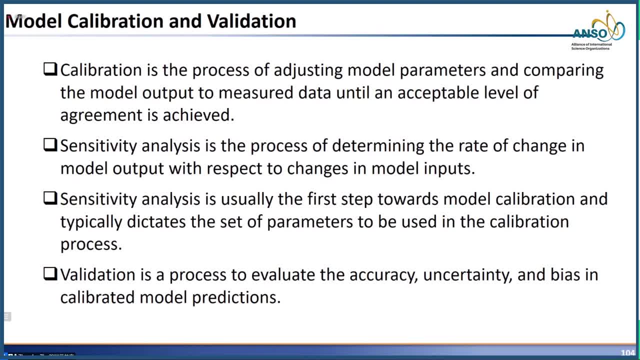 best of practice for hydrologic model development, given. that said, there are ongoing debate or argument regarding the purpose or the necessity of validation. So, if you are interested, there are very recent research talking about whether or not we need a model validation process. 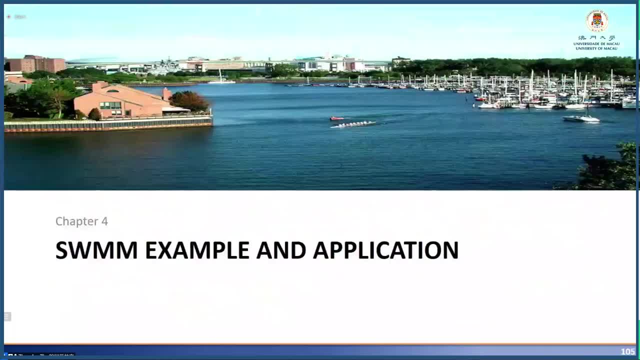 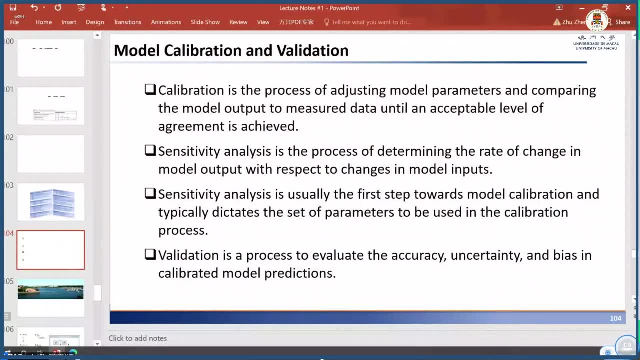 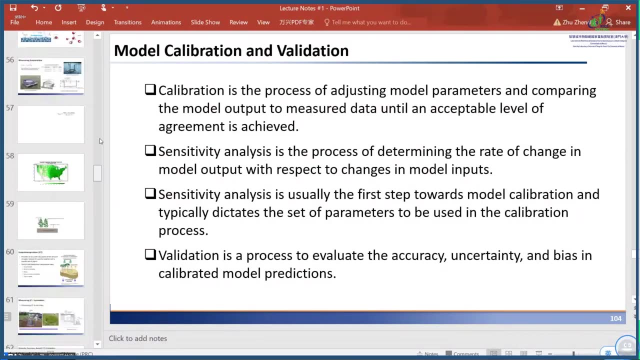 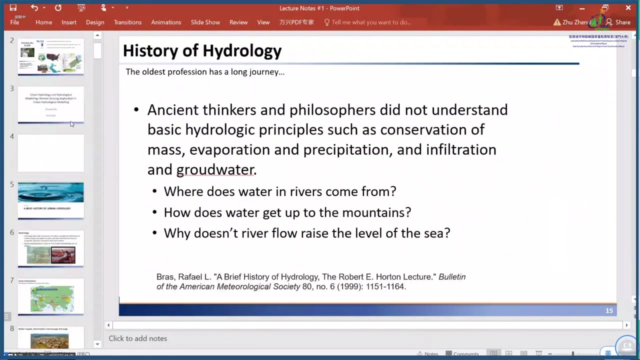 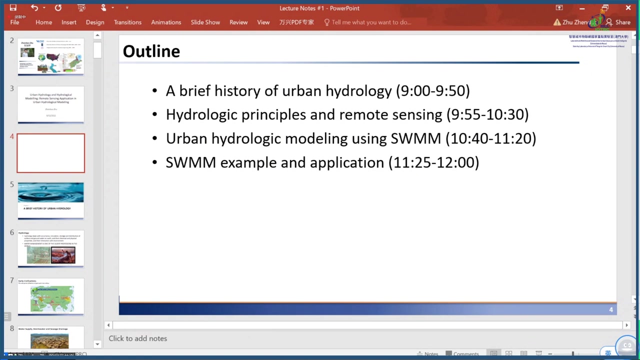 Okay, so I believe this should be chapter three. Let me see what's the time now. I think we are pretty good, right? Yeah, actually we are good. We are even three minutes ahead of time. Yeah, I was a little worried that. 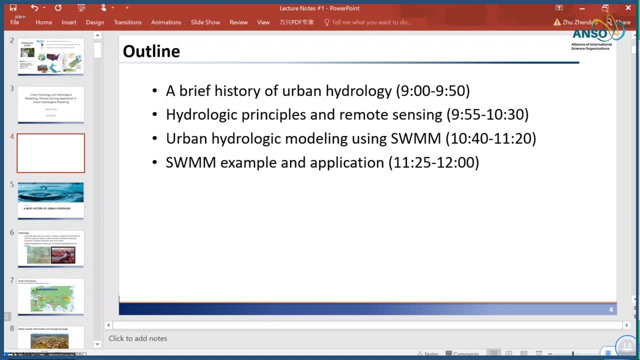 this chapter might take too long, so I probably went a little bit too fast. So if you have any questions, you can type in chat and I will try to answer those questions. Otherwise, let's take a break and we will continue to the last chapter at 11.25.. 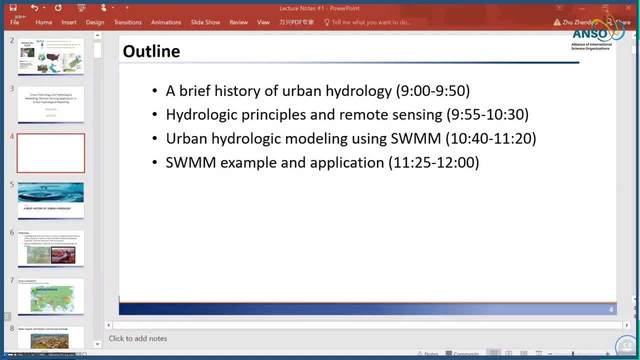 Okay, Okay. So I saw the follow-up question by shortcut early, Alicia, but I think we need to continue to the next chapter. Hopefully after that I may be able to answer. Okay, that I may be able to answer those follow-up questions. 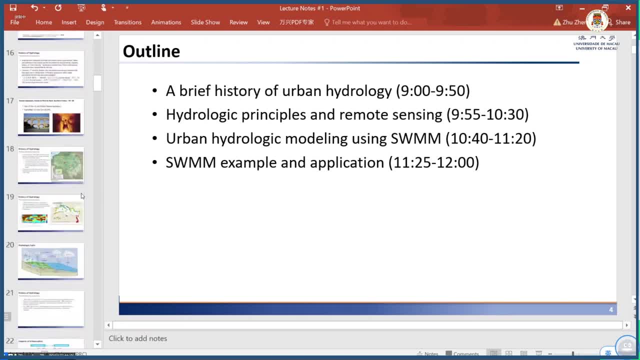 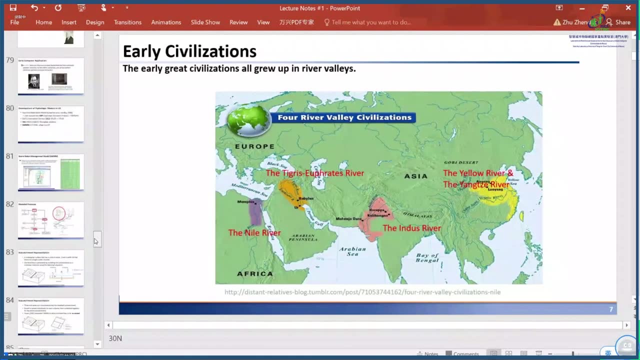 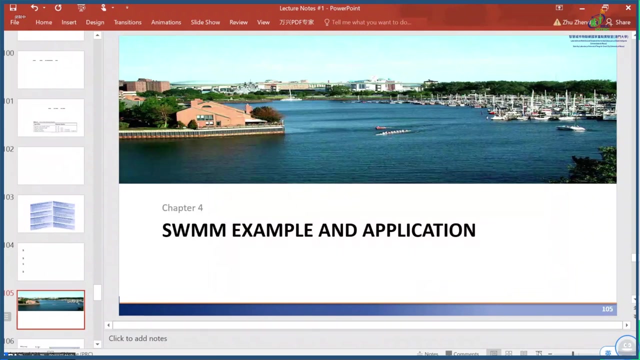 So in the last chapter, I'd like to show you some example and application of SWIM. So we have talked about the series, those processes, formulas. So what can we do with this model? So, unfortunately, if it's an in-person training, 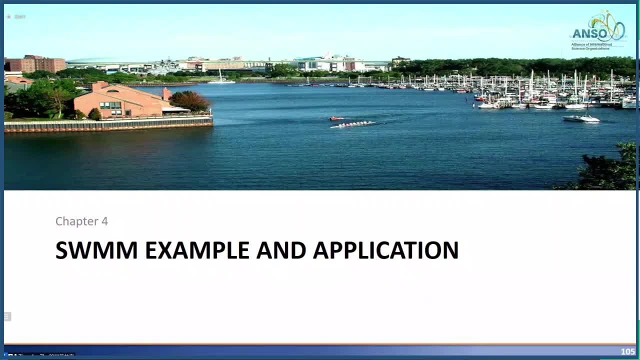 we might be able to do some hands-on practice, But because now it's online, so I think I'm going to show you the example. and obviously the best way to really learn SWIM is actually by doing it by yourself, So I will also upload some instructions as an exercise. 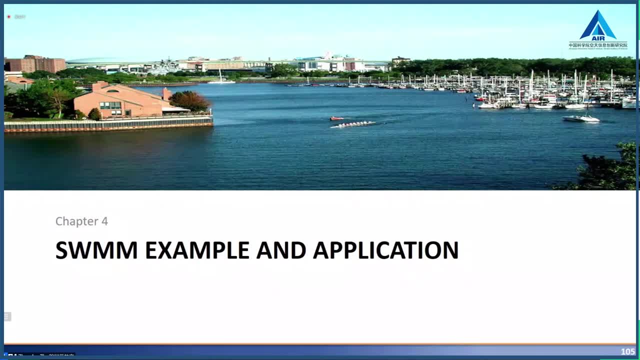 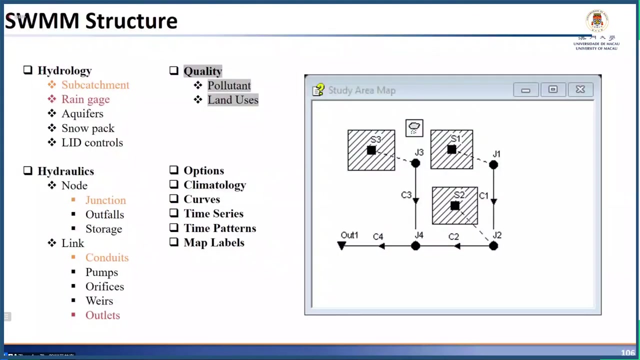 to your online learning platform. So if you are interested, you may want to follow those instructions and do this practice by yourself. So first I'm going to introduce you an example from the SWIM tutorial. This is a pretty simple example with three subcatchments, four junctions. 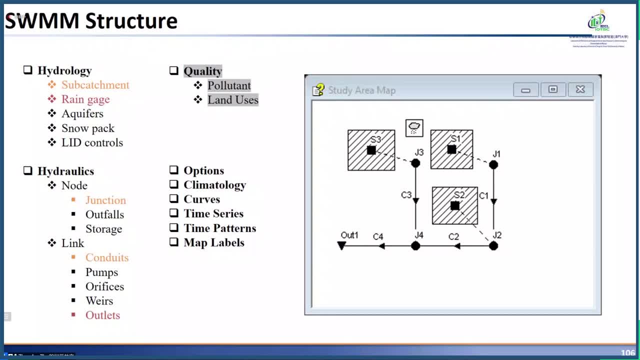 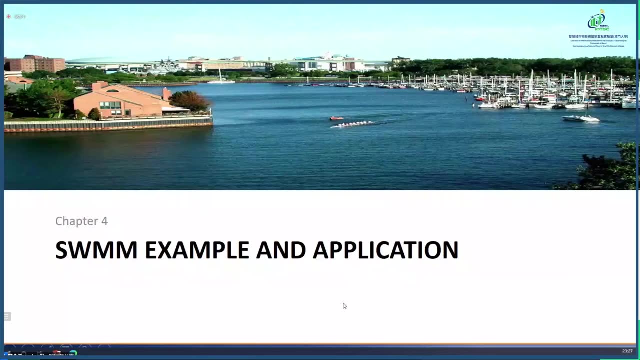 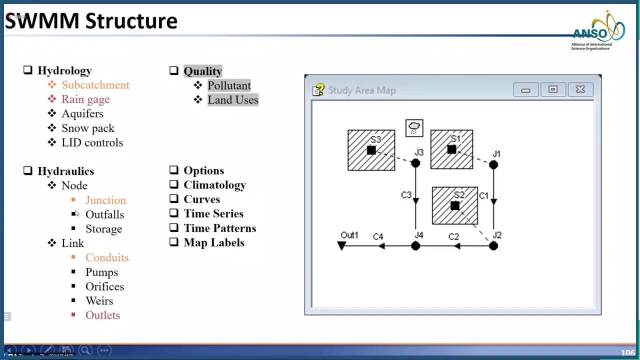 one outfall and four conduits. okay, So this is just for you to get somehow familiar with how a SWIM model looks like. okay, So basically there are those like three main components. One is hydrology, right, One is hydraulics. 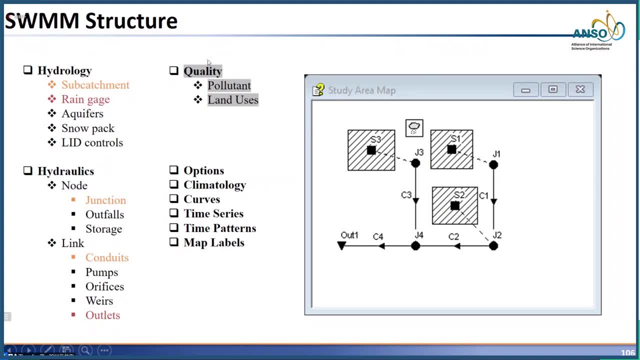 Then one is water quality. So here today we are not going to focus on water quality, but mainly hydrology and hydraulics. So there are also others like options, climatology curves, time series, time cycles, patterns, map labels. So I think later I'm going to show you the graphical user interface so you can. 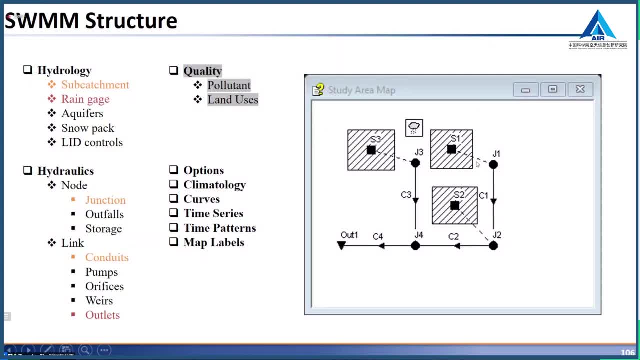 get some idea. So the main components here, at least for this example, are subcatchment. So those are: subcatchment, Rain gate. you have to provide precipitation data, either rain or snow. So there has to be a precipitation data as an input. Then for the node it can be junctions. 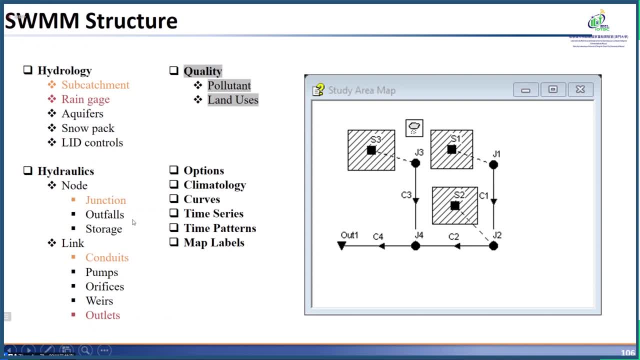 like those like G1, G2, G3, G4.. It can be outfalls like this, So this is the final outfall. Then, for the links, there can be conduits and there also can be outlets. So those are the 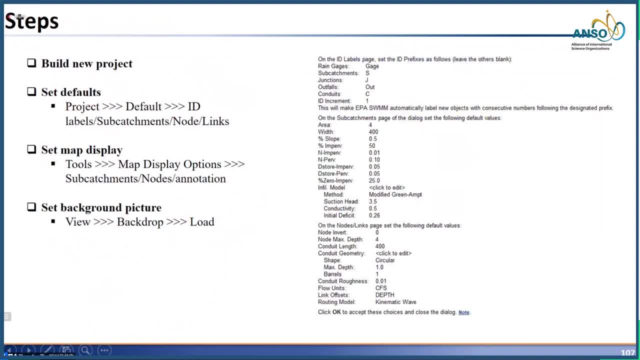 different components. So if you follow the tutorial steps again, unfortunately we're not going to do it step by step together, But the steps are as follows: First you need to build a new project, Then you need to set the default values, Then set the map display, set background. 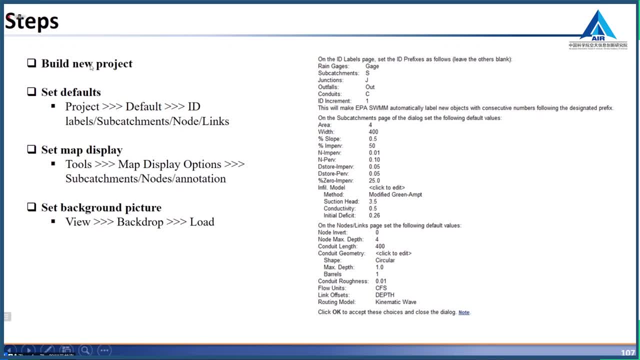 picture. Those are optional, So of course, building a new project is mandatory. Set defaults are also optional, but highly recommended. Set map display and the background picture are optional, So you don't need to do it all the time, but they can be helpful. So here, 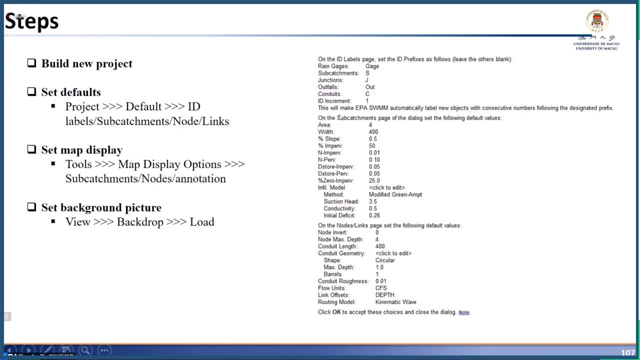 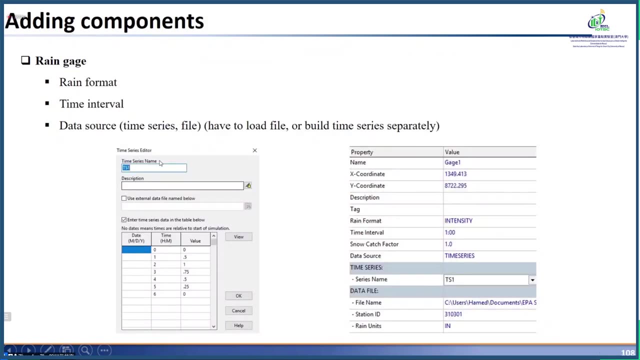 if you follow that tutorial, it gives you the parameters for each subcatchment, For each node or conduit, So you just have to follow this step by step. So for the ring gauge, I think it's pretty straightforward. You need a time series. 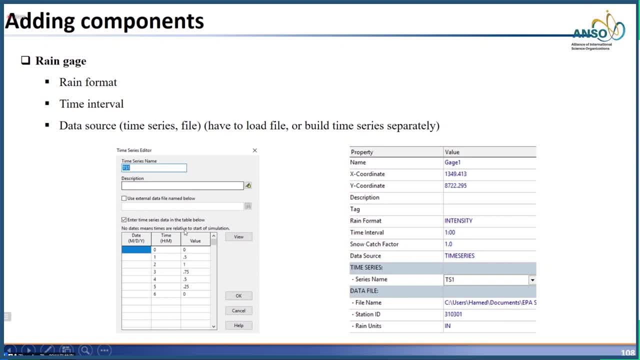 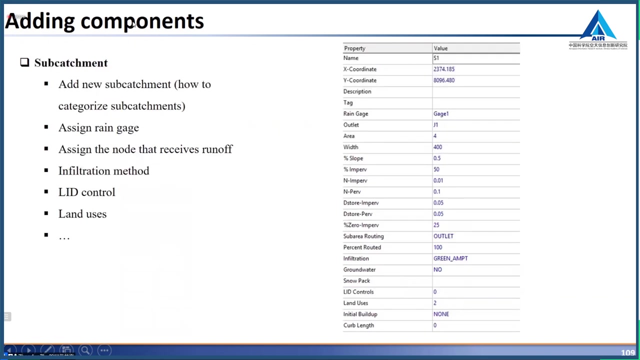 for the rainfall hitograph. So remember what a rainfall hitograph is. That's the time series over rainfall intensity. So this can be a time series, So the data actually can be manually input. It can also be input at the fire Then for the subcatchment. those are pretty straightforward. 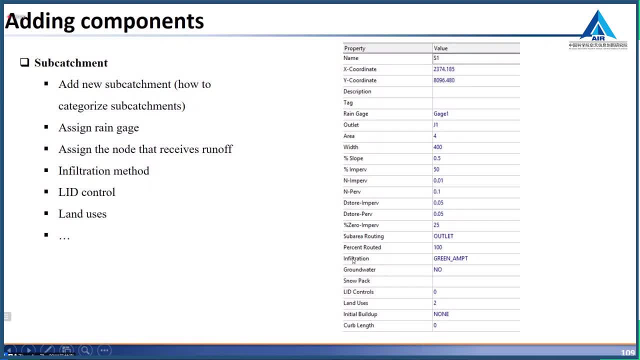 So it's going to skip this. Just keep in mind that infiltration- you have to select which method you want to use for infiltration. Here we select the green apt. MCC groans for a moment. after seeing this alpha code and my mixed state data, screen error appears high. 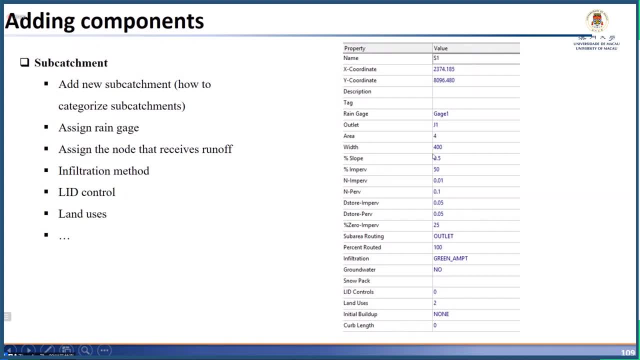 other parameters like the area, the width, the slope, percent of imperviousness. Manning's roughness for impervious area. Manning's roughness for pervious area. depression storage for impervious area. depression storage for pervious area. 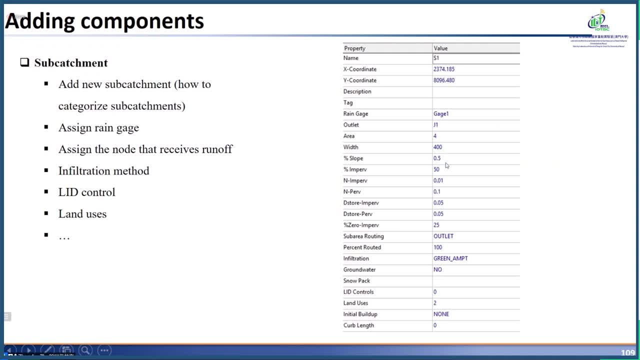 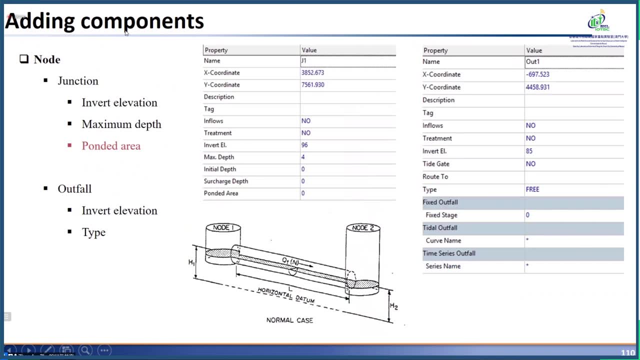 right, and so on. Okay, so those are different parameters or different settings. So for the node, first is junction and then there can be also outfall, right? so here, imagine: like you know, this is a junction, right? so? 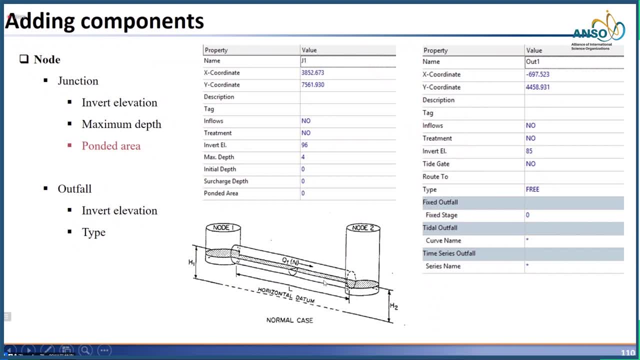 between two junctions, there can be a pipe or conduit connecting the two junctions. I think all the others are pretty straightforward. The only one I want to explain a little bit more is this one. This one is a little bit more. is a little bit more is what's called pounded area, because this may not be. 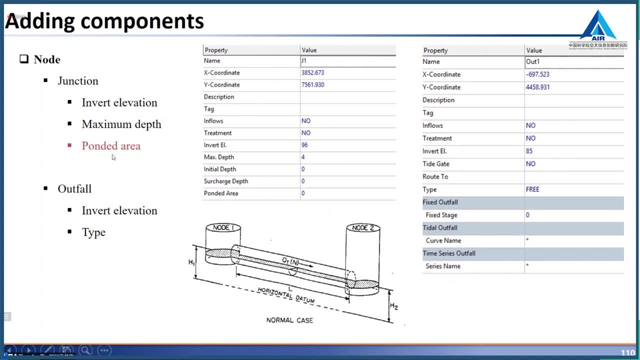 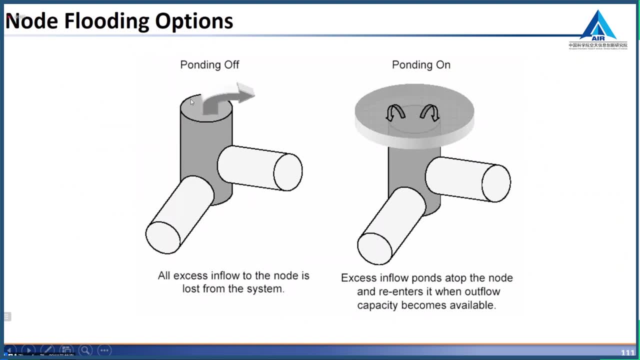 straightforward to understand. So what does it mean by pounded area? Pounded area means: imagine this is a manhole, okay, in this manhole. so obviously the storm runoff can get into the drainage system from this manhole. However, if 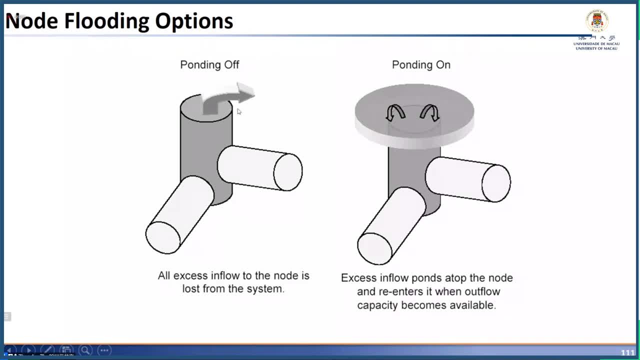 there is too much storm runoff coming in right, so there could be a lot of. So if there is too much storm runoff coming in right, so there could be a could be pounding water on the street, And if there are too much pounding water, that can be a street flooding. So, however, 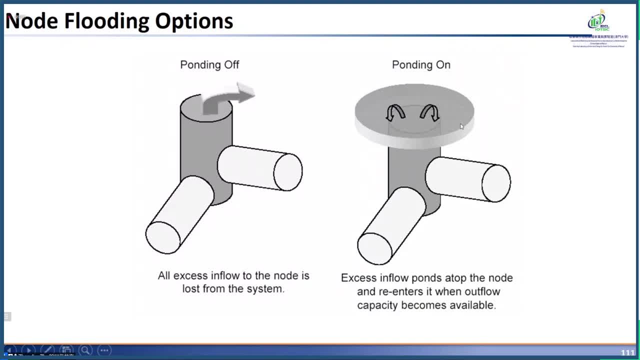 there is an option in SwimModel to either select pounding off or on. So if you select the pounding off, that means all of the access inflow to this node is lost from the system. So basically you do not consider any pounding at this junction, or. 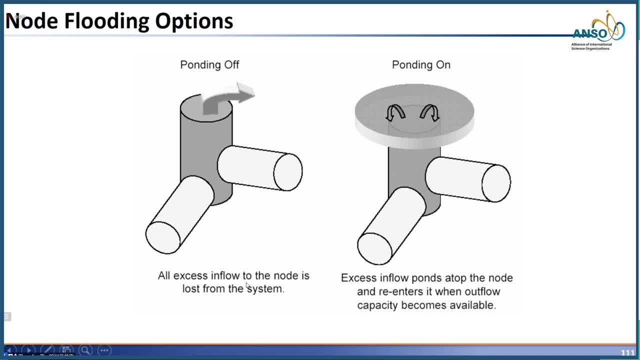 at this manhole. It could make sense sometimes if, imagine, your junction may actually be close to some surface storage, so if there is pounding water, actually it will go to the surface storage and it will not come back to the drainage system. So in that case this option will make more sense. 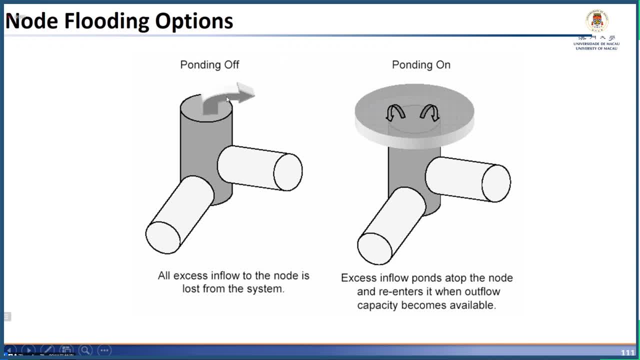 It's more reasonable to select pounding off. However, there are other cases that you should consider pounding, especially if you are starting street flooding. So have to consider pounding on. And if you select the pounding on option, then this access inflow will pounce at the top of this junction or the node, And then 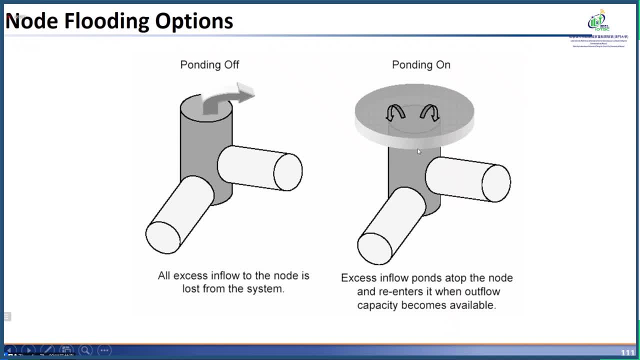 later it will re-enter the drainage system when the outflow capacity becomes available. So obviously you can give the surface area for the pounding water. So the area does not have to be just the area of the junction, because normally the area of the junction 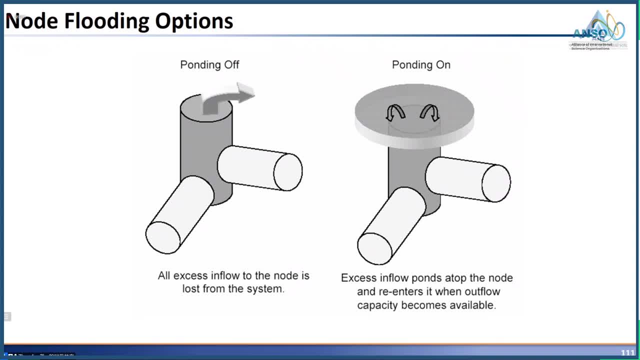 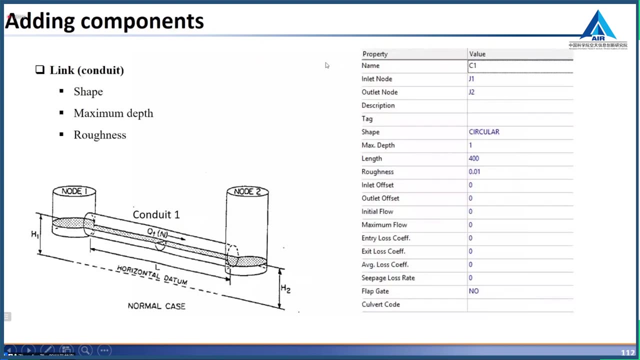 is very small, If an area of the manhole that is normally very small, But the pounding water actually can be distributed on a much larger area. So that will become another parameter to consider. So for the link or conduit, so you need to specify the shape of 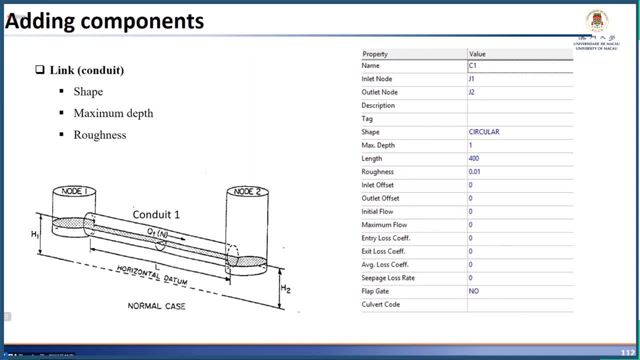 the conduit, the depth of the conduit and the roughness of the conduit. I think all of those are pretty straightforward. So for roughness, maybe you know this is normally an important calibration parameter because the roughness controls the routing. 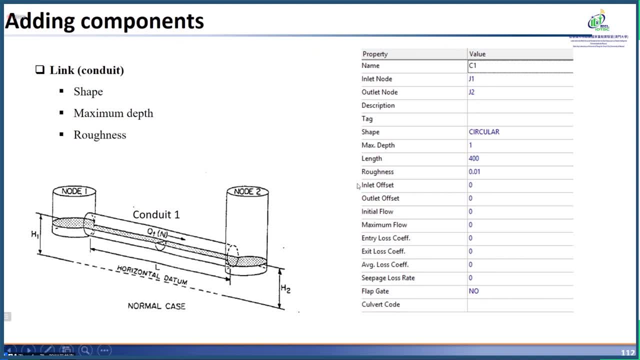 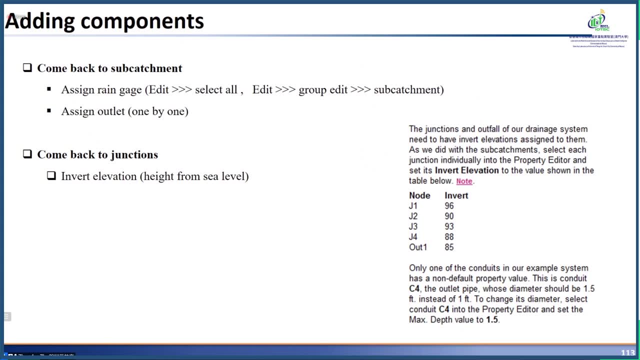 process right. So roughness is pretty sensitive And okay. coming back to a subcatchment, you know you need to assign a ring gauge to a subcatchment and also assign outlage to a subcatchment. And then back to the junctions. you 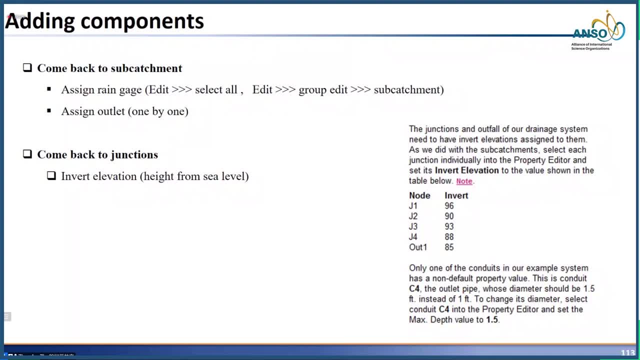 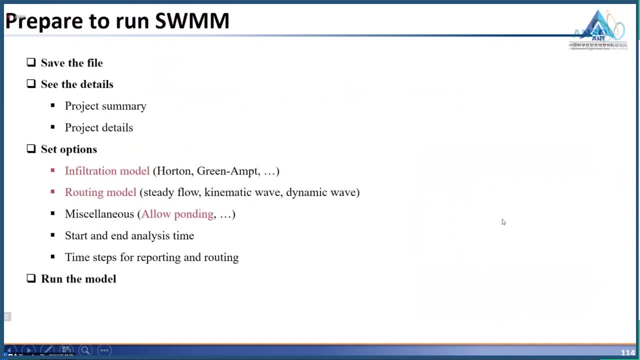 need to give invert elevation for each junction. Okay, so those are also actually straightforward if you follow the tutorial. Okay, So for the options you select: infiltration model, routing model- we have introduced those, whether or not allow pounding right and so on. Okay, so then you can run the model. So let me 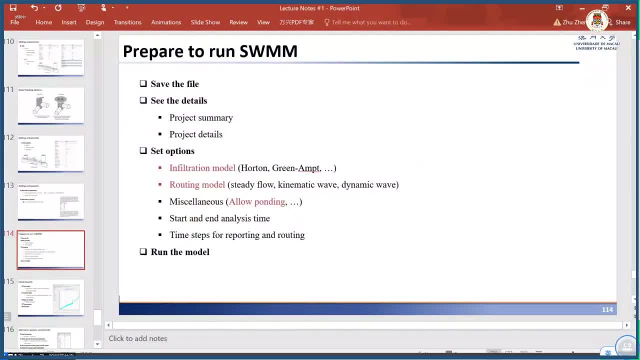 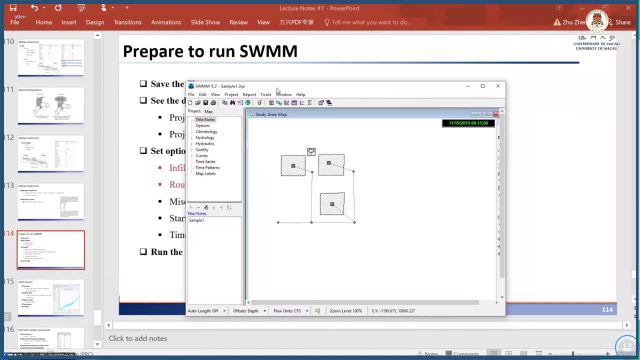 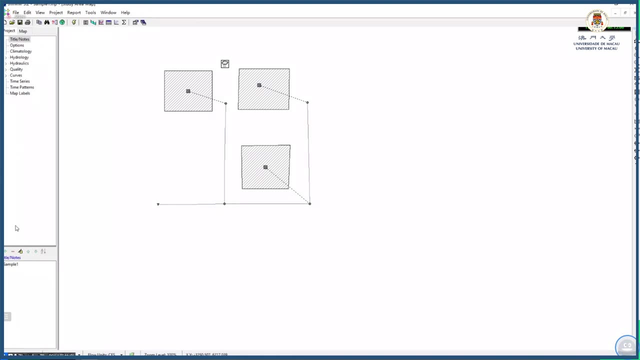 bring up the SWIM model, this simple example That I've already built. okay, So, as you can see, first this is the graphical user interface of SWIM, right? So you have the toolbox, the menu, and then in the project there are different options. So those are. 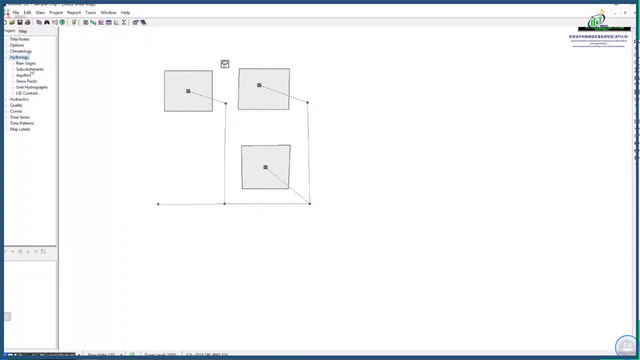 options: climatology, hydrology. Then there is a ring gauge, subcatchment, and so on. right Then hydraulics. So quality curves, time series: right. So this time series is for the rainfall, right? So if you go to the ring, 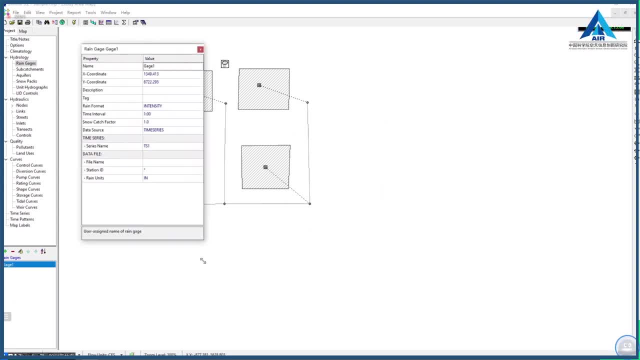 gauge. let me make it louder, right as you can see the data source. you can select the data source. you can select the data source. you can select from time series or it can come from a file, And if you select time series, you need to tell like which time series it. 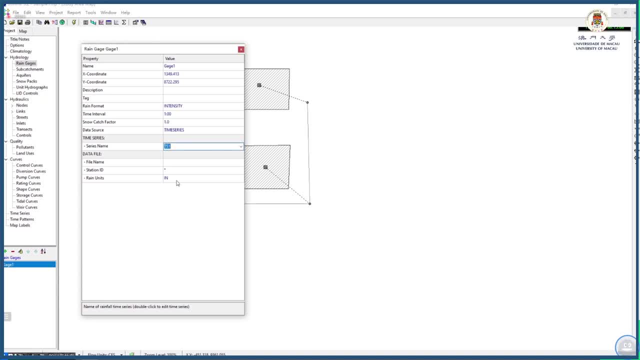 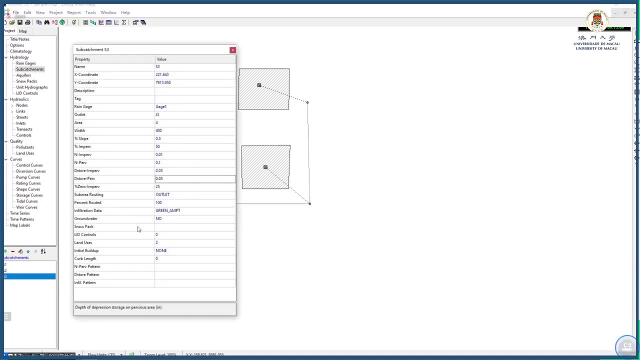 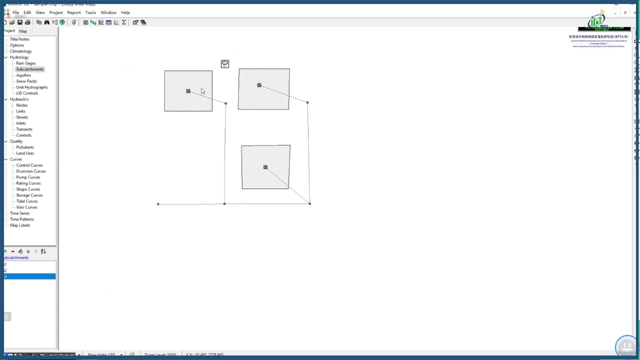 is right. And also the unit is that in inch or millimeter you can select. So this is for the ring gauge For subcatchment. as you can see, those are the parameters of each subcatchment. So each subcatchment, the runoff need to be discharged to outlet right. 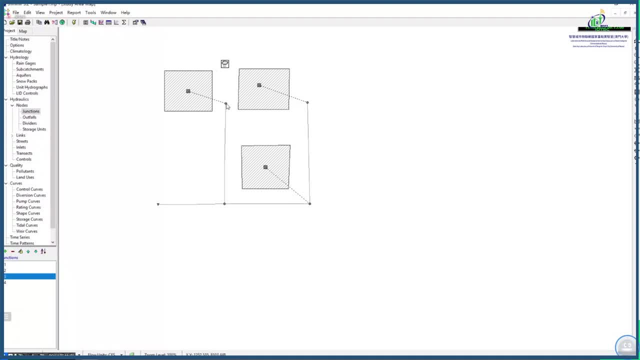 By outlet I mean the outlet of the subcatchment. So in this case it's a junction, right? So this is a junction that will receive outflow from this subcatchment. Same for here, right, This is a junction receiving flow. 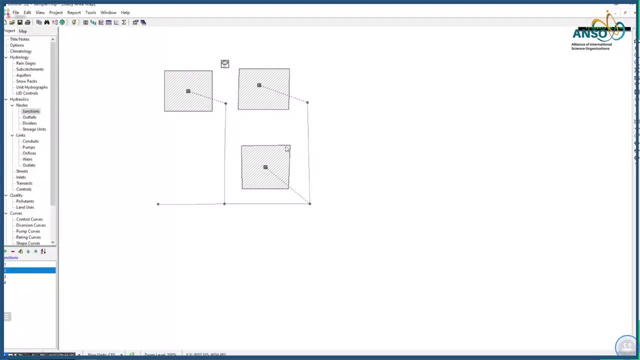 outflow from this subcatchment, These receive outflow from this subcatchment, And then those junctions are connected by pipelines, right, And finally it goes to outflow. Okay, So you can run the model, Obviously this. 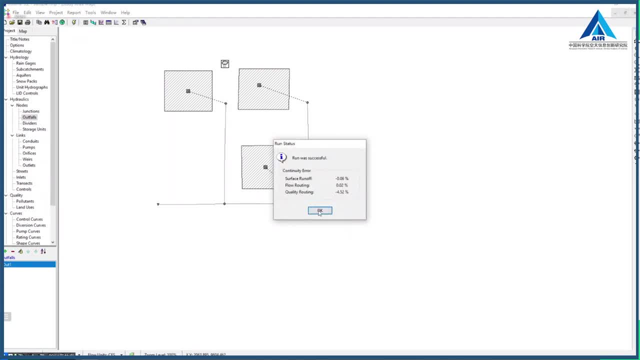 is very fast because it's very simple. Again, only three subcatchments, like four junctions. This is a very simple model And we also run it for only one rainfall event. right, It's a very short event, So there are a lot of different ways to actually. 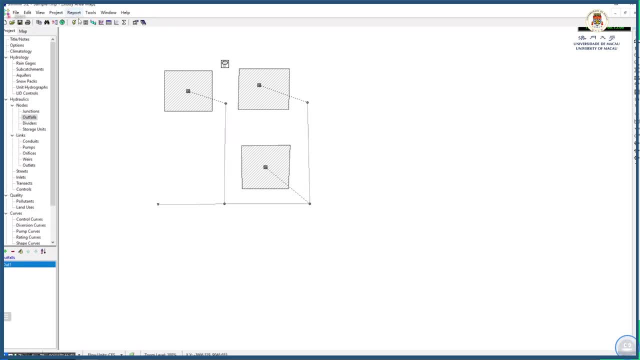 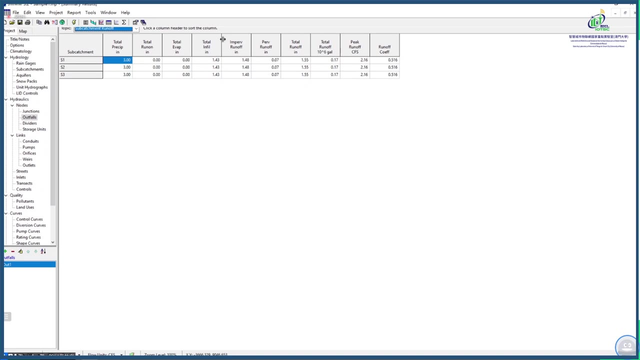 visualize your results, right So normally I will start with the report. So if you go to the summary report, this gives you a summary of total precipitation, total runoff, total evaporation, infiltration runoff and so on for each subcatchment. right So you? 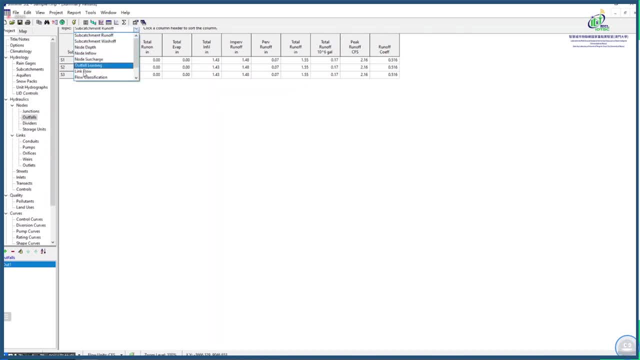 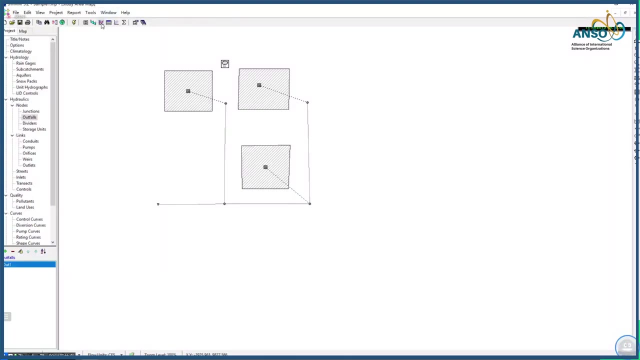 can also go to different node, different conduit right. So this gives you a summary. Of course, this is the summary of the whole simulation period. If you want to get a time series right, so here you can do time series plot for. 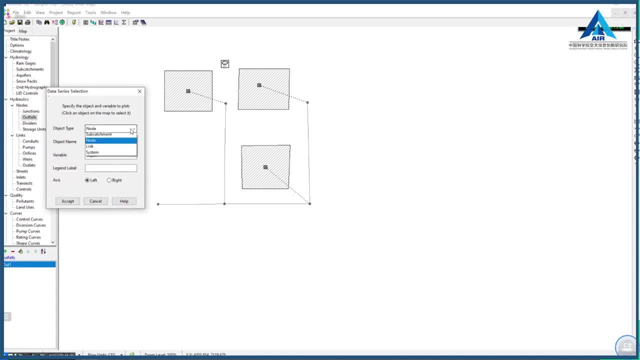 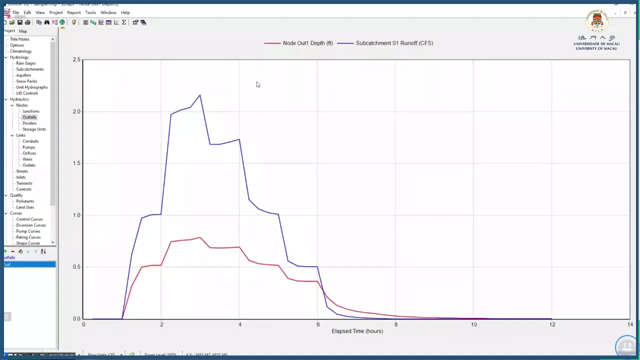 different options. For example, we can add subcatchment, say runoff. We go to subcatchment one. I hope this is called subcatchment one. Okay, as one, All right. So this plot the runoff from subcatchment one. 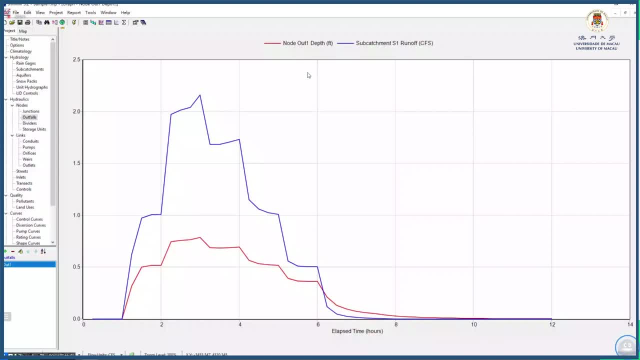 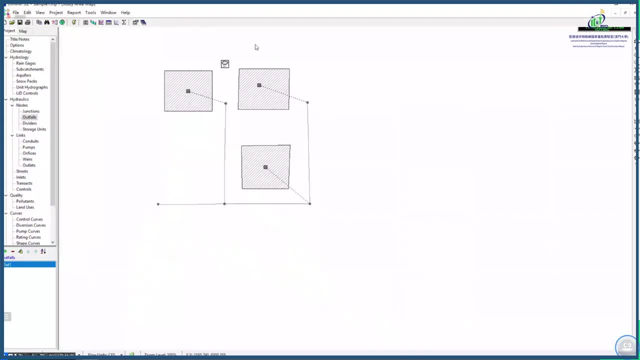 we can also add subcatchment one And we also include the water depths at the outlet right, So you can actually include multiple curves in the same plot. So this is for time series right. Another useful way to visualize the results would be to do a profile plot. 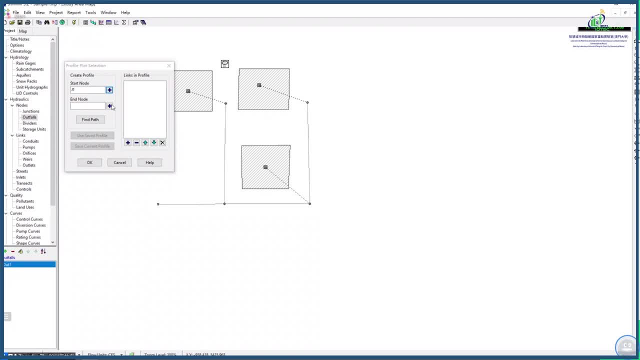 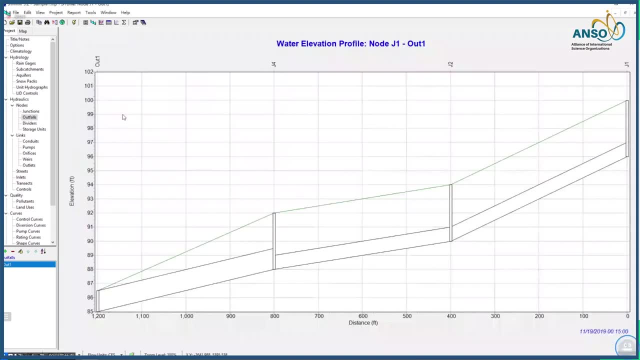 All right, So let's start. So let's start with Junction 1.. fall and find the path C1, C2, C4. So this gives you from junction 1 until the outfall. So if you go to map and this actually 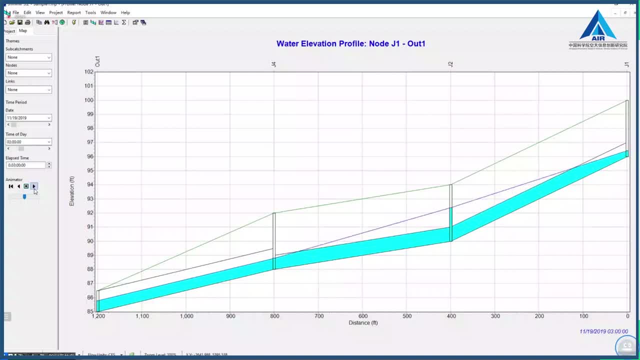 can play a video showing you, at a different time, how the water level changes in each conduit and also at each junction. So you may notice one thing that- let's go back to the beginning. You may notice one thing: that all the time, at each junction or at each conduit, 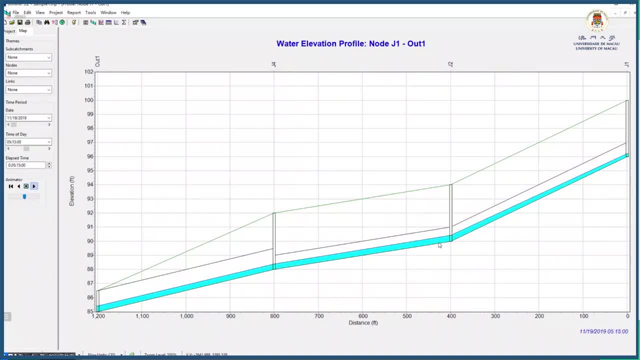 the water depth is actually uniform, Unless it becomes pressurized. So if it is unpressurized, as you can see, this water depth is always uniform in each conduit. So that indicates that you are adopting a kinematic weave method for the hydraulics. So what if we do? 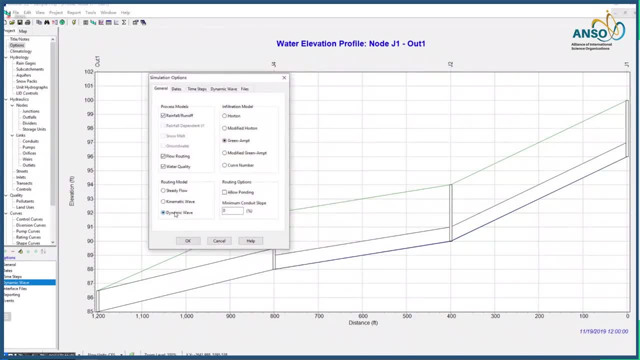 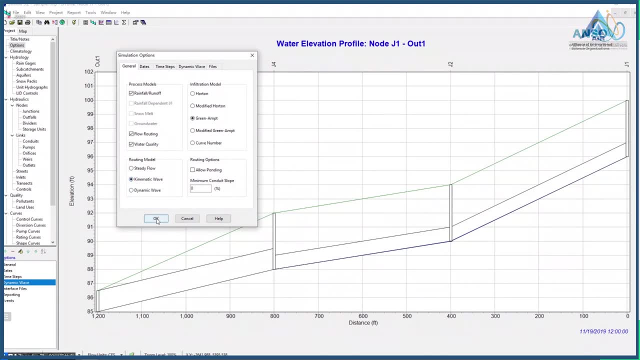 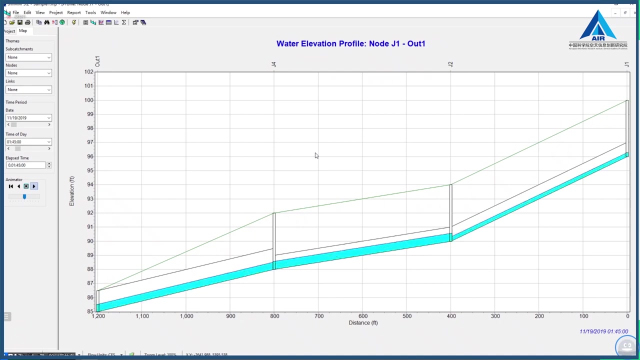 a kinematic web method for the hydraulics. What if we do a dynamic weave? Oh, actually, that may already be. Let me see if we do a kinematic method forер surg method. Okay, See, when you do kinematic wave method at all the time. 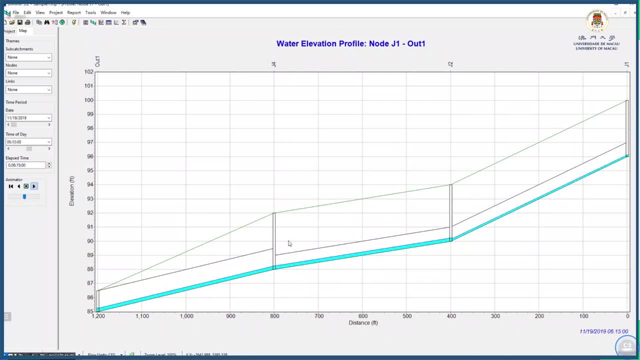 this water depth is actually uniform in each conduit And at a certain time it actually overflowed at this junction, junction 2.. So that is given by the kinematic wave method. However, if you select the dynamic wave method, if you select the wave method, 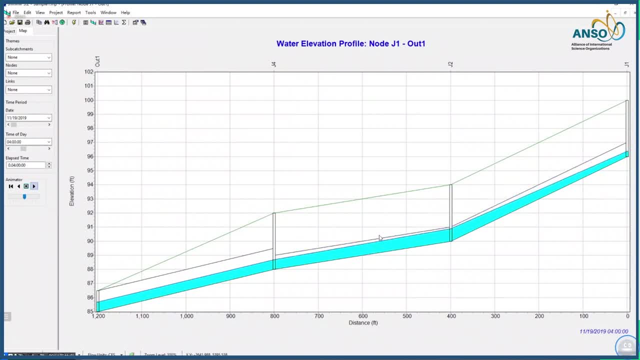 then you know when it becomes pressurized So it can actually resolve the water depth variation within each column conduit. So in that case you can actually see junction 2 actually will not be flooded, So that node flooding given by kinematic wave could be false. 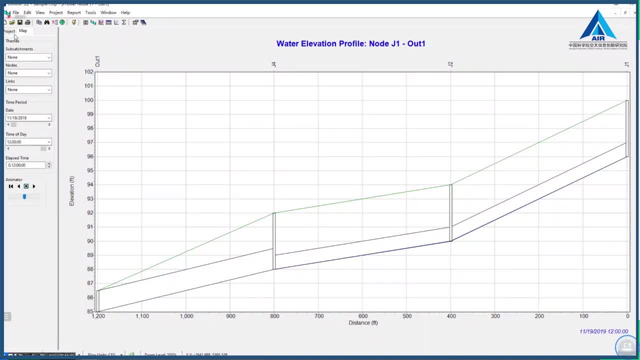 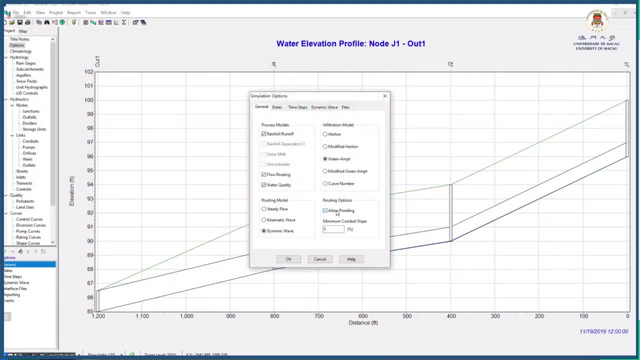 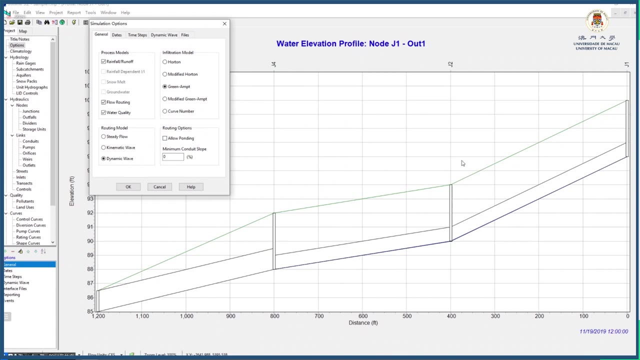 So this is the difference between kinematic wave and the dynamic wave. There is also a difference, if you want to try that, allow pounding or not allow pounding. So in this case, because if we use dynamic wave there is no node flooding, So then the pounding doesn't matter. 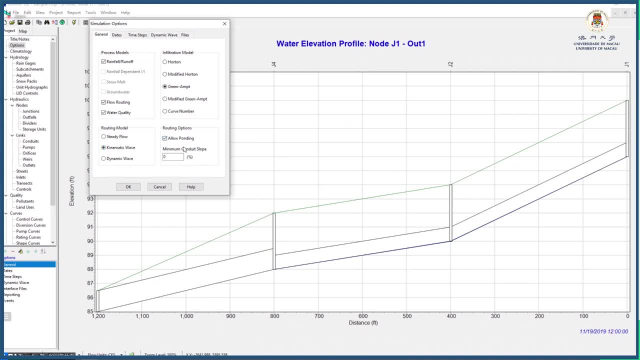 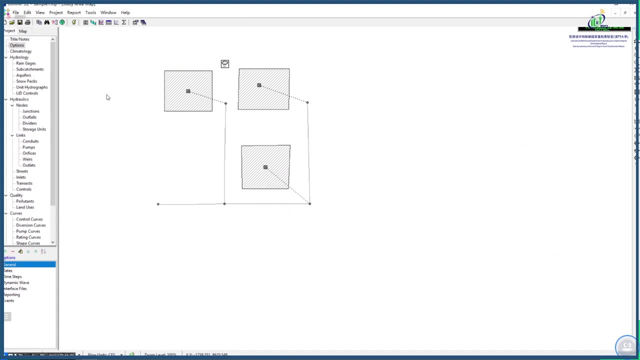 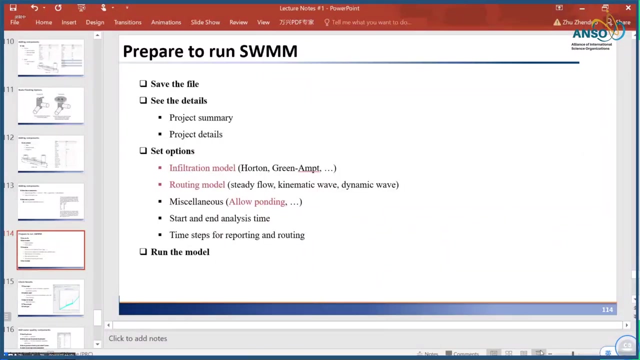 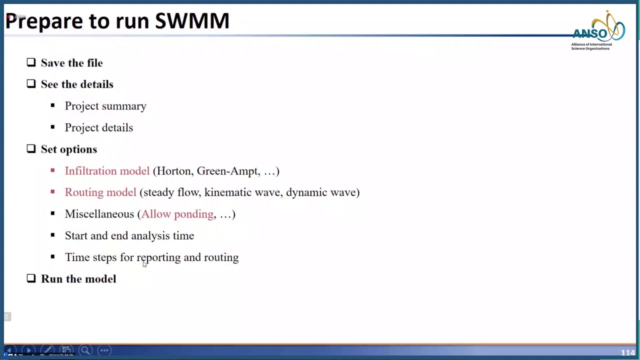 But if you select kinematic wave, allow pounding or not allowing pounding, that will make a difference. So that's something you can see. That's for the visualization of this. OK, Let's go back to all right. So here in this example, we do not. 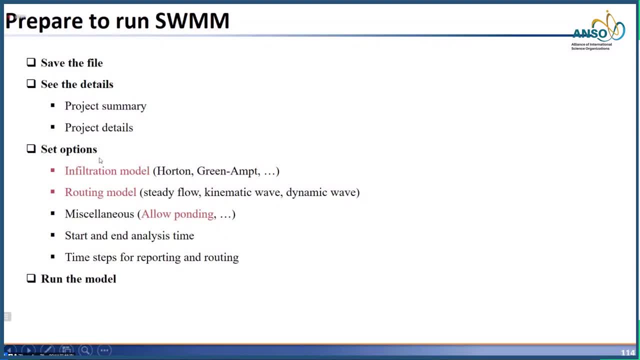 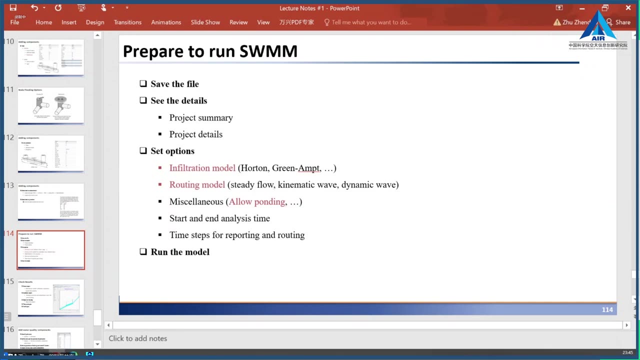 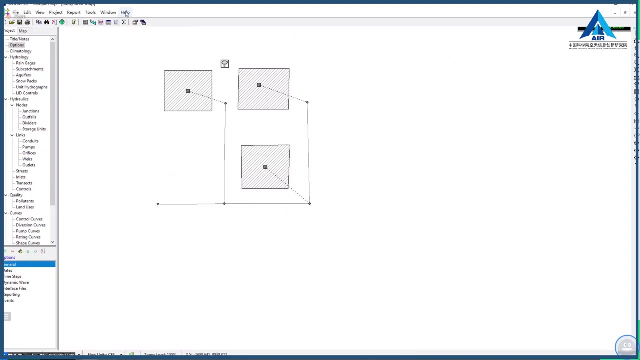 do any calibration or validation. So this is just a simple exercise to build a simple swing model and then run the model. Oh, by the way, I forgot one thing quickly. OK, Let's see That simple example, this simple example. 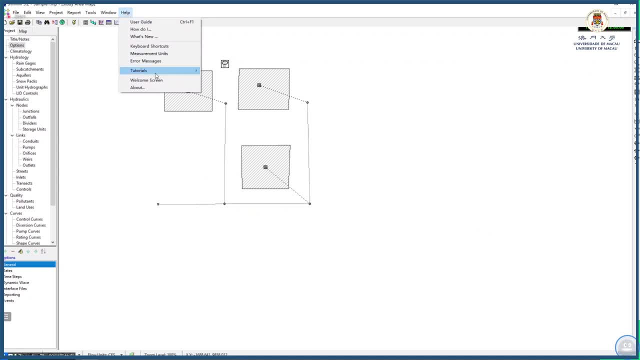 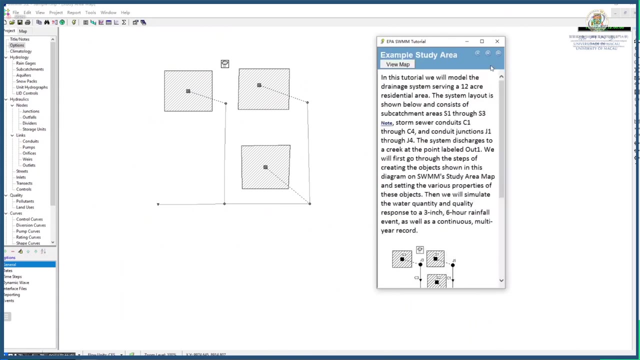 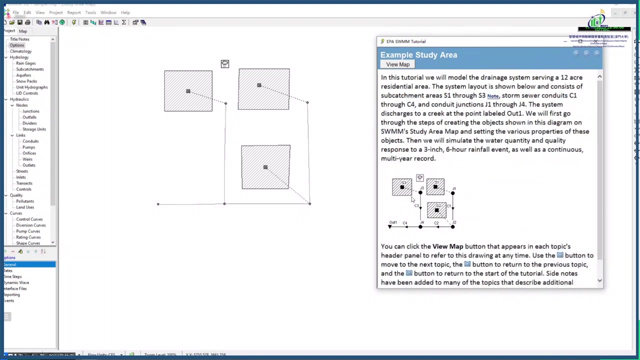 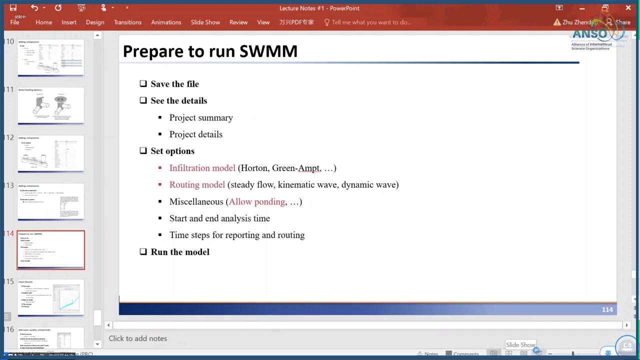 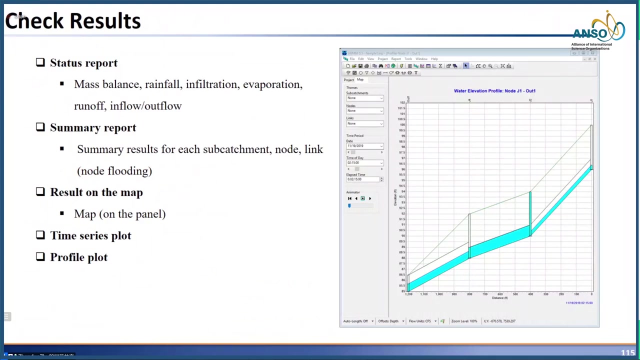 actually, if you go to tutorial, you go to basic tutorial. So this is actually the tutorial, The tutorial you could follow, right. So, as you can see, following this you will get a model like this, right? So here are the different ways to check results. 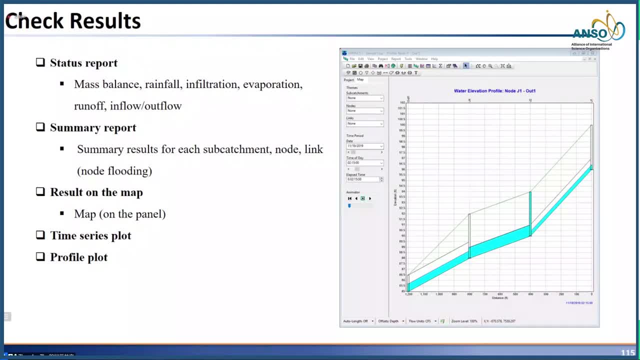 All right, All right, All right. So here we have the data report, the summary report, results on the map, time series, plot, profile, plot. So I think we have shown everything except the result on the map. OK, But again I think we can skip it for now. 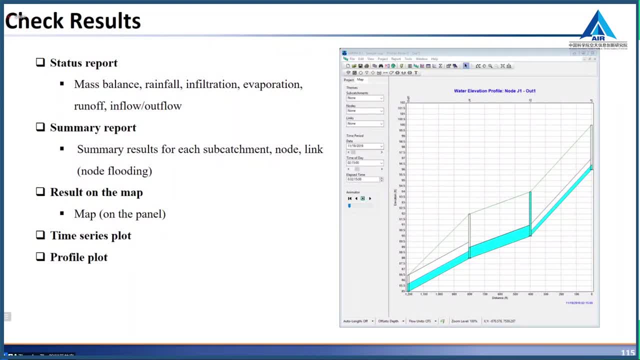 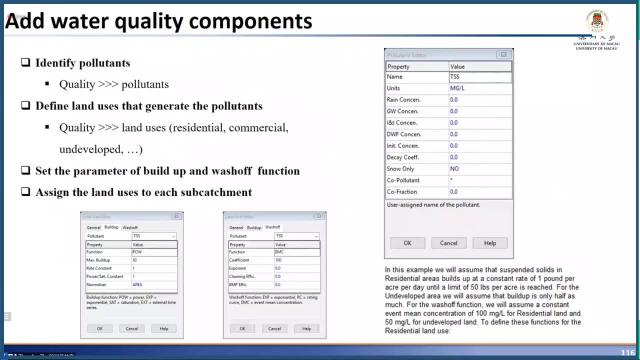 So it's actually pretty straightforward if you explore this a little bit. OK, All right, Let's go to the next slide, please. So there can also be water quality simulated using SWIM. So, however, the water quality module is still quite simple. 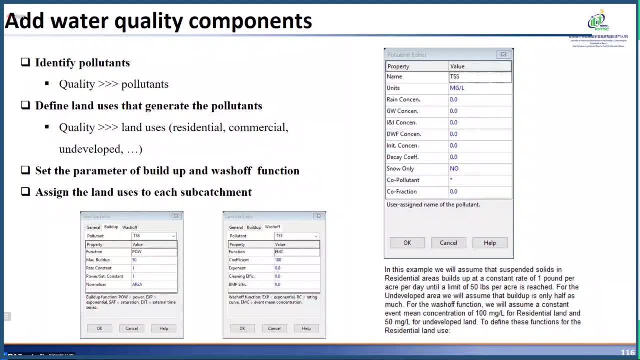 In a way that also indicates that our modeling capacity for urban hydrologic water quality, you know, is quite high. OK, I think there are still a lot of improvements to be done, like both the understanding and also like you know. 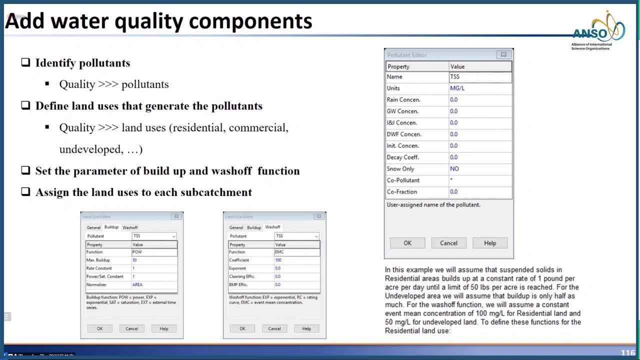 how to model it correctly. So in SWIM, how it does the water quality modeling, is by basically two processes: One is called the build-up and one is called the wash-off. So the build-up process is under the dry weather, So it simulates. 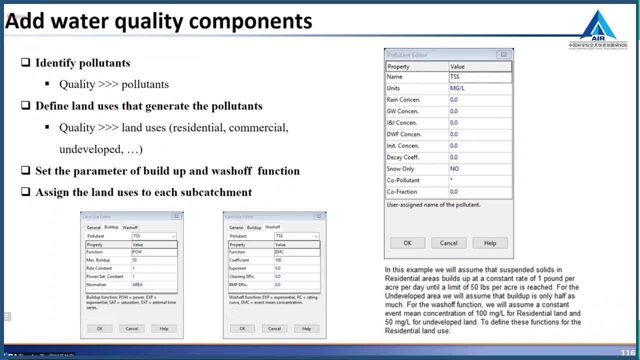 It simulates the build-up of pollutant on the surface right. So these are modeled as different empirical formulas like power function, exponential function and so on. OK, So as you can see here on the lower left, here there are different functions. you can use power, exponential. 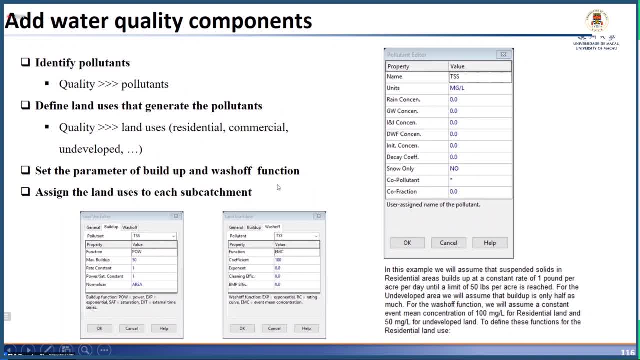 saturation, external time series, Therefore wash-off. similarly, they are empirical formulas, So these include exponential reading, curve or event mean, concentration, EMC. So if you follow the tutorial that you know, you can see how the water quality here. 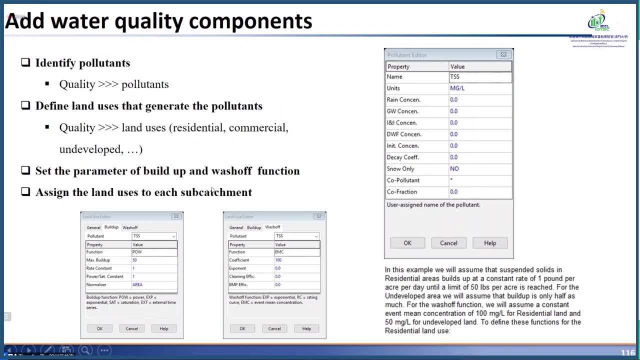 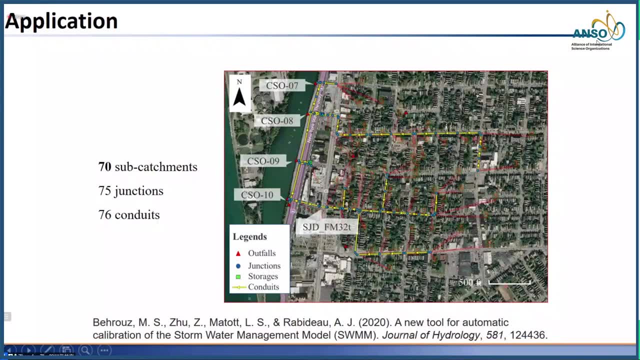 simulated as the TSS total suspended solids. OK, So that is a simple example. right Here there are a lot of applications of SWIM models. I think if you do a literature research, do a literature review, like you know, you will find thousands. 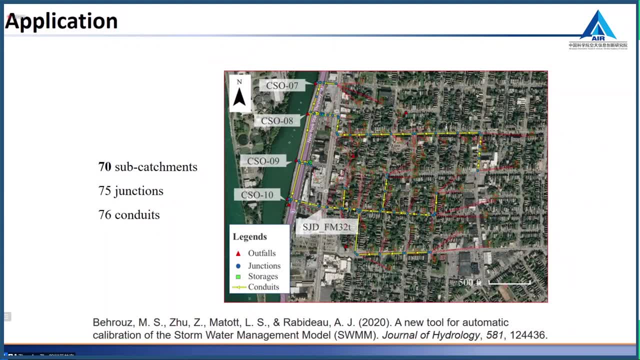 of different applications. So here I'm showing you like something we did recently, that you know is a small subcatchment within the city of Buffalo, So that includes about 70 subcatchments, 75 junctions, 76 conduits. 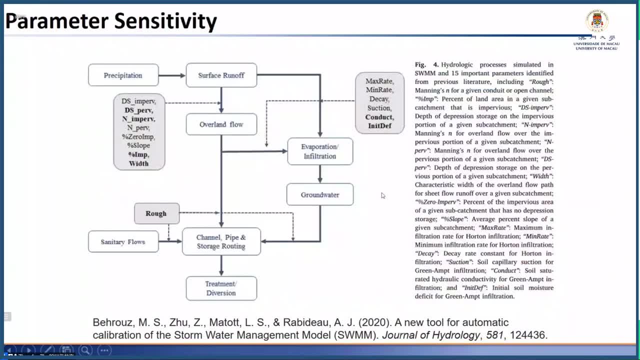 So obviously for this more realistic model, we need to spend a lot of time and efforts on model calibration, validation. So here we summarize. OK, Thank you. We summarized like all the sensitive parameters people have found in literature And then, based on that, we did our own sensitivity analysis. 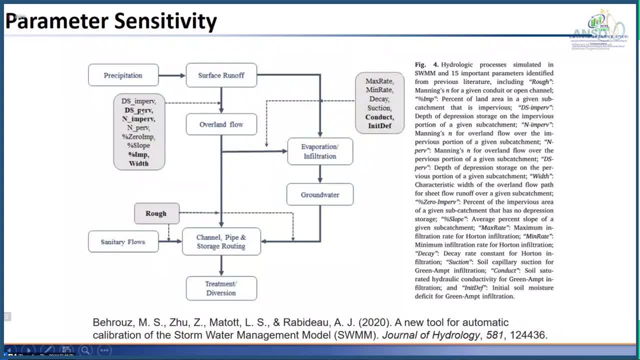 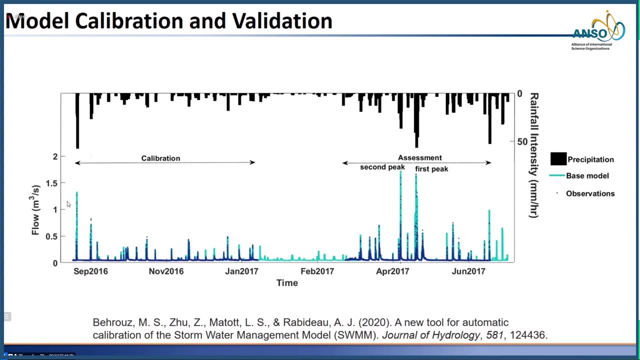 and find out which parameters are the most sensitive in our case study, Then by calibrating the parameters. this is just to show you that the comparison between the simulation and the measurement. So here on the top is the rainfall heat graph And then on the lower part this is the flow time series. 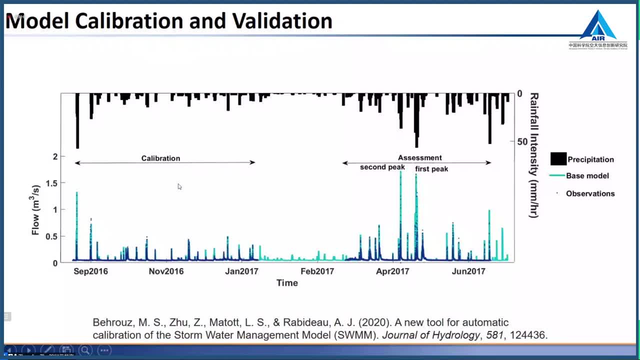 from 2016 to 2017.. So we pick these six months- about half year- for model calibration and then the second half year for model validation. OK, So, as you can see, the model actually can predict those events pretty well. 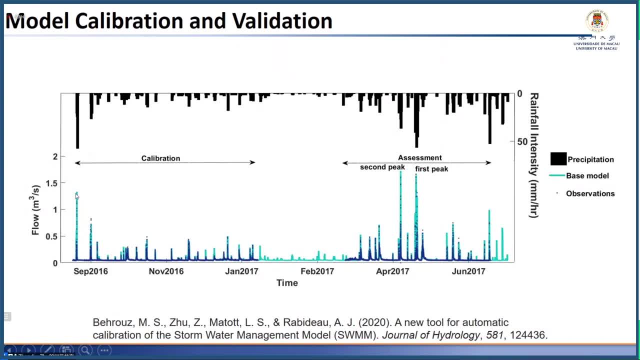 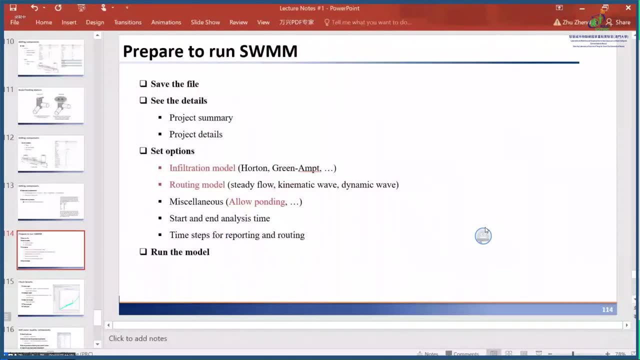 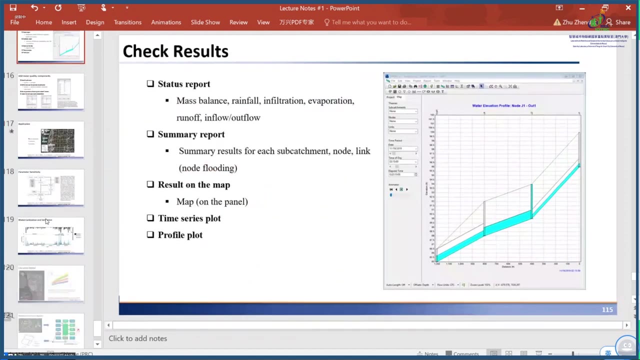 For the peak events there is a relatively larger difference. But again, those comparisons are pretty good. So that is simple. OK, So that's all like the tutorial for SWIM, And also I showed you just one application that you can do. 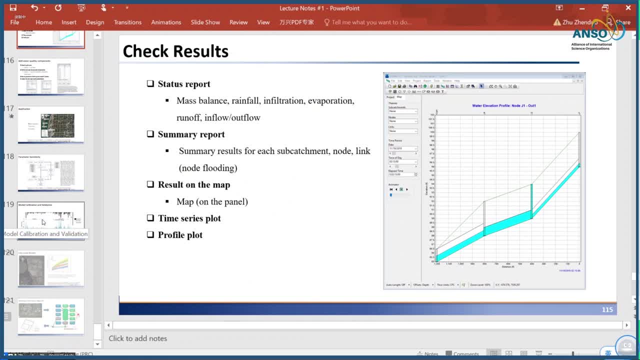 So there are other works we did for analyze the climate change effects, also analyzing how to manage the system in order to mitigate combined sewer overflows, and so on. So So tomorrow I will talk a little bit more about the second part. 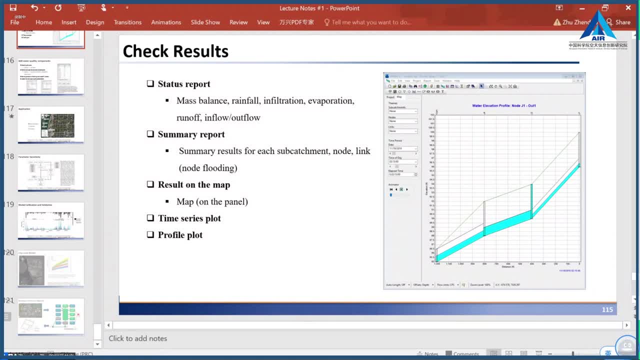 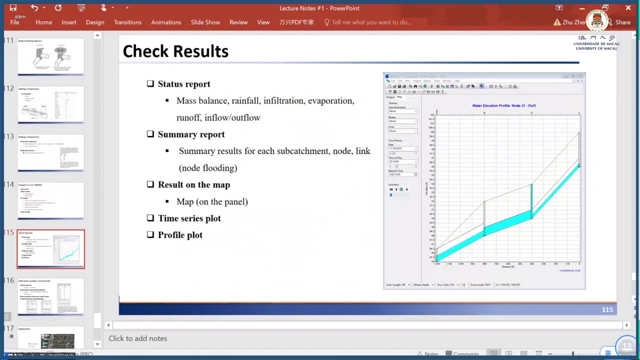 I think that's pretty much it for today. So let me see I think I may have some time to. I think I may have some time to answer questions. I will start with the last one, from Amit Kumar. What was the meaning of green line in this model? 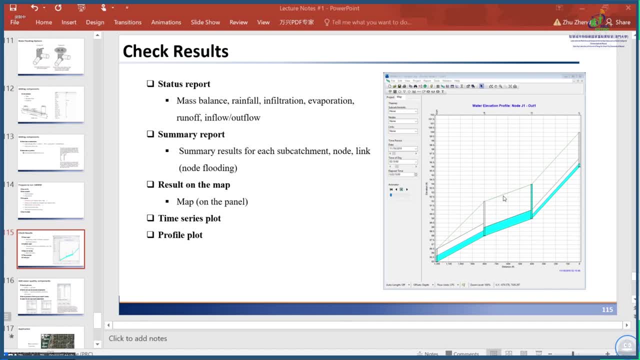 Wasn't sure what you mean by the green line. Are you talking about this line? Yes, or maybe not This line? OK, So this is a gradient line, But in this case it's simply just the elevation, the connecting of the elevation of the junctions. 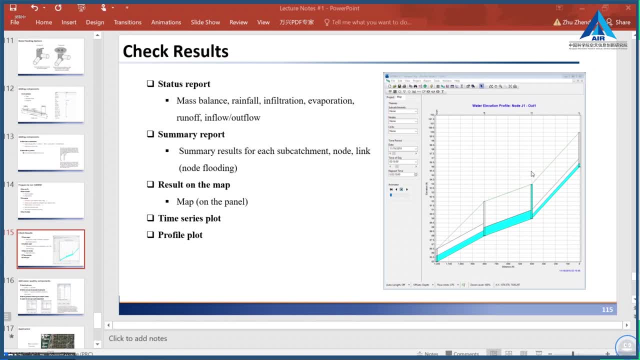 However, if the junction get pounding water or overflowing or something like that, then it's going to be a gradient line, But in the case of the overland flow, this might be different. OK, So let me see There are some follow up questions by Shukard Alisha.